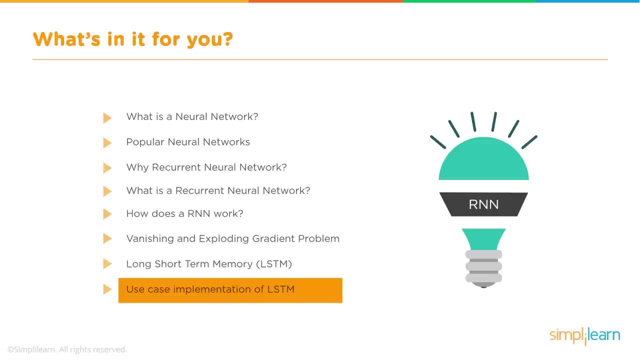 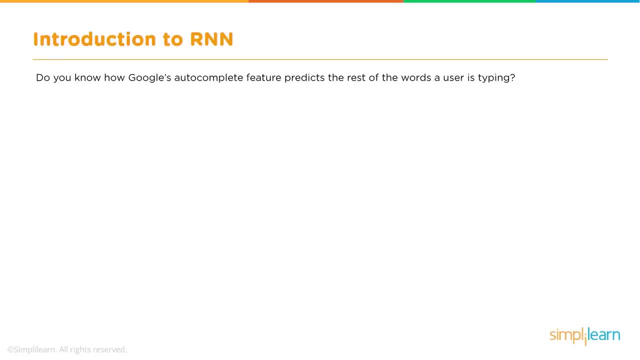 Before we dive into any of this, we're going to take a look at what is an RNN or an introduction to the RNN. Do you know how Google's autocomplete feature predicts the rest of the words a user is typing? I love that autocomplete feature as I'm typing away. It saves me a lot of time. 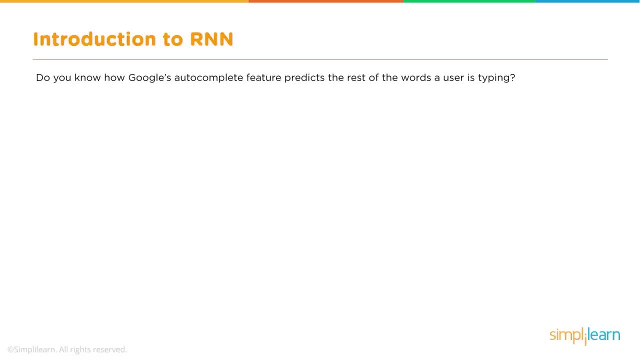 I can just kind of hit the enter key. It auto-fills everything and I don't have to type as much. First is a collection of large volumes of most frequently occurring consecutive words. This is fed into a recurrent neural network, analyses the data by finding the sequence of words occurring frequently and builds a model to predict the next word in the sentence. 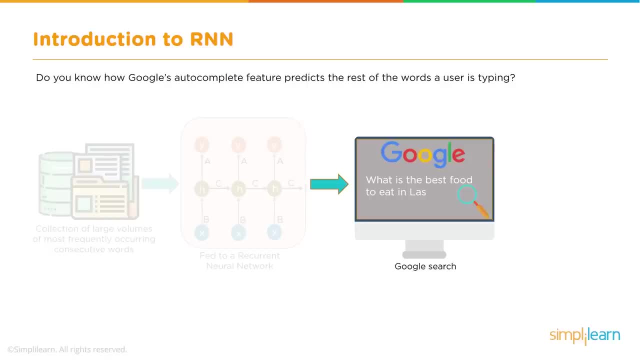 Then Google: what is the best food to eat in Las? I'm guessing you're going to say Las Mexico. No, it's going to be Las Vegas. The Google search will take a look at that and say, hey, The most common autocomplete is going to be Vegas in there and usually it gives you three or four different choices. 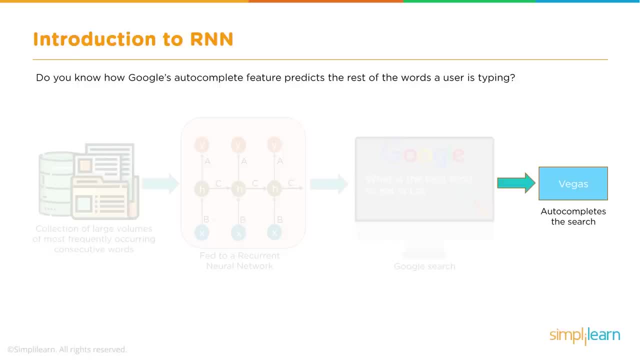 So it's a very powerful tool. It saves us a lot of time, especially when we're doing a Google search or even in Microsoft words has a. Some people get very mad at it because it auto-fills with the wrong stuff, But you know you're typing away and it helps you auto-fill. 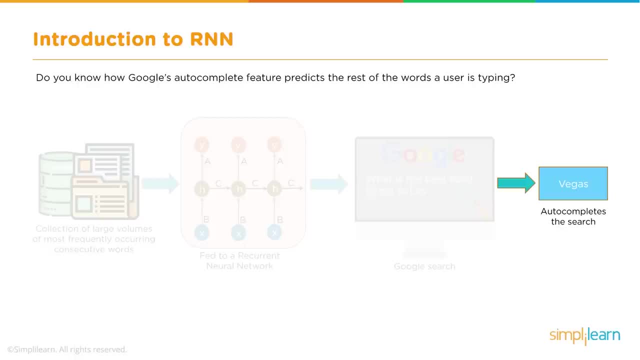 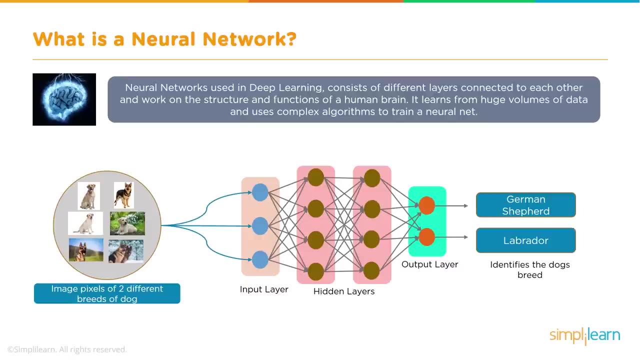 I have that in a lot of my different packages. It's just a standard feature that we're all used to now. So before we dive into the RNN and getting into the depths, let's go ahead and talk about what is a neural network. 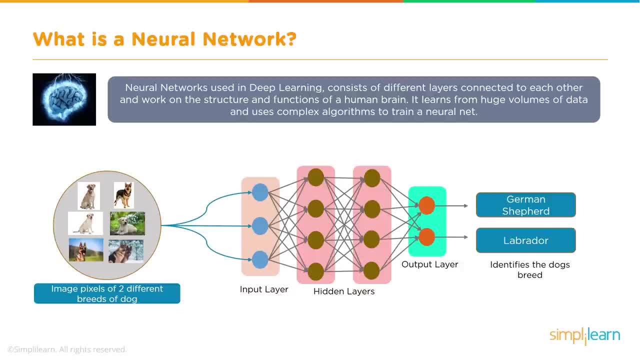 Neural network. Neural networks used in deep learning consist of different layers connected to each other and work on the structure and functions of a human brain. You're going to see that thread human in human brain and human thinking throughout deep learning. The only way we can evaluate an artificial intelligence or anything like that is to compare it to human function. 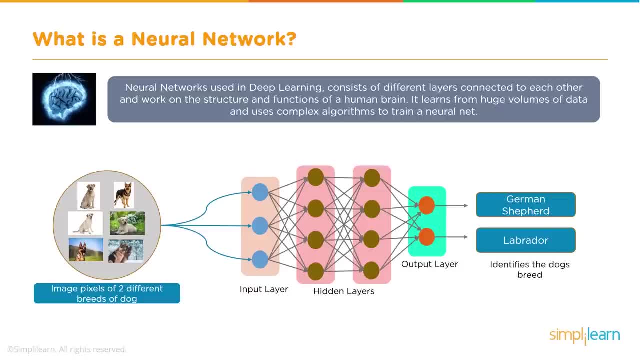 Very important note on there- And it learns from huge volumes of data and it uses complex algorithm to train a neural net. So in here we have image pixels of two different Breeds of dog. One looks like a nice floppy-eared lab and one a German shepherd. 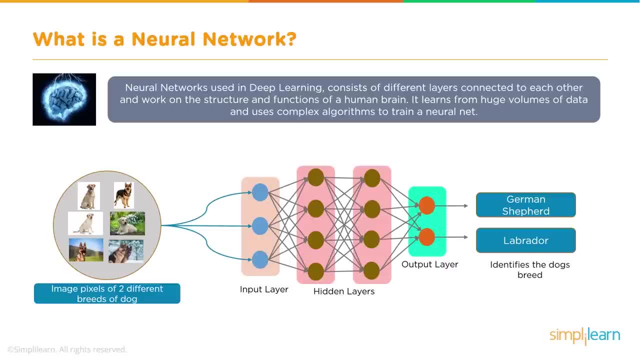 You know both wonderful breeds of animals. That image then goes into an input layer. That input layer might be formatted at some point because you have to let it know. like you know, different pictures are going to be different sizes and different color content. 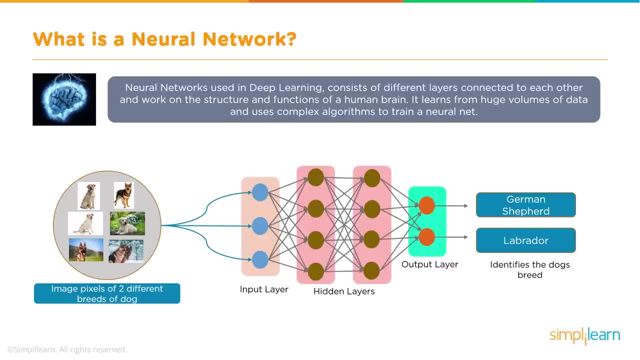 Then it'll feed into hidden layers. So each of those pixels or each point of data goes in and then splits into the hidden layer, which then goes into another hidden layer, which then goes to an output layer, RNN. there's some changes in there which we're going to get into. 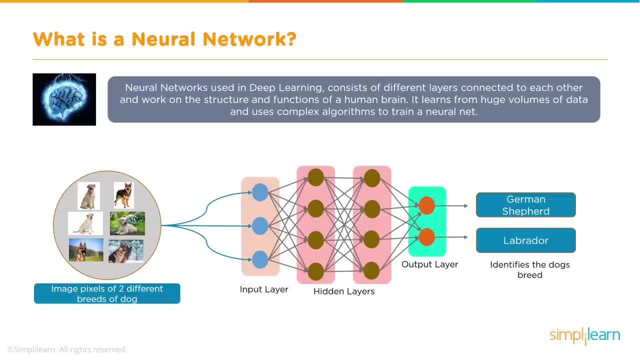 So it's not just a straightforward propagation of data, like we've covered in many other tutorials. And finally, you have an output layer, and the output layer has two outputs. It has one that lights up if it's a German Shepherd and another that lights up if it's a Labrador. 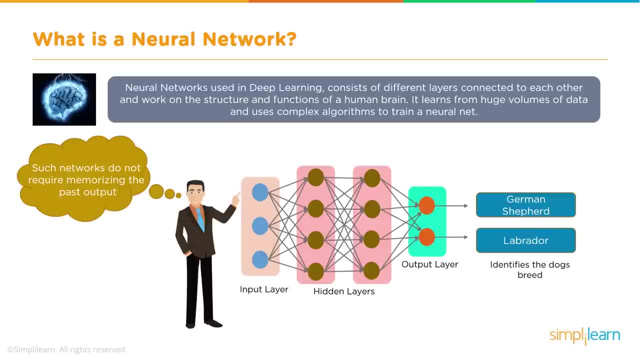 So it identifies the dog's breed. Set networks do not require memorizing the past output. So our forward propagation is just that It goes forward and doesn't have to re-memorize stuff. And you can see there, That's not actually me in the picture. 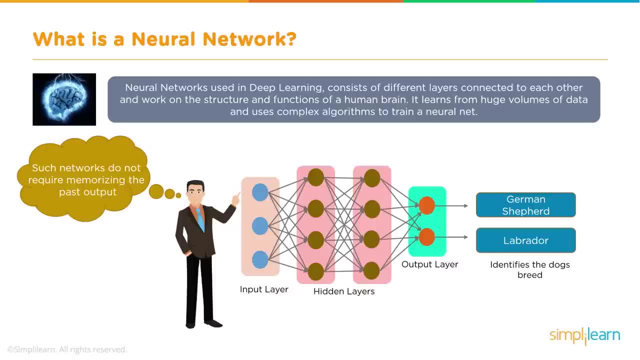 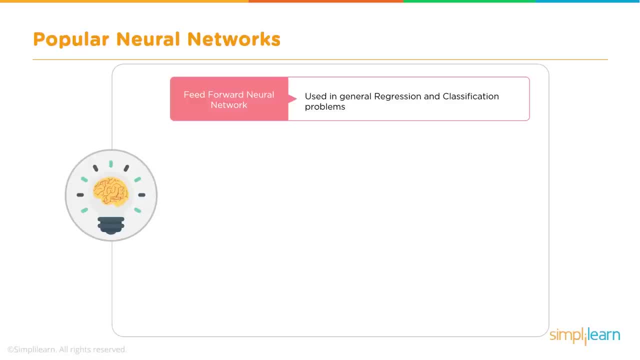 Dressed up in my suit. I haven't worn a suit in years, So as we're looking at this, we're going to change it up a little bit. Before we cover that, let's talk about popular neural networks. First, there's the feed-forward neural network, used in general regression and classification problems. 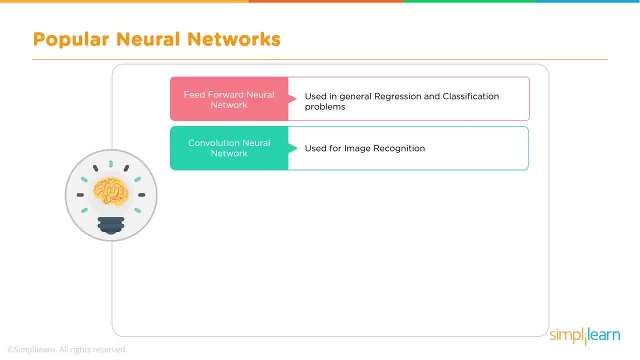 And we have the convolution neural network, used for image recognition, Deep neural network used for acoustic modeling, Deep belief network used for cancer detection, And recurrent neural network used for speech recognition. Now, taken a lot of these and mixed them around a little bit. 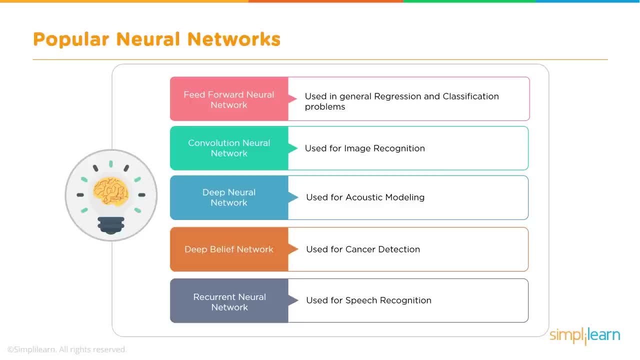 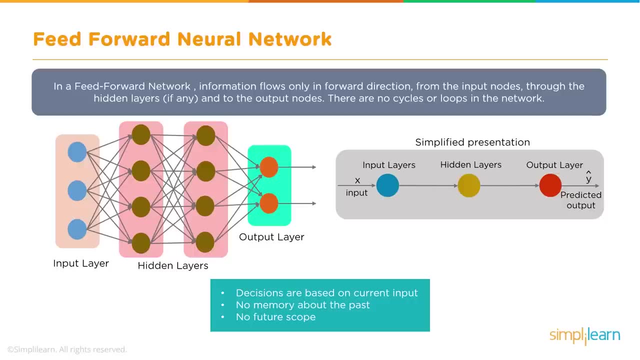 So just because it's used for one thing doesn't mean it can't be used for other modeling. But generally, this is where the field is And this is how those models are generally being used right now. So we talk about a feed-forward neural network. 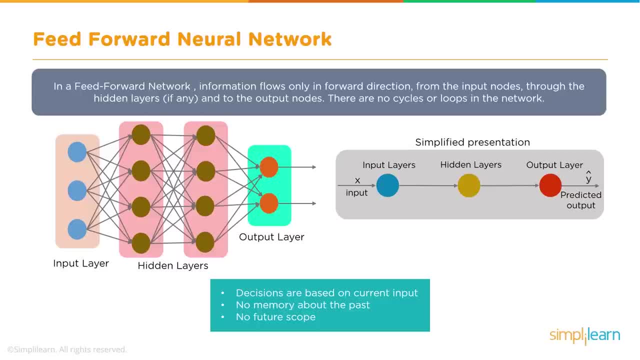 In a feed-forward neural network, information flows only in the forward direction, From the input nodes through the hidden layers, if any, and to the output nodes. There are no cycles or loops in the network, And so you can see, here we have our input layer. 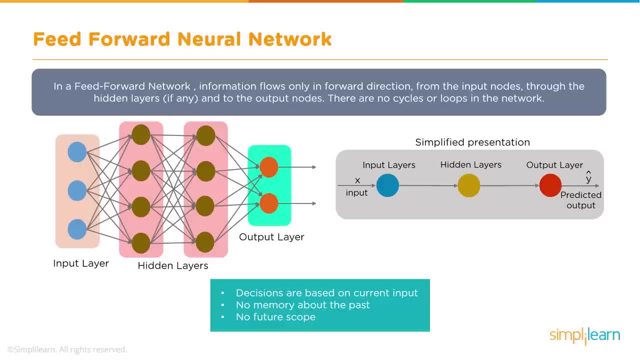 I was talking about how it just goes straight forward Into the hidden layers, So each one of those connects And then connects to the next hidden layer. It connects to the output layer And of course we have a nice simplified version where it has a predicted output. 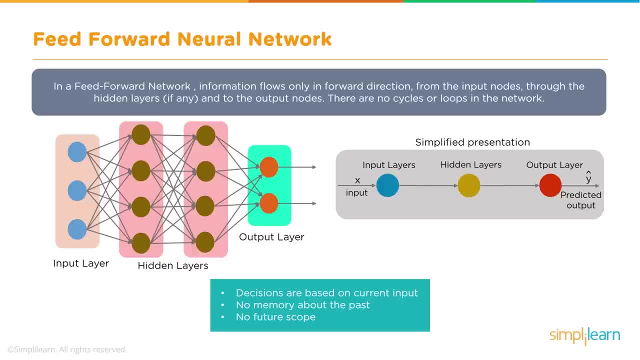 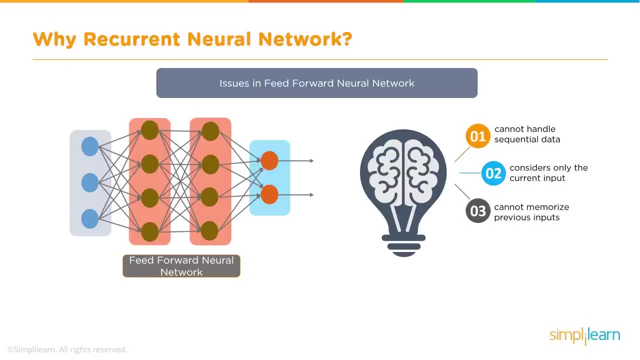 And they refer to the input as X a lot of times, And the output as Y. Decisions are based on current input, No memory about the past, No future scope. Why recurrent neural network Issues in feed-forward neural network? So one of the biggest issues is because it doesn't have a scope of memory or time. 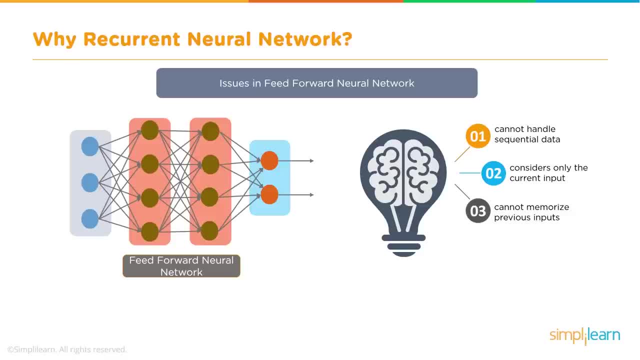 A feed-forward neural network doesn't know how to handle sequential data. It only considers only the current input. So if you have a series of things, and because three points back affects what's happening now And what's your output, affects what's happening. 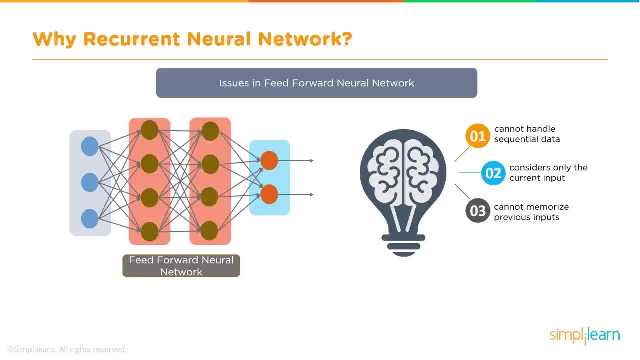 That's very important. So whatever I put as an output is going to affect the next one. A feed-forward doesn't look at any of that. It just looks at this is what's coming in And it cannot memorize previous inputs. So it doesn't have that list of inputs coming in. 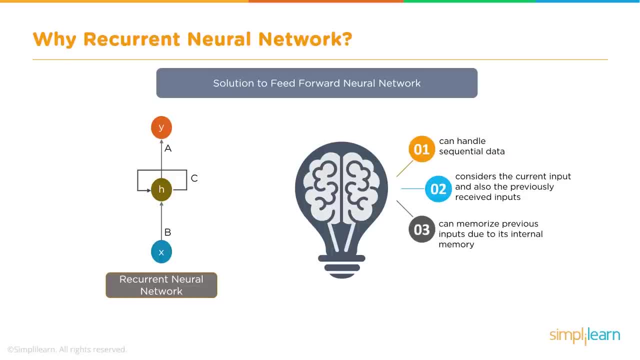 Solution to feed-forward neural network. You'll see here where it says recurrent neural network And we have our X on the bottom, Going to H, Going to Y. That's your feed-forward, But right in the middle it has a value C. 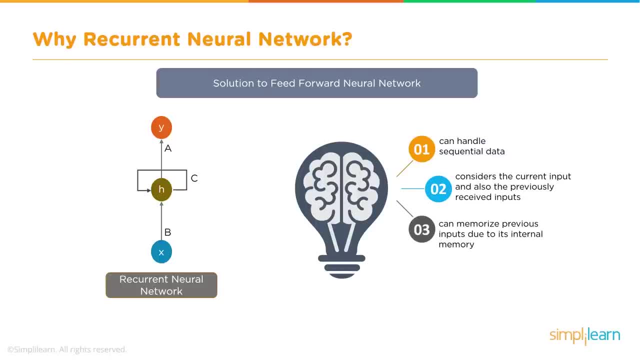 So it's a whole other process. So it's memorizing what's going on in the hidden layers, And the hidden layers, as they produce data, feed into the next one. So your hidden layer might have an output that goes off to Y, But that output goes back into the next prediction coming in. 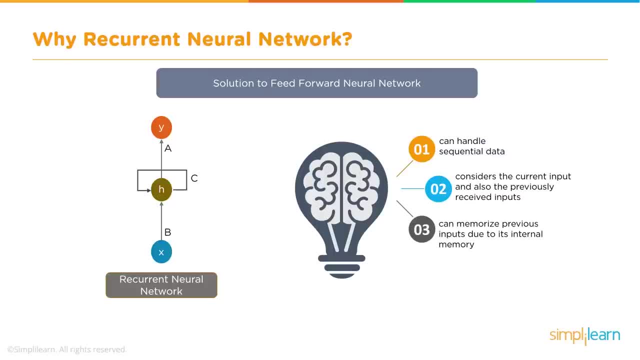 What this does is. this allows it to handle sequential data. It considers the current input and also the previously received inputs, And if we're going to look at general drawings And solutions, We should also look at applications of the RNN. Image captioning. 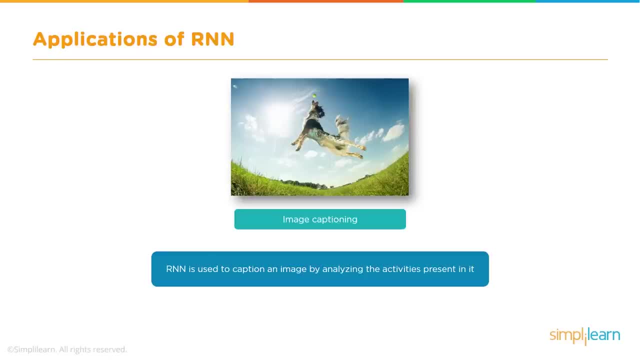 RNN is used to caption an image by analyzing the activities present in it. A dog catching a ball in midair. That's very tough. I mean, we have a lot of stuff that analyzes images of a dog And the image of a ball. 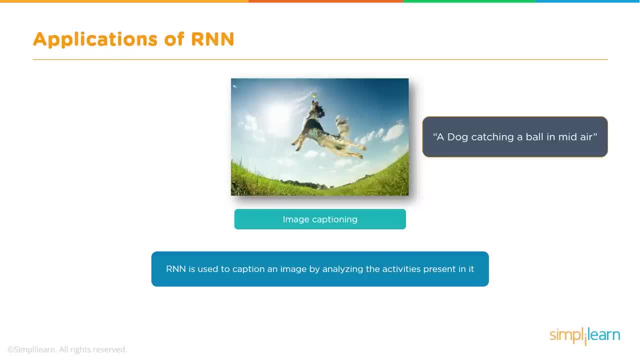 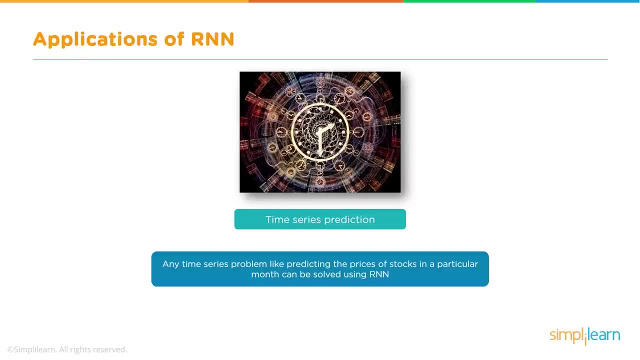 But it's able to add one more feature in there. that's actually catching the ball in midair: Time series prediction. Any time series problem, like predicting the prices of stocks in a particular month, can be solved Using RNN, And we'll dive into that in our use case. 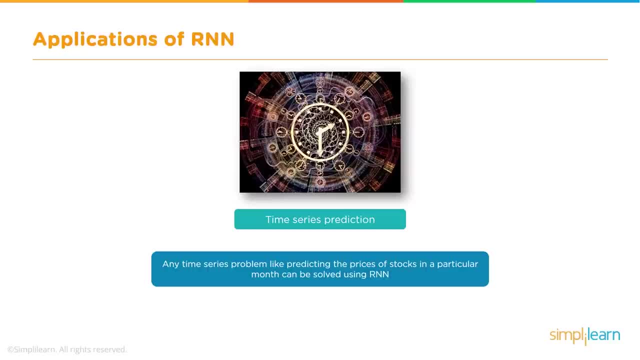 And actually take a look at some stock. One of the things you should know about analyzing stock today Is that it is very difficult And if you're analyzing the whole stock, The stock market at the New York Stock Exchange in the US- 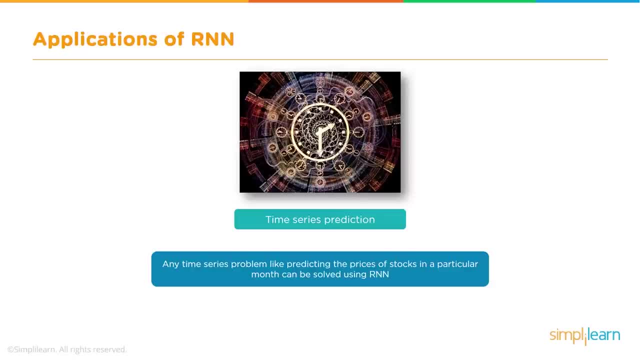 Produces somewhere in the neighborhood. If you count all the individual trades And fluctuations by the second, It's like three terabytes a day of data. So we're only going to look at one stock. Just analyzing one stock is really tricky. 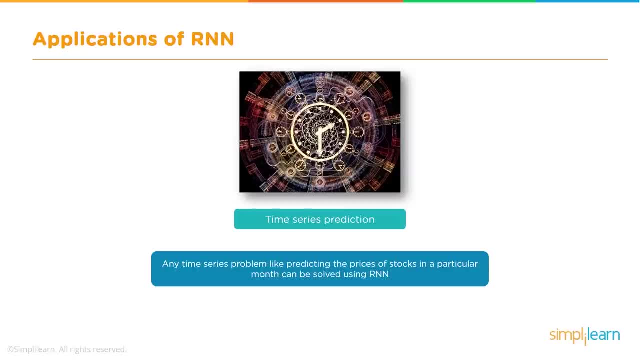 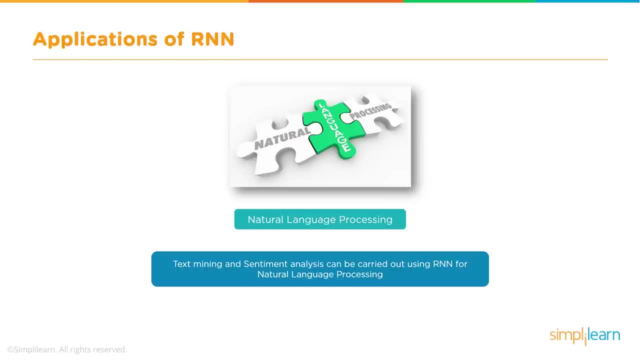 And here we'll give you a little jump on that. So that's exciting, But don't expect to get rich off of it immediately. Another application of the RNN is natural language processing. Text mining and sentiment analysis can be carried out using RNN for natural language processing. 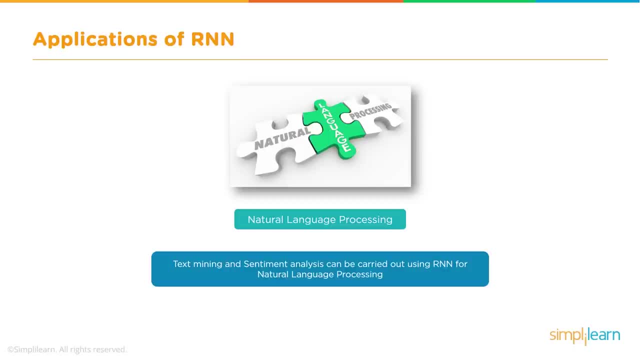 And you can see right here The term natural language processing, When you stream those three words together, Is very different than if I said processing language naturally. So the time series is very important when we're analyzing sentiments. It can change the whole value of a sentence. 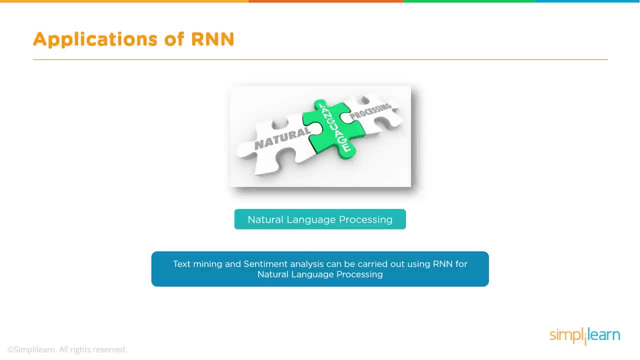 Just by switching the words around, Or if you're just counting the words, You might get one sentiment Where, if you actually look at the order they're in, You get a completely different sentiment. When it rains, Look for rainbows. When it's dark, 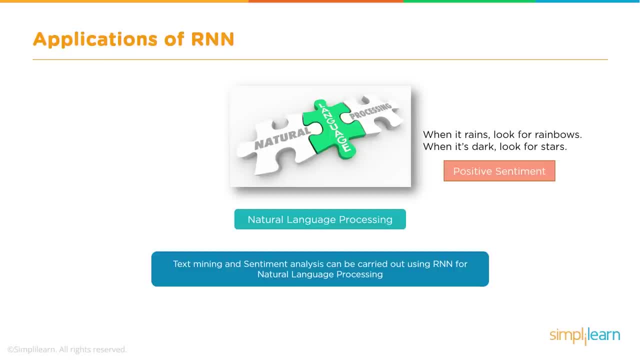 Look for stars. Both of these are positive sentiments And they're based upon the order of which the sentence is going in Machine translation Given an input in one language, RNN can be used to translate the input into different languages as output. 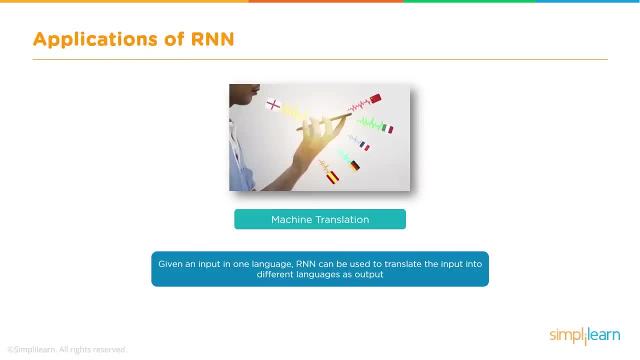 I myself am very linguistically challenged. But if you study languages And you're good with languages- You know right away That if you're speaking English, You would say big cat, And if you're speaking Spanish You would say cat big. 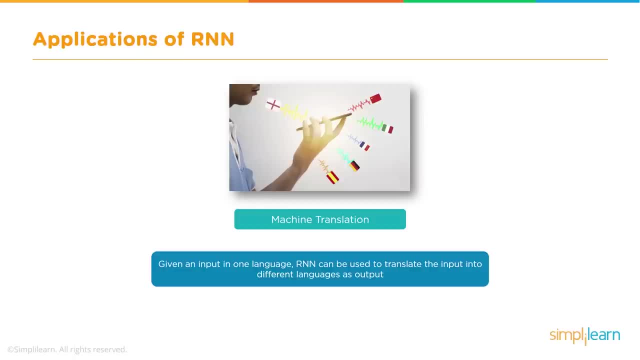 So that translation is really important To get the right order To get. There's all kinds of parts of speech That are important to know By the order of the words. Here this person is speaking in English And getting translated And you can see here. 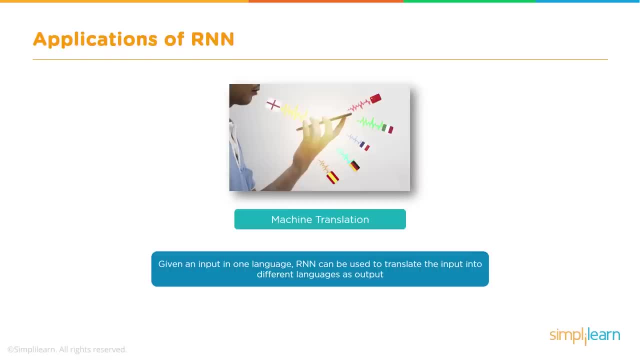 A person is speaking in English In this little diagram. I guess that's denoted by the flags. I have a flag. I own it, No, But there's probably a person in the room. That's a person. That's a person. 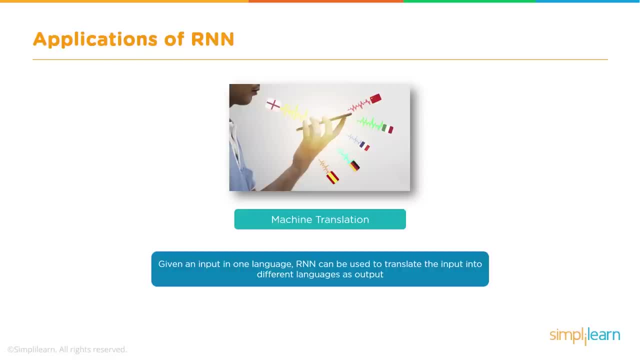 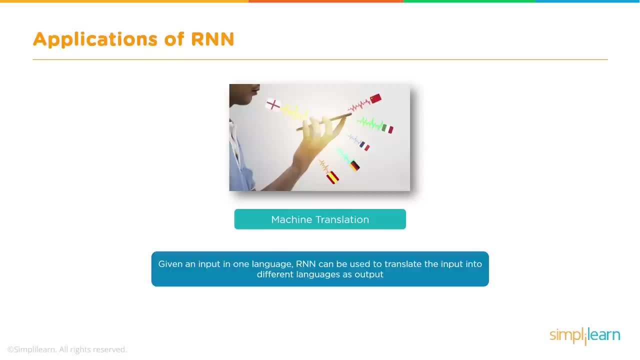 German And Spanish languages. Some of the tools coming out Are just so cool. So somebody like myself, Who's very linguistically challenged, I can now travel into worlds I would never think of Because I can have something Translate my English. 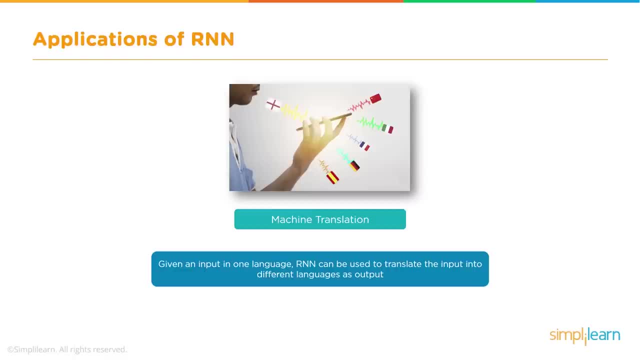 Back and forth Readily And I'm not stuck With a communication gap, So let's dive in To. what is a recurrent neural network. Recurrent neural networks Is a recurrent neural network. Is a recurrent neural network. Is a recurrent neural network. 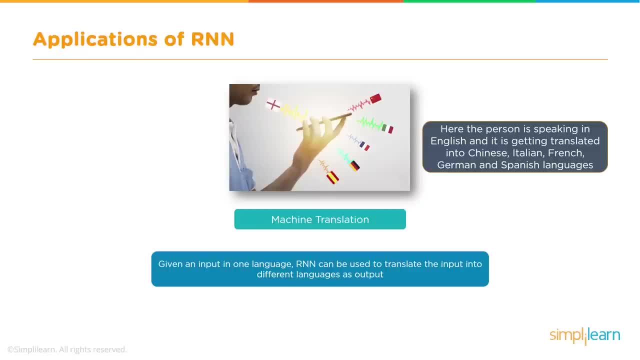 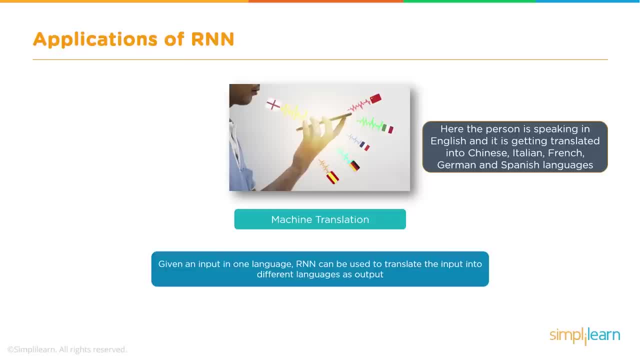 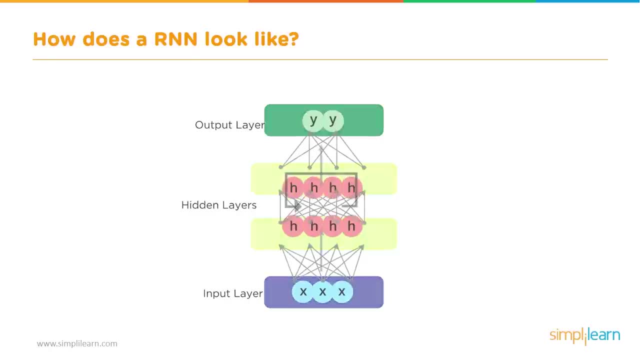 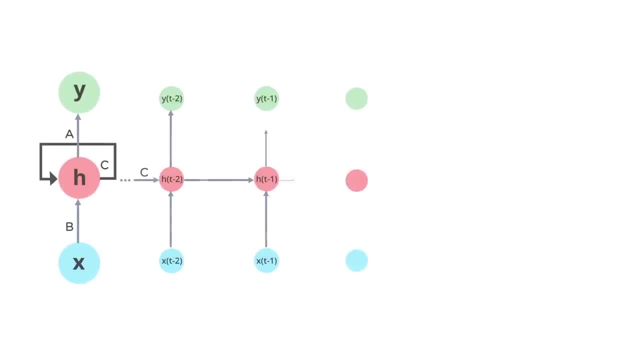 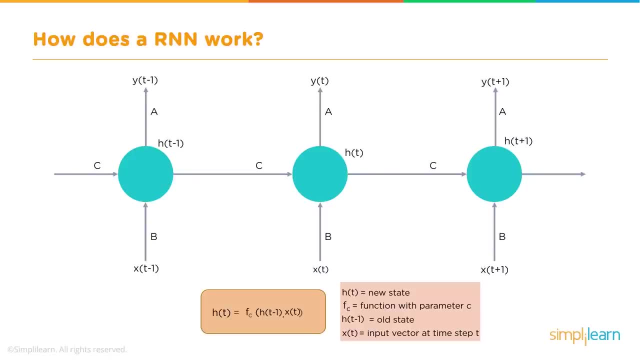 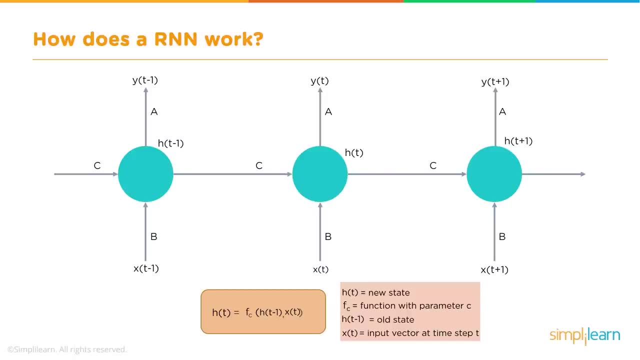 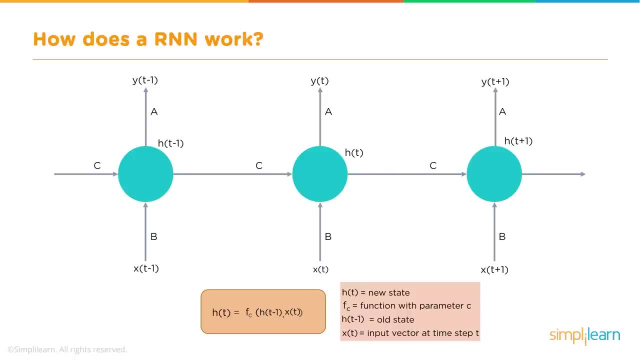 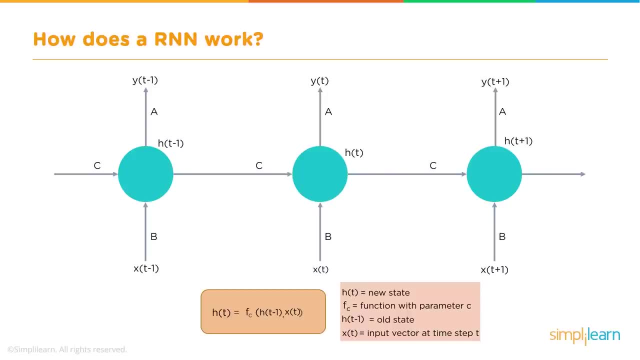 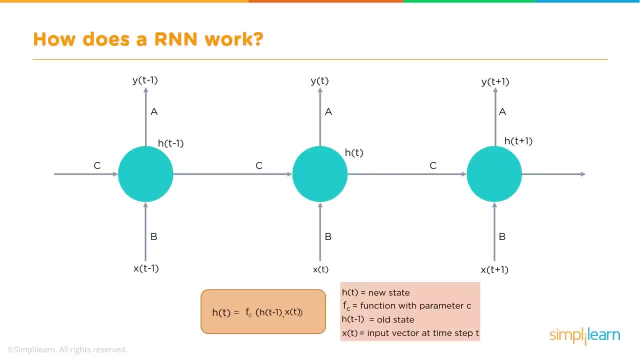 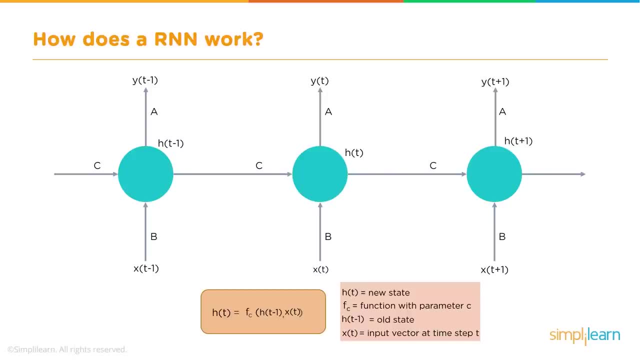 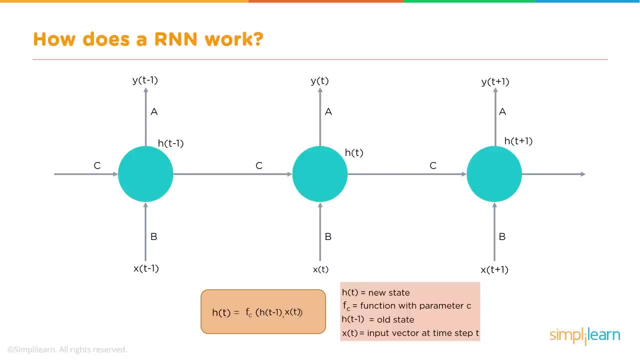 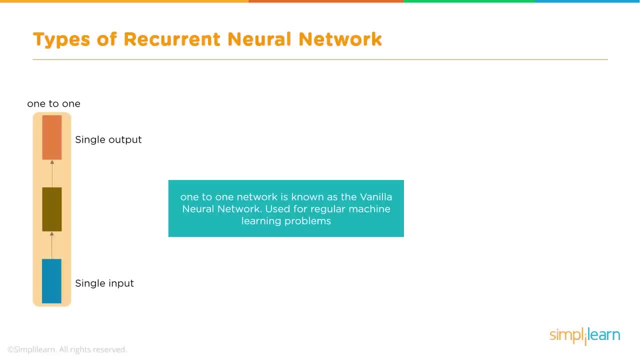 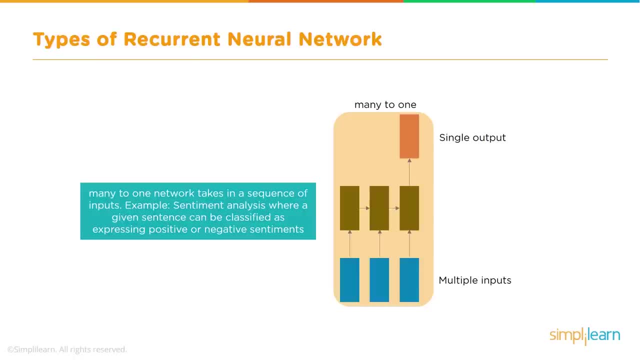 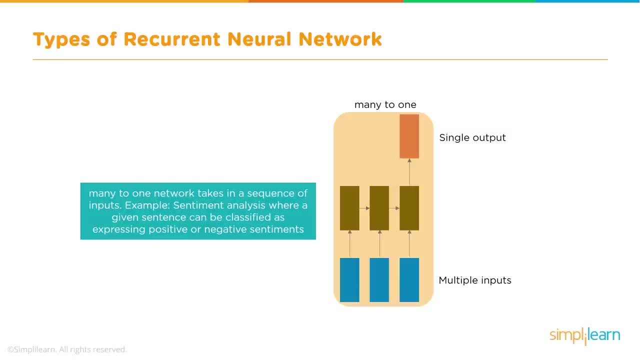 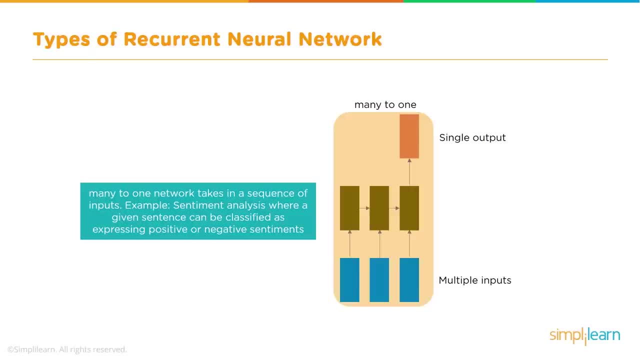 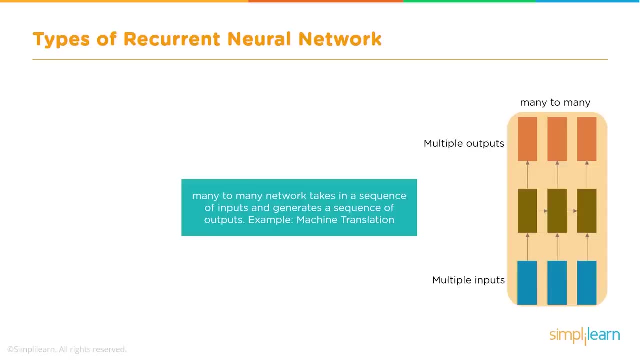 this case, image captioning, as we looked at earlier, where we have not just looking at it as a dog, but a dog catching a ball in the air. And then you have many-to-one network. takes in a sequence of inputs. Examples: sentiment analysis, where a given sentence can be classified as 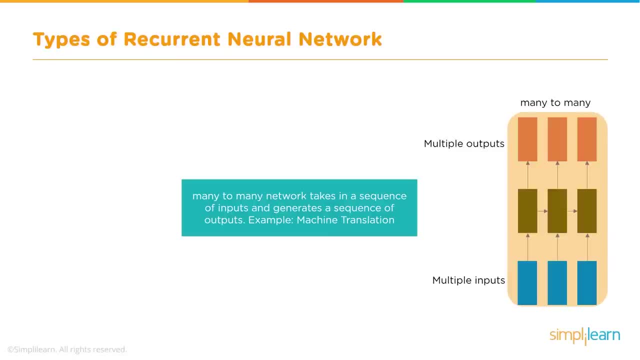 expressing positive or negative sentiments And we looked at that as we were discussing: if it rains, look for a rainbow. So positive sentiment where rain might be a negative sentiment. if you're just adding up the words in there And then the course, if you're going to do, 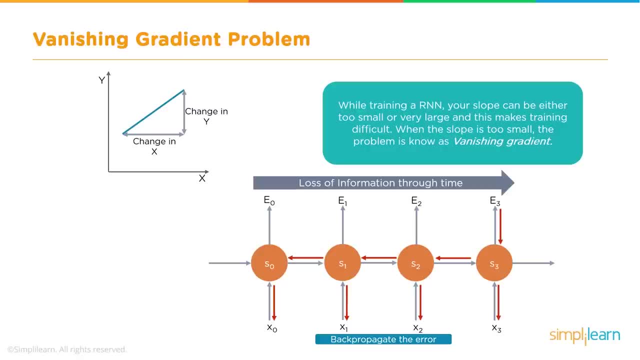 a one-to-one, many-to-one, one-to-many- there's many-to-many networks- takes in a sequence of inputs and generates a sequence of outputs. Example: machine translation. So we have a lengthy sentence coming in in English and then going out in all the different languages. You know just a. 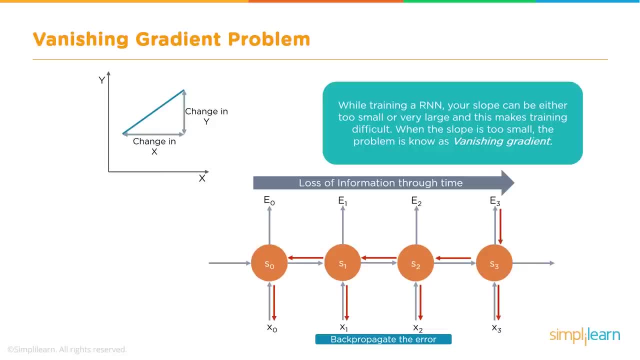 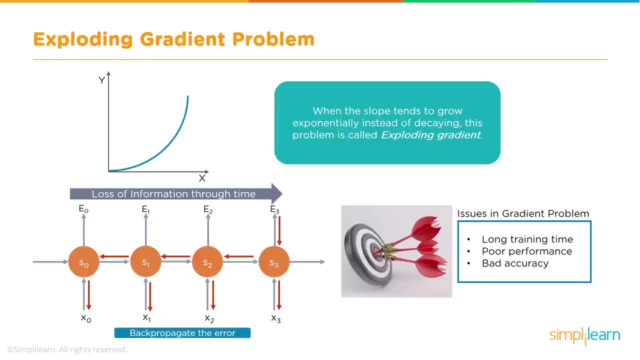 wonderful tool, Very complicated. It's a complicated set of computations. You know, if you're a translator, you realize just how difficult it is to translate into different languages. One of the biggest things you need to understand when we're working with this neural network is what's called the vanishing gradient. 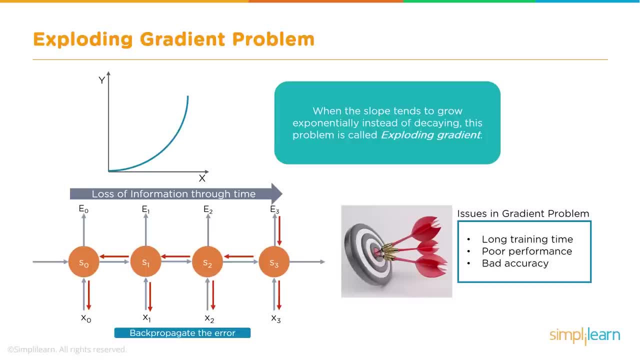 problem While training an RNN. your slope can be either too small or very large, And this makes training difficult. When the slope is too small, the problem is known as vanishing gradient And you'll see here they have a nice image: loss of information through time. So if you're 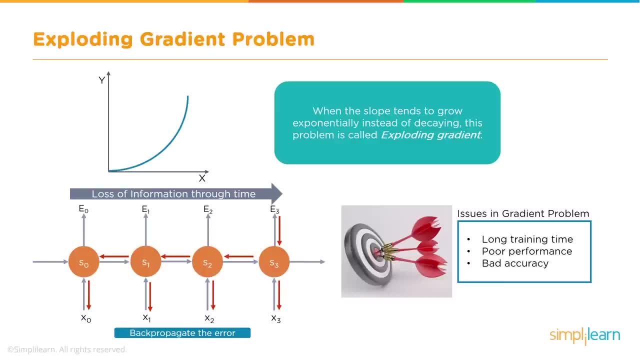 pushing not enough information forward, that information is lost. And then when you go to train it, you start losing the third word in the sentence, or something like that, or it doesn't quite follow the full logic of what you're working on. Exploding gradient problem: Oh, this is one that runs into. 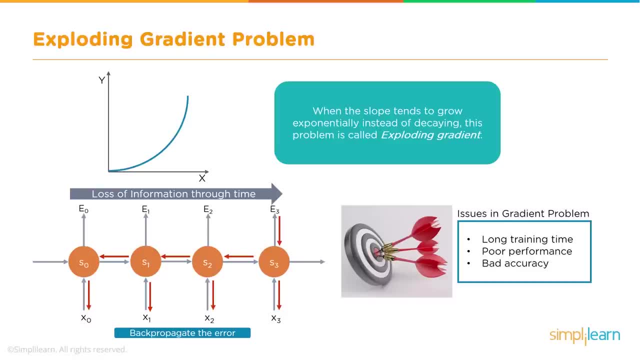 everybody When you're working with this particular neural network, when the slope tends to grow exponentially instead of decaying. this problem is called exploding gradient Issues in gradient problem: long tracking time, poor performance, bad accuracy. And I'll add one more in there: Your computer, if you're on a lower end computer testing out a. 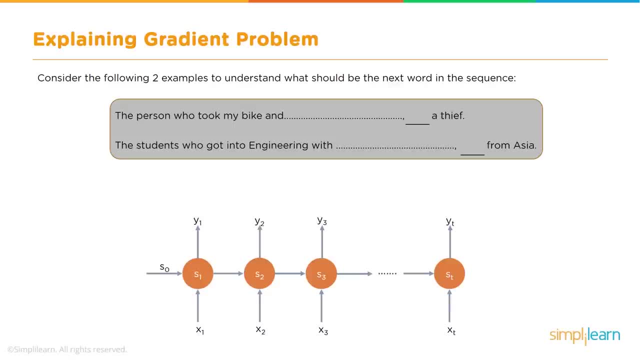 model will lock up and give you the memory error: Exploding gradient problem. Consider the following two examples to understand what should be the next word in the sequence: The person who took my bike and blank a thief, The students who got into engineering with blank from Asia, And you can see. 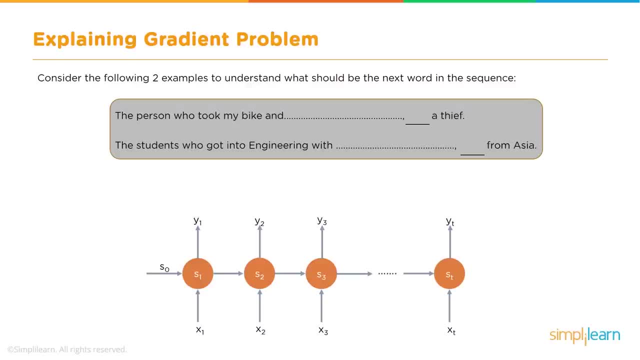 in here. we have our X value going in, We have the previous value going forward, And then you back, propagate the error like you do with anything, And then you have the next word in the sequence: Any neural network. And as we're looking for that missing word, maybe we'll have. the person took my 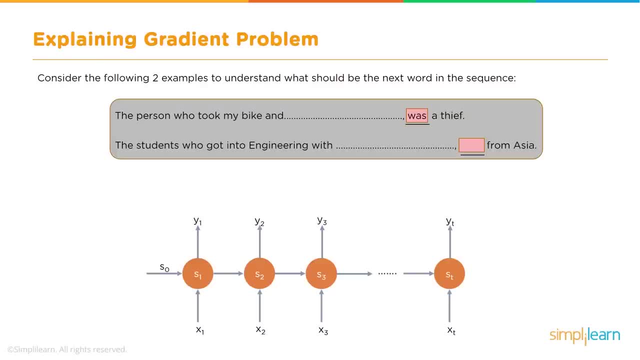 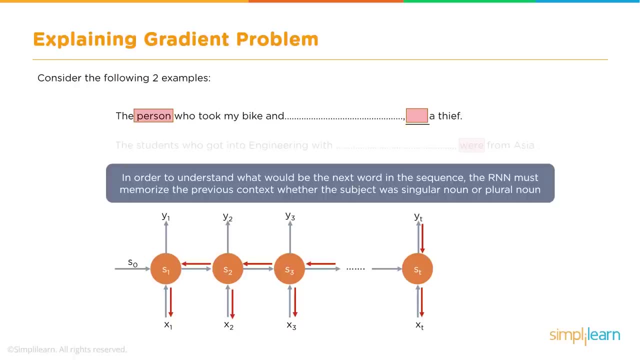 bike and blank was a thief, And the student who got into engineering with a blank were from Asia. Consider the following example: The person who took the bike- So we'll go back to the person who took the bike- was, blank, a thief, In order to understand what would be the next word in the. 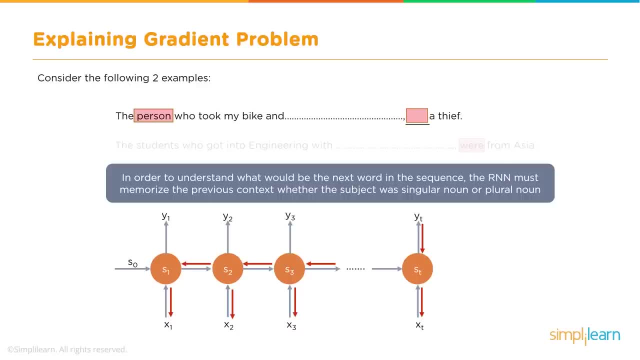 sequence. the RNN must memorize the previous context, whether the subject was singular noun or a plural noun. So was a thief is singular The student who got into engineering with a blank. the RNN must memorize the previous context, whether the subject was singular noun or a plural noun. 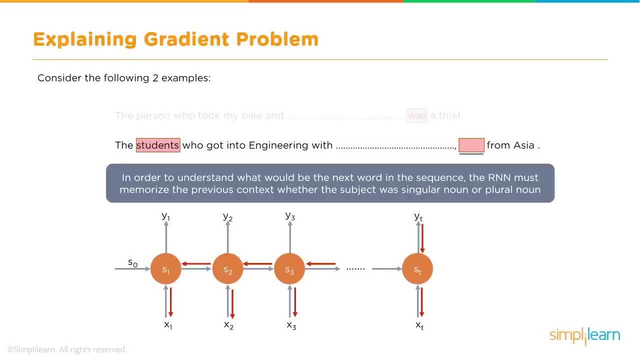 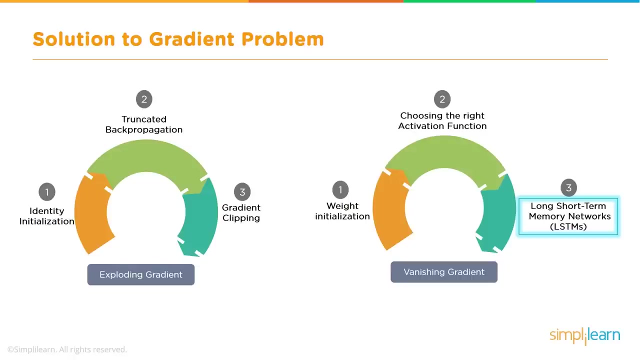 And so you can see here, the students who got into engineering with blank were from Asia. It might be sometimes difficult for the error to back propagate to the beginning of the sequence, to predict what should be the output. So when you run into the gradient problem, we need a solution. The solution: to the gradient problem. First, we are going to look at exploding gradient where we are going to're going to look at exploding gradient Where we are going to run into the gradient problem. We're going to run in the gradient problem ind we need a solution, The solution to the gradient problem. First we're going to look. 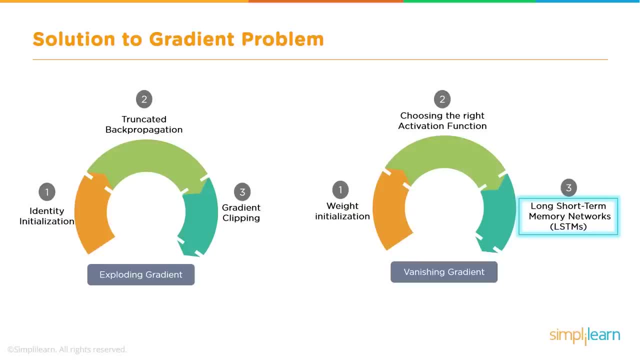 We have three different solutions, depending on what's going on. One is identity initialization. So the first thing we want to do is see if we can find a way to minimize the identities coming in instead of having it identify everything- just the important information we're looking at. 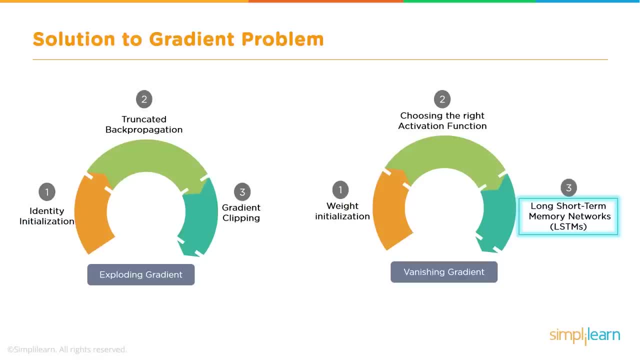 Next is to truncate the back propagation. So instead of having whatever information it's sending to the next series, we can truncate what it's sending. We can lower that particular set of layers, make those smaller. And finally, is a gradient clipping, So when we're training it, we can clip what that gradient looks like. 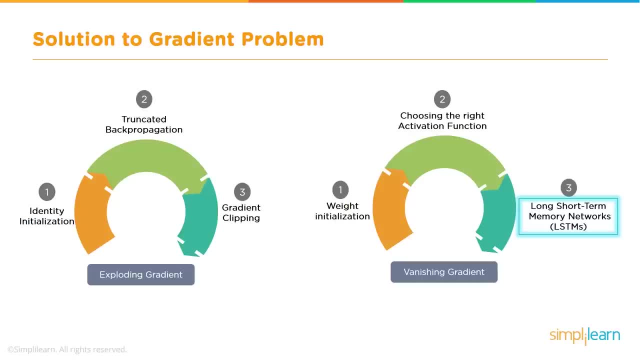 and narrow the training model that we're using. When you have a vanishing gradient- the option problem- we can take a look at weight initialization: very similar to the identity, but we're going to add more weights in there so it can identify different aspects of what's coming in better. 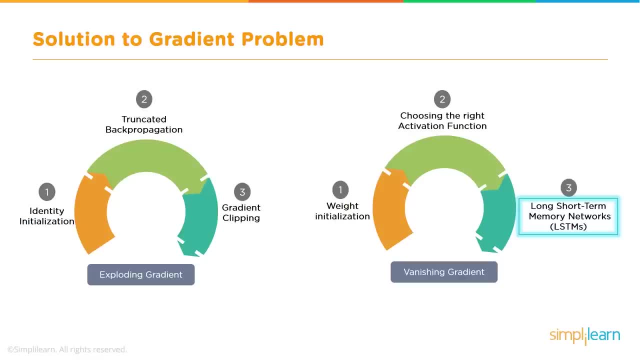 Choosing the right activation function. that's huge. So we might be activating based on one thing and we need to limit that. We haven't talked too much about activation functions, so we'll look at that just minimally. There's a lot of choices out there. 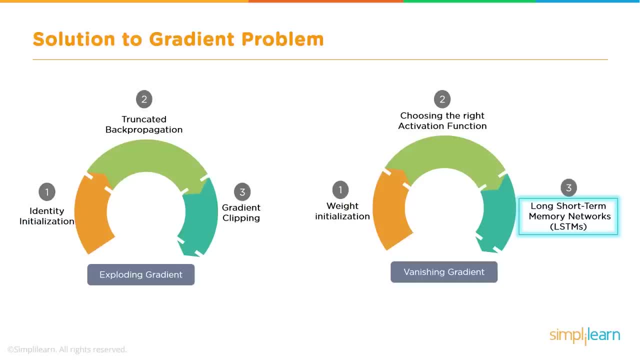 And then finally, there's long short-term memory networks, the LSTMS. We can make adjustments to that. So just like we can clip the gradient as it comes out, we can also expand on that. We can increase the memory network, the size of it so it handles more information. 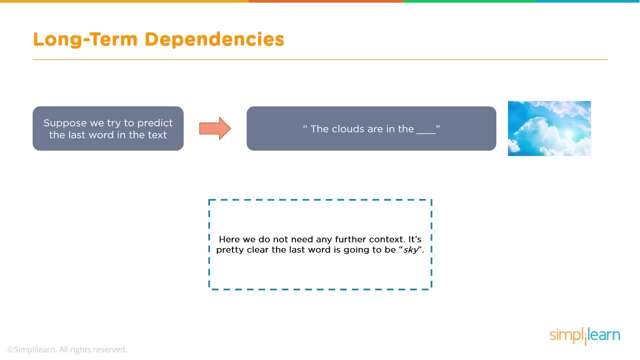 And one of the most common problems in today's setup is what they call long-term dependencies. Suppose we try to predict the last word in the text: The clouds are in the- and you probably said sky Here. we do not need any further context. 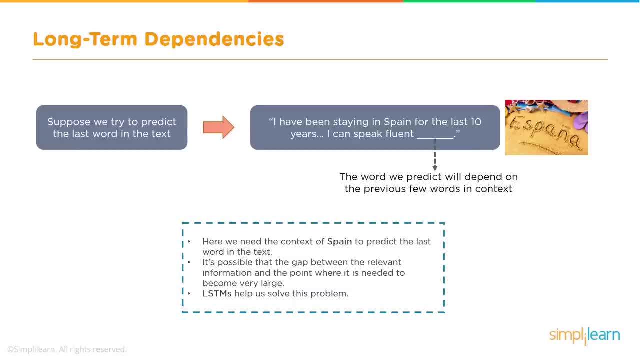 It's pretty clear that the last word is going to be sky. Suppose we try to predict the last word in the text. I have been staying in Spain for the last 10 years. I can speak fluent. Maybe you said Portuguese or French. 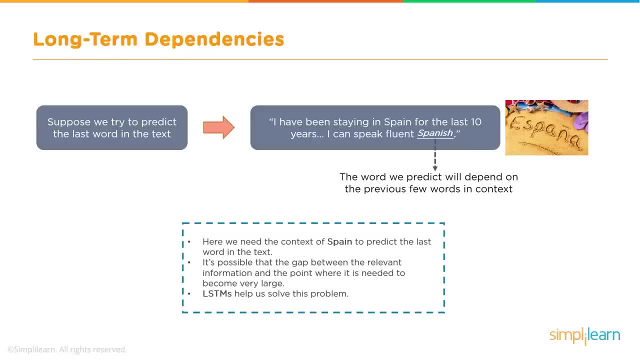 No, you probably said Spanish. The word we predict will depend on the previous few words in context. Here we need the context of Spain to predict the last word in the text. It's possible that the gap between the relevant information and the point where it is 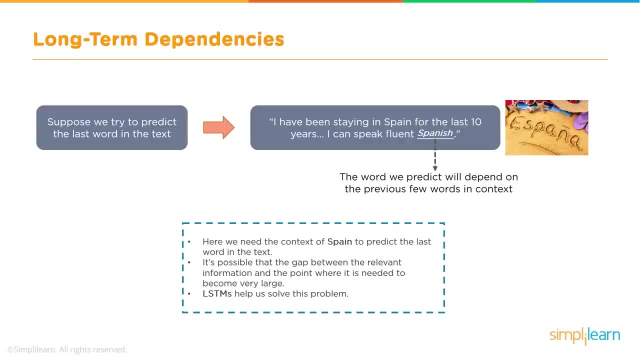 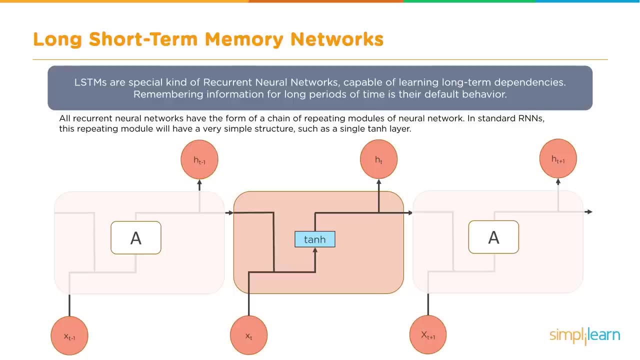 needed to become very large. LSTMs help us solve this problem. So the LSTMs are a special kind of recurrent neural network capable of learning long-term dependencies. Remembering information for long periods of time is their default behavior. All recurrent neural networks have the form of a chain of repeating modules of neural network connections. 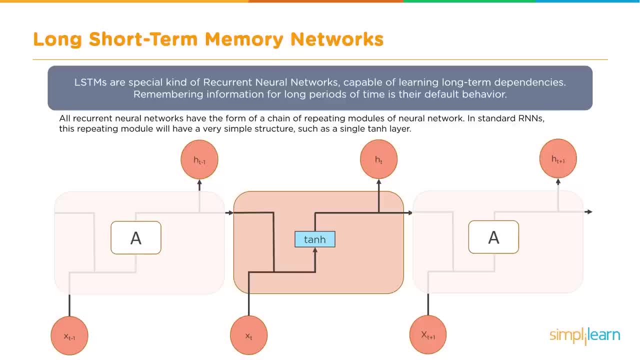 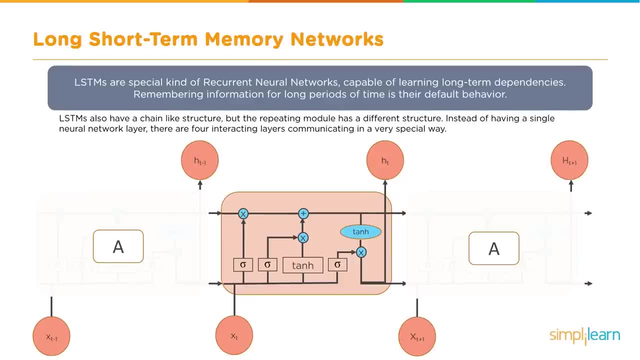 In standard RNNs. this repeating module will have a very simple structure, such as a single tangent H layer. LSTMSs also have a chain-like structure, but the repeating module has a different structure. Instead of having a single neural network layer, there are four interacting layers communicating in a very special way. 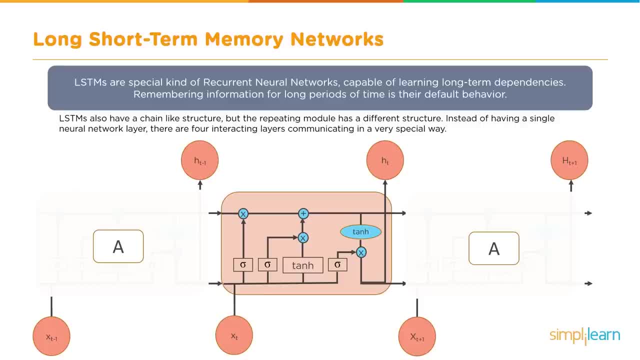 LSTMSs are a special kind of recurrent neural network capable of learning long-term dependencies. Remembering information for long periods of time is their default behavior. LSTMSs also have a chain-like structure, but the repeating module has a different structure. 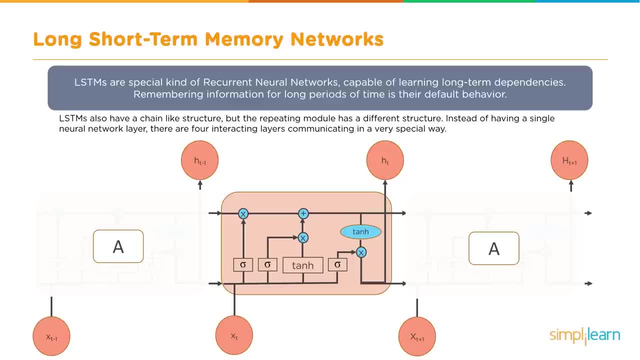 Instead of having a single neural network layer, there are four interacting layers communicating in a very special way. As you can see, the deeper we dig into this, the more complicated the graphs get In. here I want you to note that you have X of T minus 1 coming in. 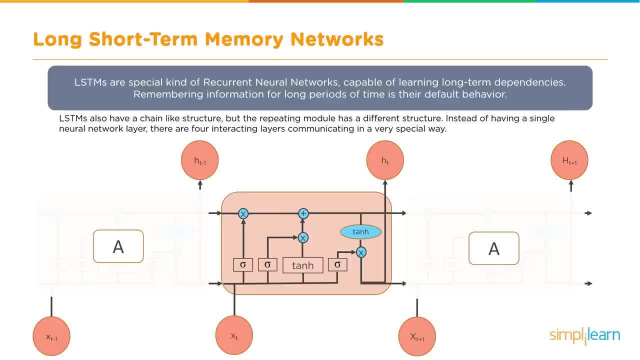 you have X of T coming in and you have X of T plus 1.. And you have H of T minus 1, and H of T coming in and H of T plus 1 going out, And of course, on the other side is the output A. 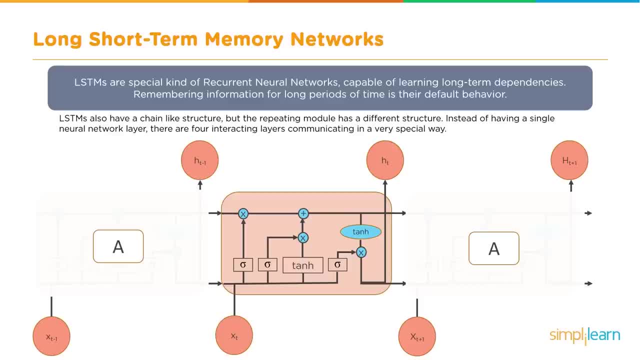 In the middle we have our tangent H, but it occurs in two different places. So not only when we're computing the X of T plus 1 are we getting the tangent H from X of T, but we're also getting that value coming in from the X of T minus 1.. 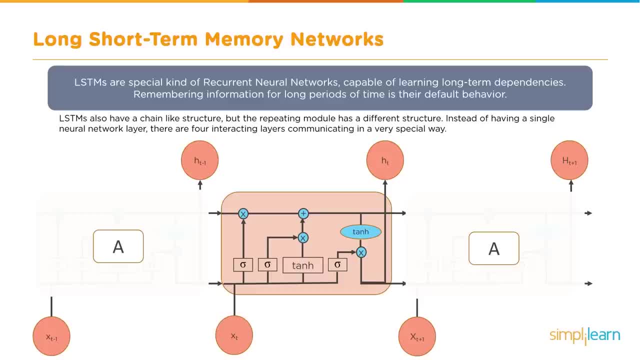 So the short of it is: as you look at these layers, not only does the propagate through the first layer, goes into the second layer, back into itself, but it's also going into the third layer. So now we're kind of stacking those up. 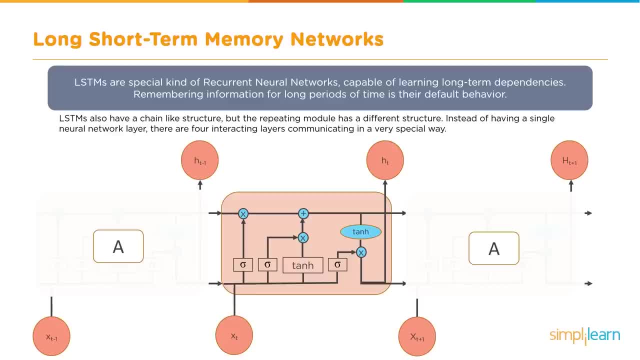 And this can get very complicated. as you grow that in size, It also grows in memory too and in the amount of resources it takes. But it's a very powerful tool to help us address the problem of complicated, long, sequential information coming in, like we were just looking at in the sentence. 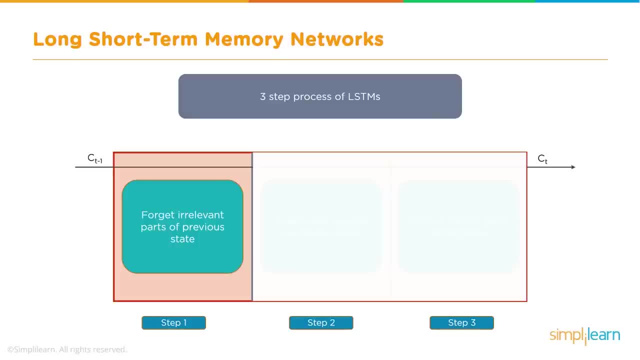 And when we're looking at our long, short-term memory network, there's three steps of processing in the LSTMS that we look at. The first one is we want to forget irrelevant parts of the previous state. You know a lot of times, like you know, is as in a 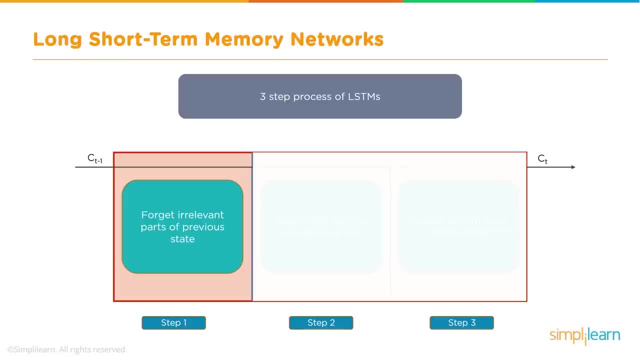 unless we're trying to look at whether it's a plural noun or not. they don't really play a huge part in the language, So we want to get rid of them. Then selectively update cell state values. So we only want to update the cell state values that reflect what we're working on. 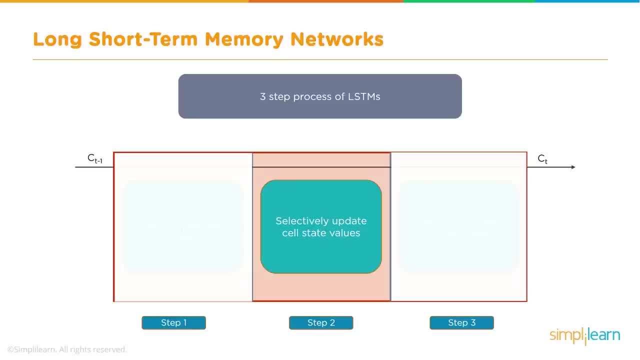 And finally, we want to put only output certain parts of the cell state. So, whatever's coming out, we want to limit what's going out too. And let's dig a little deeper into this. Let's just see what this really looks like. 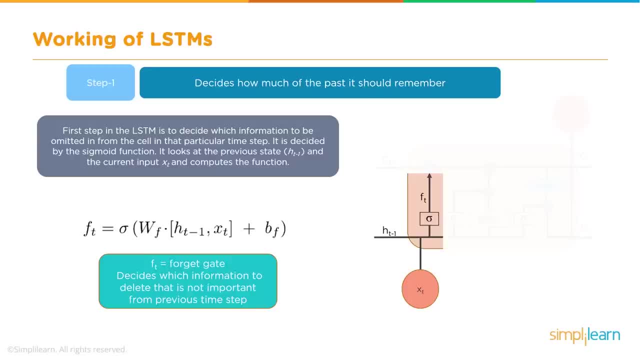 So step one decides how much of the past it should remember. First step in the LSTM is to decide which information to be omitted in from the cell in that particular time step. It is decided by the sigmoid function. It looks at the previous state h at t minus 1,. 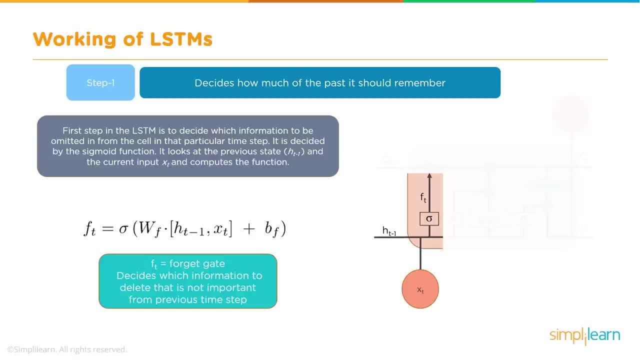 and the current input, x at t, and computes the function. So you can see over here we have a function of: t equals the sigmoid function of the weight of f, the h at t minus 1, and then x at t plus. of course you have a bias in there. 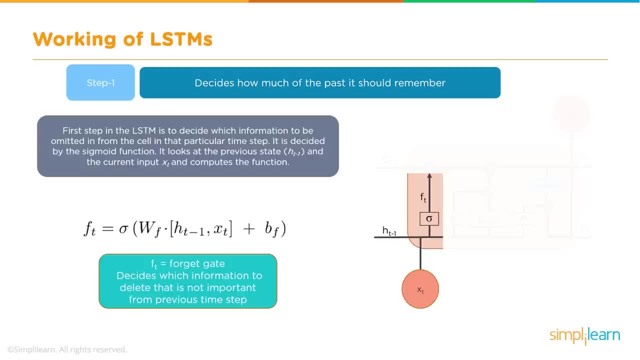 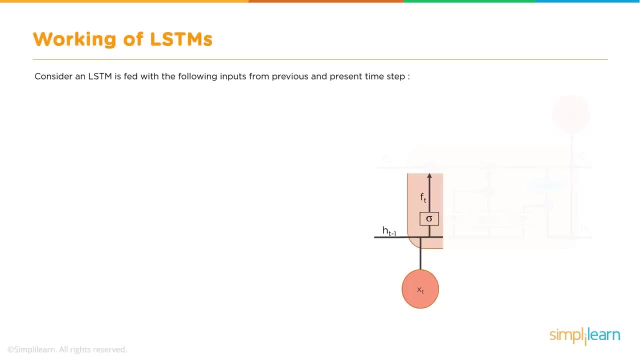 with any of our neural networks. so we have a bias function. So f at t equals forget gate Decides which information to delete that is not important from the previous time step. Consider again. LSTM is fed with the following inputs from the previous and present time step: 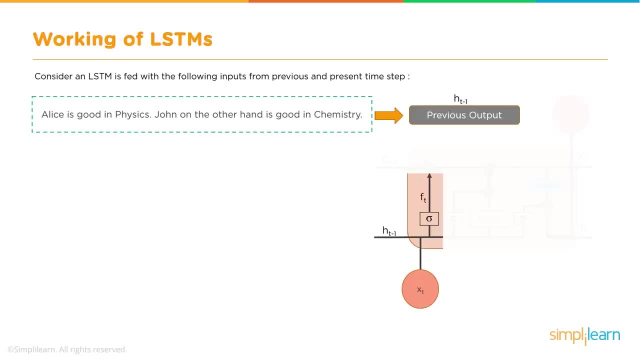 Alice is good in physics. John, on the other hand, is good in chemistry. So previous output: John plays football well. He told me yesterday over the phone that he had served as a captain of his college football team. That's our current input. 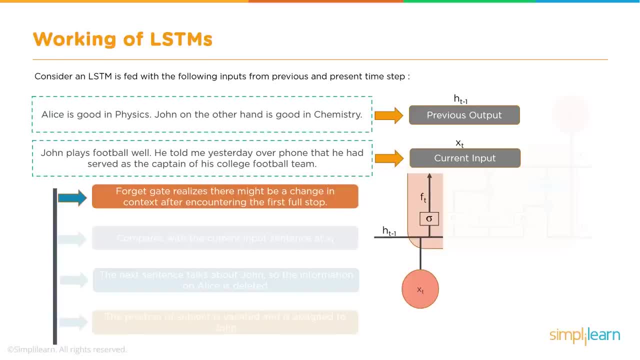 So, as we look at this, the first step is the forget gate realizes there might be a change in context after encountering the first full stop. It compares with the current input sentence of x at t- So we're looking at that full stop- and then compares it with the input of the new sentence. 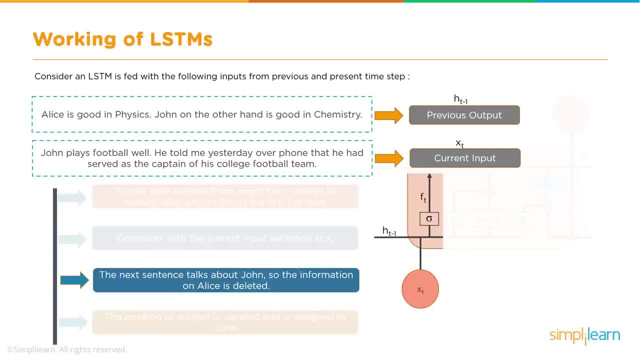 The next sentence talks about John, so the information on Alice is deleted. Okay, that's important to know. So we have this input coming in and if we're going to continue on with John, then that's going to be the primary information we're looking at. 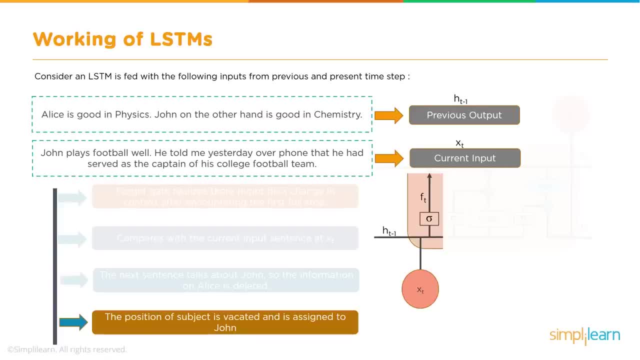 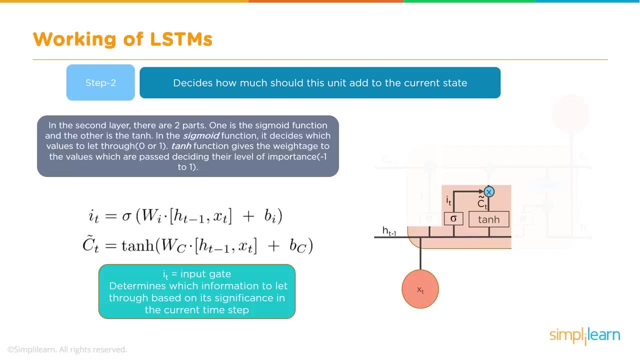 The position of the subject is vacated and is assigned to John, And so in this one we've seen that we've weeded out a whole bunch of information and we're only passing information on John. that's now the new topic. So step two is then to decide how much should this unit 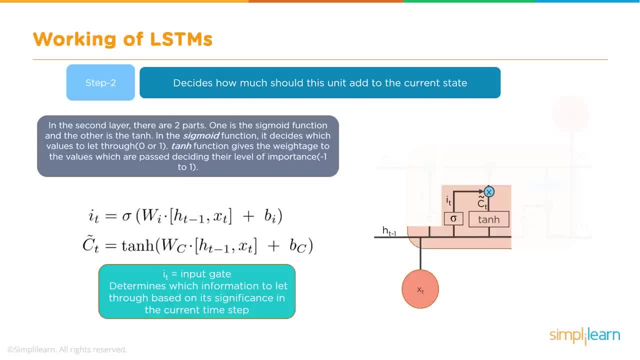 add to the current state. In the second layer there are two parts. One is the sigmoid function and the other is the tangent h. In the sigmoid function it decides which values to let through: 0 or 1.. Tangent h function gives the weightage to the values which are passed. 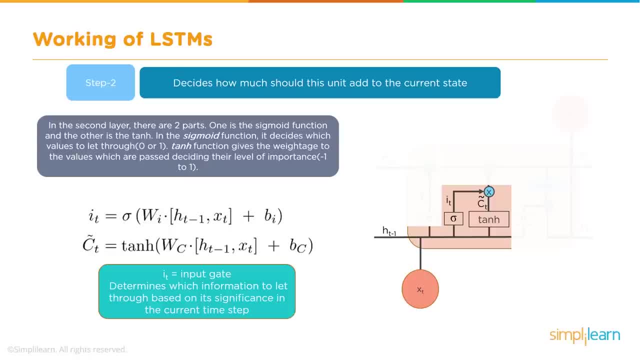 deciding their level of importance minus 1 to 1.. And you can see the two formulators that come up. the i of t equals the sigmoid of the weight of i, h of t minus 1, x of t plus the bias of i. 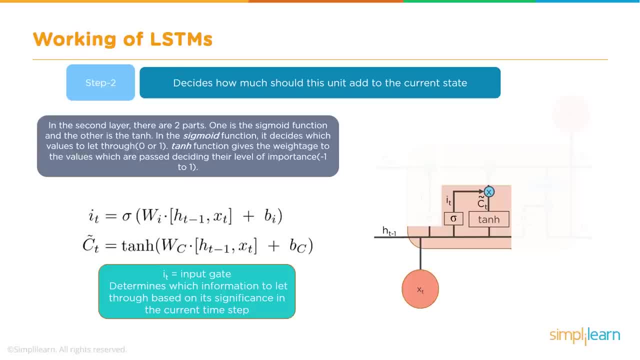 And the c of t equals the tangent of h, of the weight of c, of h of t minus 1, x of t plus the bias of c. So our i of t equals the input gate determines which information to let through based on its significance in the current time step. 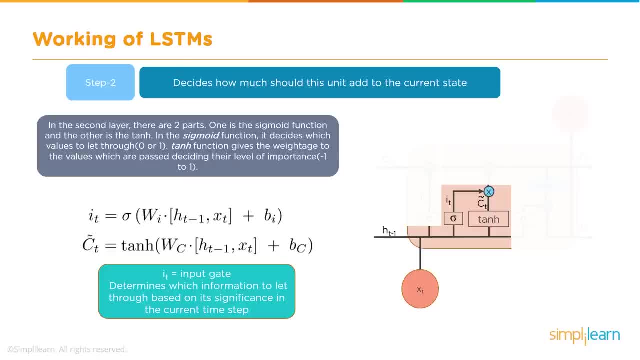 If this seems a little complicated, don't worry, because a lot of the programming is already done when we get to the case study. Understanding, though, that this is part of the program is important when you're trying to figure out what to set your settings at. 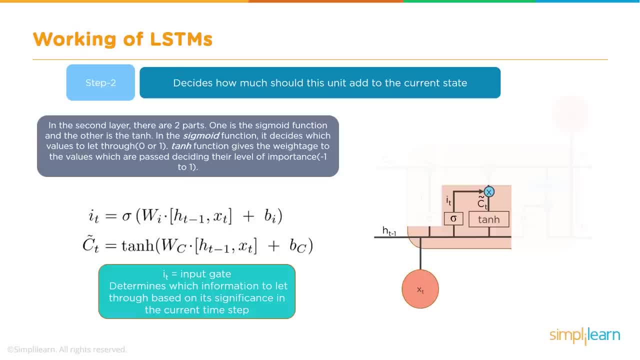 You should also note when you're looking at this. it should have some semblance to your forward propagation neural networks, where we have a value assigned to a weight plus a bias, Very important steps in any of the neural network layers, whether we're propagating into them the information. 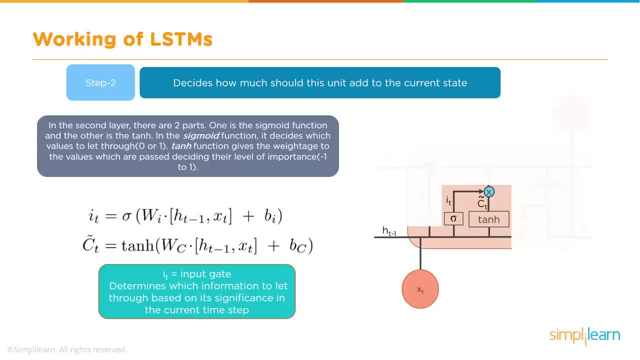 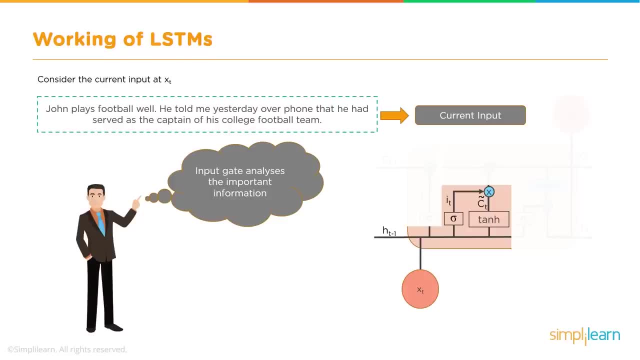 from one to the next, or we're just doing a straightforward neural network propagation. Let's take a quick look at this: what it looks like from the human standpoint. as I step out of my suit again, Consider the current input at x of t. 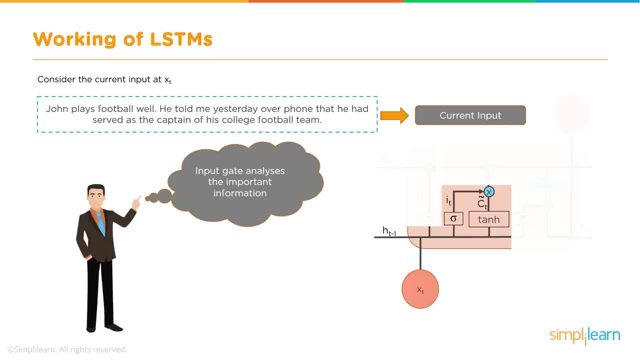 John plays football well. He told me yesterday over the phone that he had served as a captain of his college football team. That's our input Input gate. analyses the important information- John plays football and he was a captain of his college team- is important. 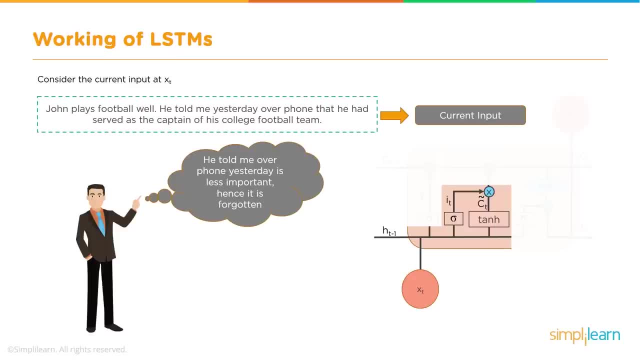 He told me over the phone yesterday, is less important, hence it is forgotten. This process of adding some new information can be done via the input gate. Now, this example is as a human form, and we'll look at training this stuff in just a minute. 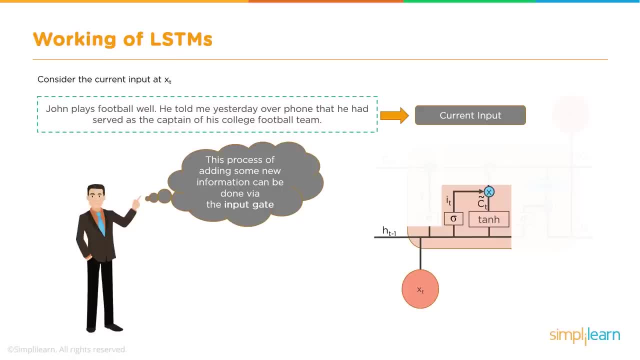 But as a human being, if I wanted to get this information from a conversation- maybe it's a Google Voice listening in on you or something like that- how do we weed out the information that he was talking to me on the phone yesterday? Well, I don't want to memorize that he talked to me. 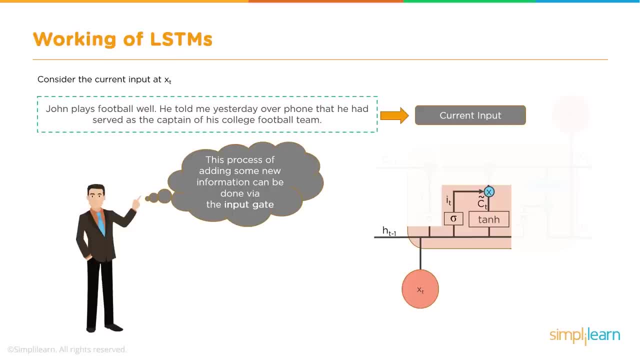 on the phone yesterday- or maybe that is important, but in this case it's not. I want to know that he was the captain of the football team. I want to know that he served. I want to know that John plays football and he was a captain of the college football team. 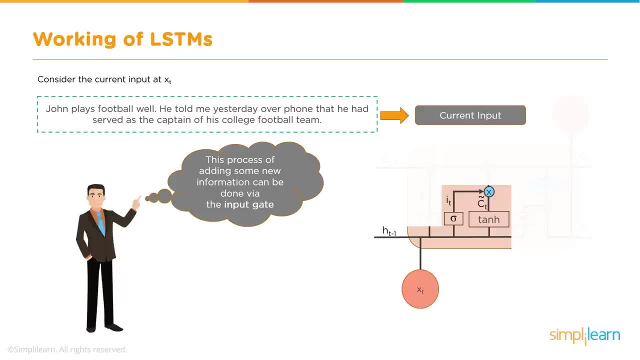 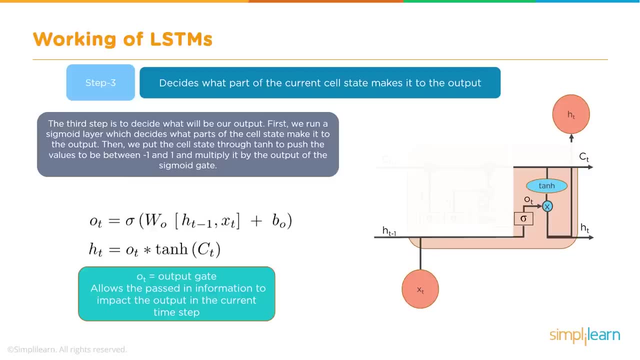 Those are the two things that I want to take away as a human being. Again, we measure a lot of this from the human viewpoint and that's also how we try to train them so we can understand these neural networks. Finally, we get to step three. 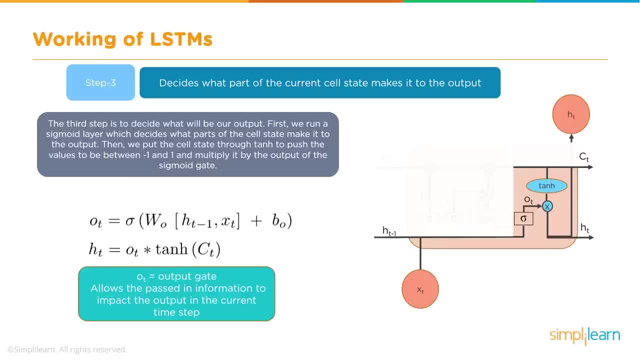 which decides what part of the current cell state makes it to the output. The third step is to decide what will be our output. First we run a sigmoid layer which decides what parts of the cell state make it to the output. Then we put the cell state through the tangent h. 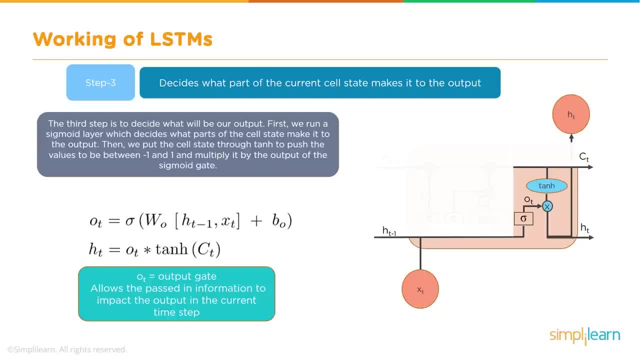 to push the values to be between minus one and one and multiply it by the output of the sigmoid gate. So when we talk about the output of t, we set that equal to the sigmoid of the weight of zero of the h of t minus one. 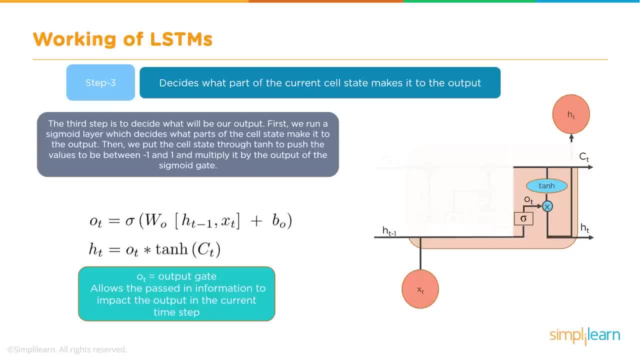 and back one step in time by the x of t plus, of course, the bias. The h of t equals the out of t times the tangent h of c of t. So our o of t equals the output gate. allows the passed in information. 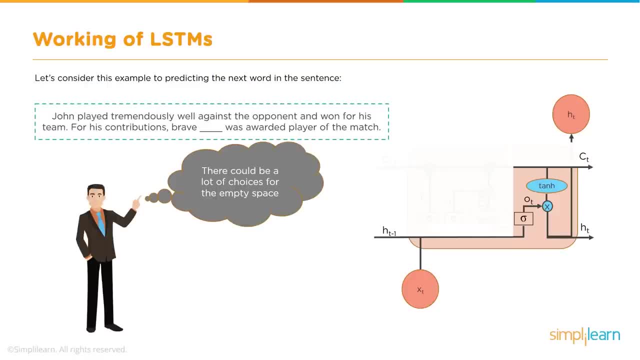 to impact the output in the current time step. Let's consider the example to predicting the next word in the sentence. John played tremendously well against the opponent and won for his team. For his contributions, brave blank was awarded. player of the match. There could be a lot of choices for the empty space. 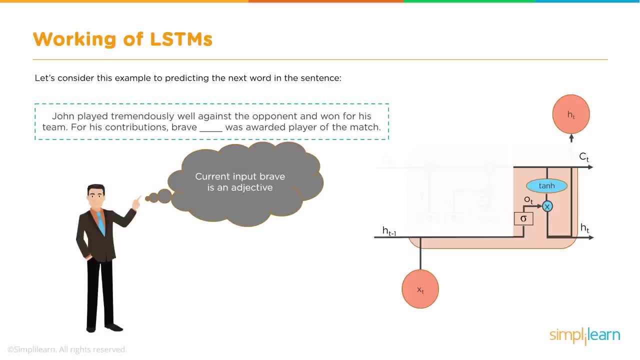 Current input. brave is an adjective. Adjectives describe a noun. John could be the best output after brave. Thumbs up for John, awarded player of the match. And if you were to pull just the nouns out of the sentence, team doesn't look right. 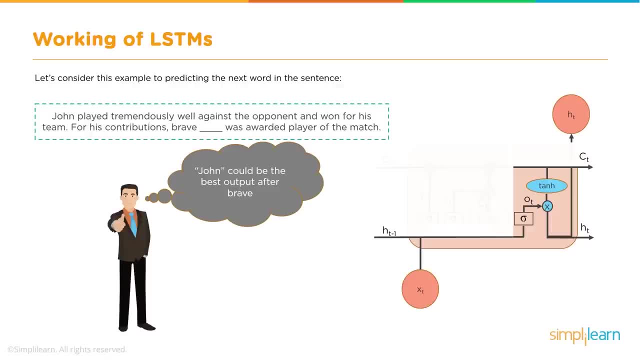 because that's not really the subject. we're talking about Contributions. you know brave contributions or brave team, brave player, brave match, so you look at this and you can start to train this, this neural network. so it starts looking at it and goes. 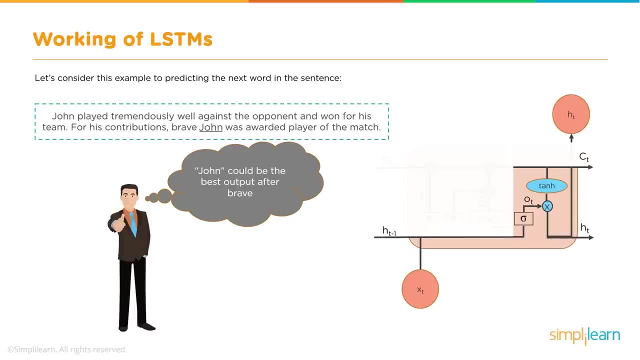 oh no, John is what we're talking about. So brave is an adjective, John's going to be the best output, And we give John a big thumbs up. And then, of course, we jump into my favorite part, the case study. 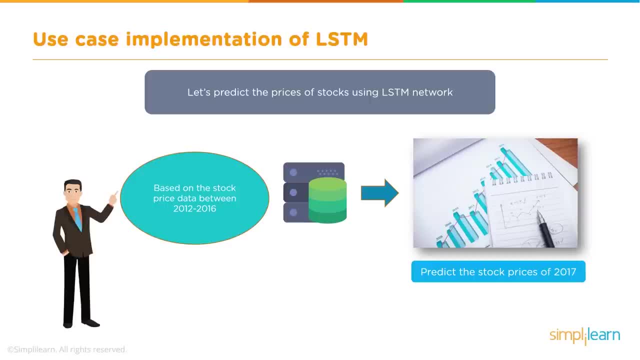 Use case: implementation of LSTM. Let's predict the prices of stocks using the LSTM network, Based on the stock price data between 2012,- 2016,. we're going to try to predict the stock prices of 2017.. And this will be a narrow set of data. 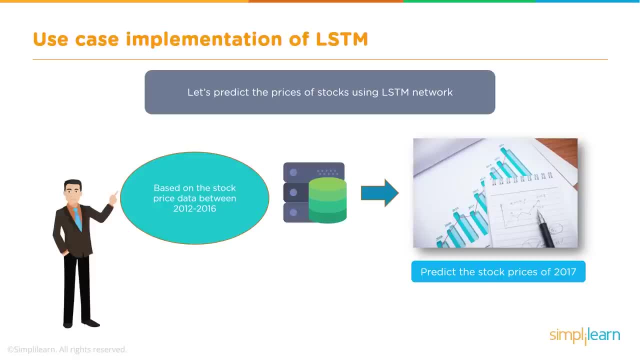 We're not going to do the whole stock market. It turns out that the New York Stock Exchange generates roughly three terabytes of data per day. That's all the different trades up and down of all the different stocks going on, And each individual one second to second. 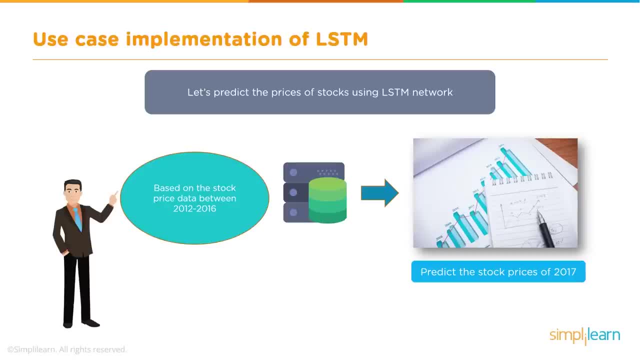 or nanosecond to nanosecond, But we're going to limit that to just some very basic fundamental information. So don't think you're going to get rich off this today, But at least you can give a step forward in how to start processing something like stock prices. 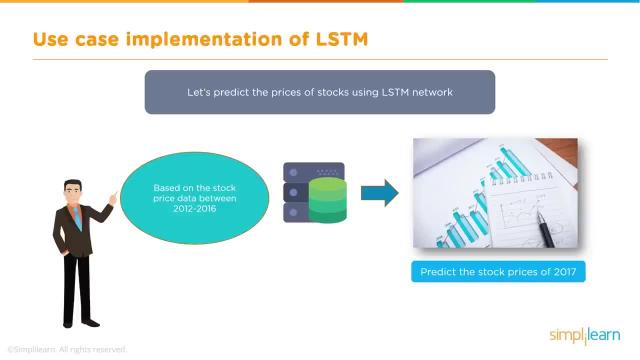 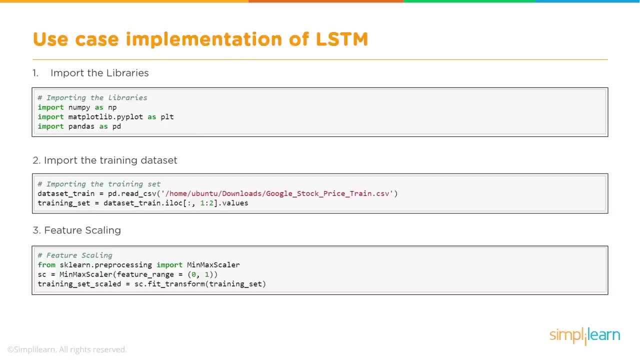 a very valid use for machine learning in today's markets. Use case implementation of LSTM. Let's dive in. We're going to import our libraries. We're going to import the training set and get the scaling going Now, if you watch any of our other tutorials, 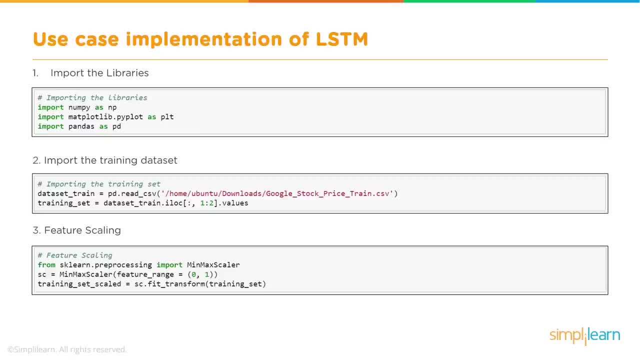 a lot of these pieces just start to look very familiar. It's a very similar setup. Let's take a look at that. and just a reminder: we're going to be using Anaconda, the Jupyter notebook, So here I have my Anaconda navigator. 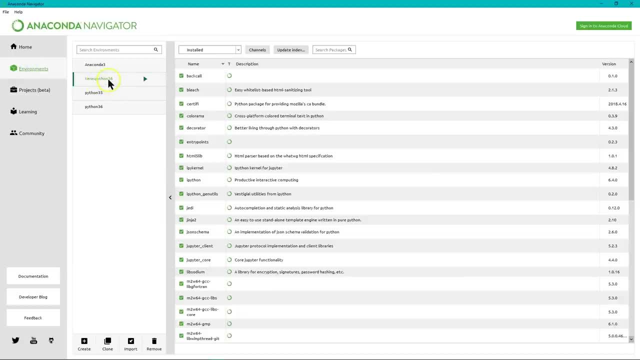 When we go under environments. I've actually set up a cross, Python 3.6.. I'm in Python 3.6.. And the nice thing about Anaconda, especially the newer version. I remember a year ago messing with Anaconda and different versions of Python in different environments. 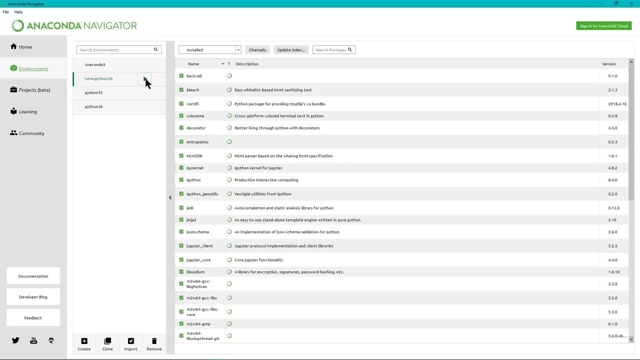 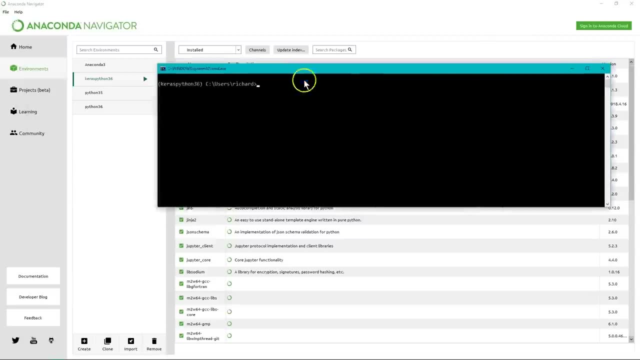 Anaconda now has a nice interface And I have this installed both on a Ubuntu Linux machine and on Windows so it works fine on there And you can go in here and open a terminal window And then in here once you're in the terminal window. 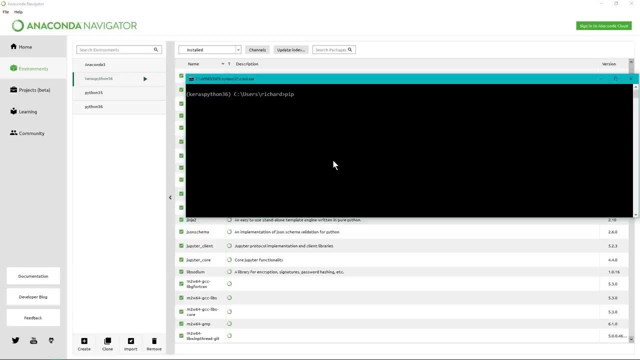 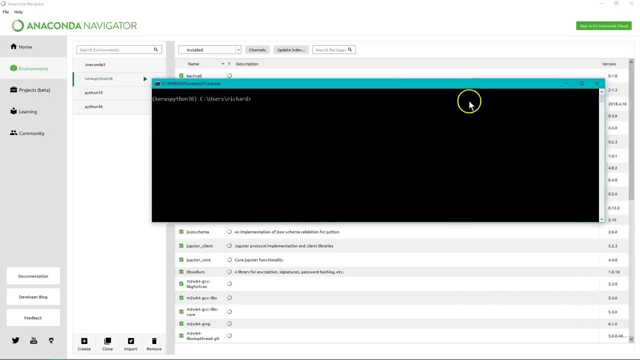 this is where you're going to start installing, using pip to install your different modules and everything. Now we've already pre-installed them, so we don't need to do that in here, But if you don't have them installed in your particular environment, you'll need to do that. 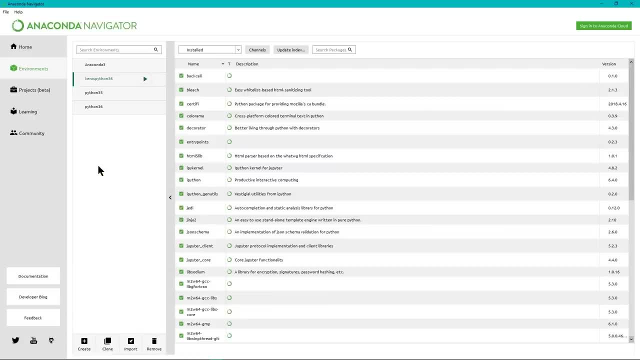 And of course you don't need to use the Anaconda or the Jupyter. You can use whatever favorite Python IDE you like. I'm just a big fan of this because it keeps all my stuff separate. You can see, on this machine. 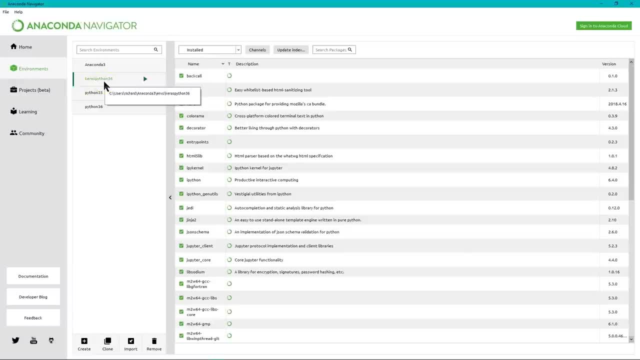 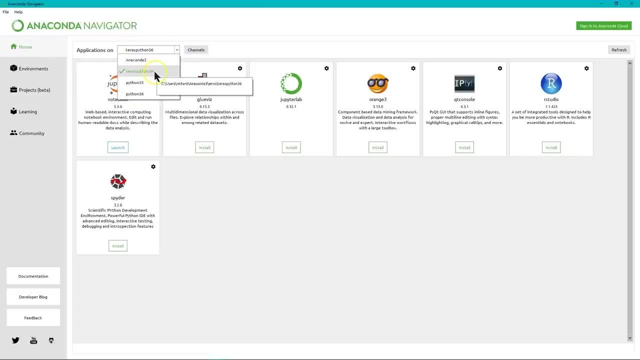 I have specifically installed one for Keras, since we're going to be working with Keras under TensorFlow When we go back to Home. I've gone up here to Application and that's the environment I've loaded on here And then we'll click on the Launch. Jupyter Notebook. 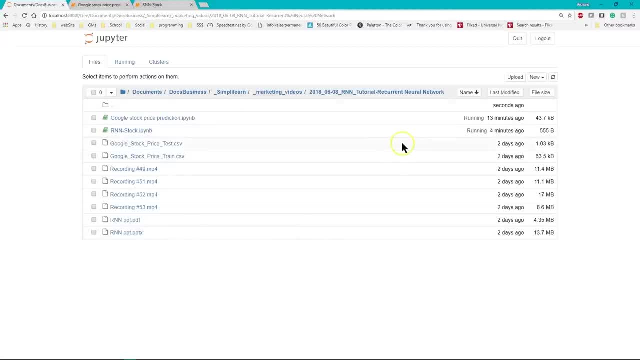 Now I've already, in my Jupyter Notebook, have set up a lot of stuff so that we're ready to go kind of like Martha Stewart's in the old cooking shows. We want to make sure we have all our tools for you. 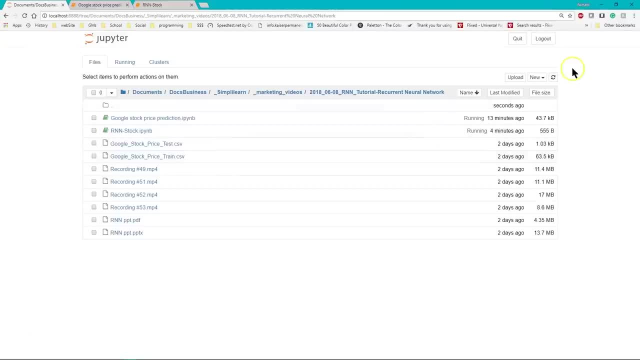 so you're not waiting for them to load, And if we go up here to where it says New, you can see where you can create a new Python 3.. That's what we did here underneath the setup, so it already has all the modules installed on it. 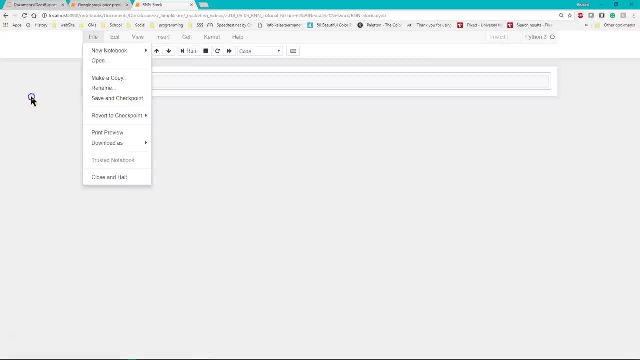 And I've actually renamed this. If you go under File, you can rename it. I'm calling it RNN Stock And let's just take a look and start diving into the code. Let's get into the exciting part Now. we've looked at the tool. 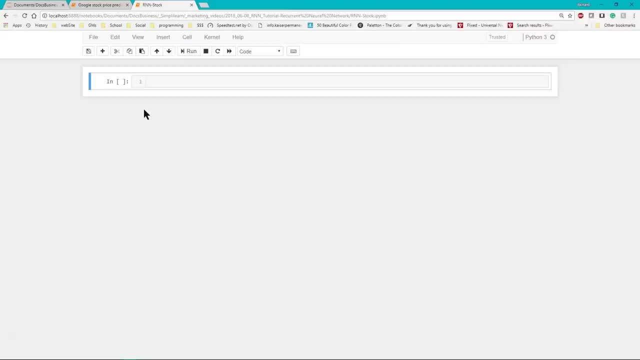 and, of course, you might be using a different tool, which is fine. Let's start putting that code in there and seeing what those imports and uploading everything looks like. Now the first half is kind of boring when we hit the Run button. 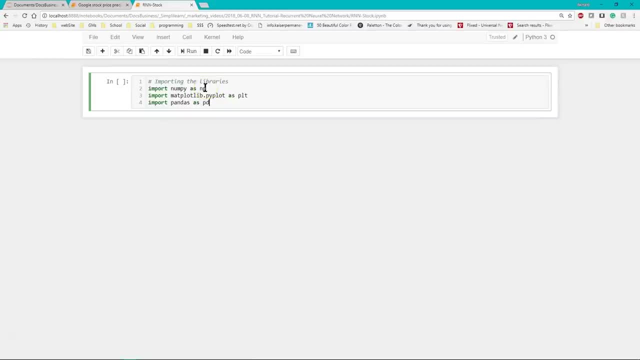 Because we're going to be importing numpy as np- That's the number- Python, which is your numpy array, And the matplot library, because we're going to do some plotting at the end, And our pandas for our data set, Our pandas as pd. 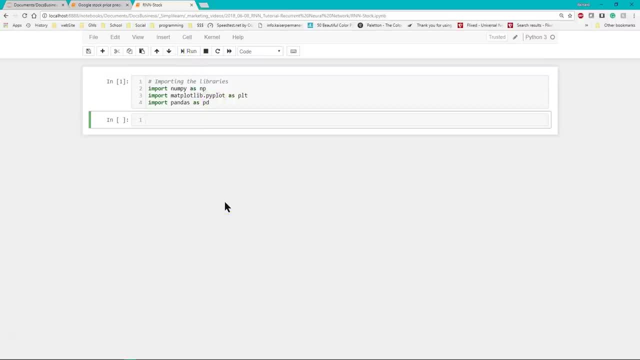 And when I hit Run it really doesn't do anything except for load those modules. Just a quick note. Let me just do a quick draw here. Oops, Shift-Alt, There we go. You'll notice when we're doing this setup. 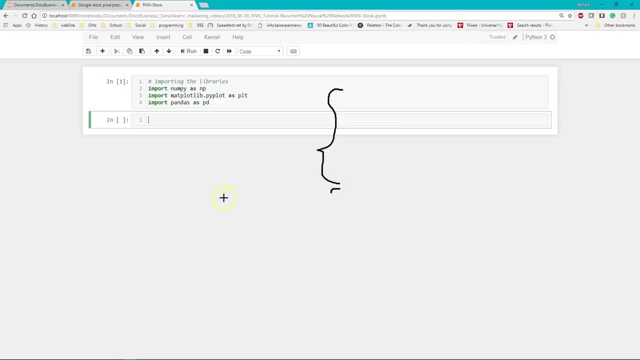 if I was to divide this up. oops, I'm going to actually overlap these. Here we go. This first part that we're going to do is our data prep- A lot of prepping involved, In fact, depending on what your system is. 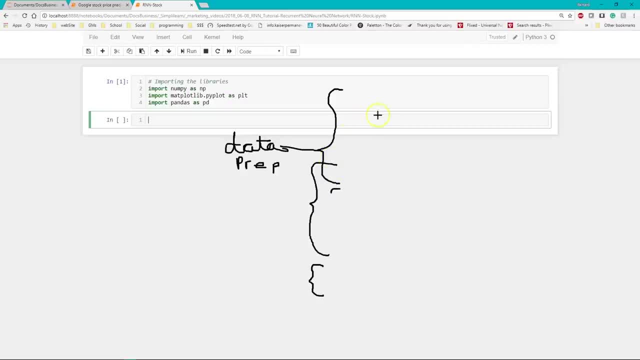 since we're using Keras, I put an overlap here, But you'll find that almost, maybe even half of the code we do is all about the data prep And the reason I overlap this with Keras. let me just put that down. 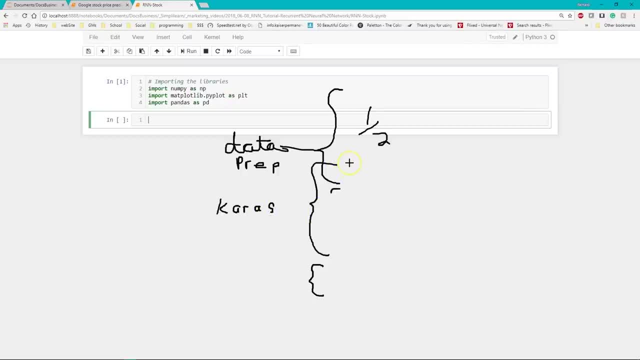 because that's what we're working in- is because Keras has like their own preset stuff, So it's already pre-built in, which is really nice. So there's a couple steps, a lot of times, that are in the Keras setup. 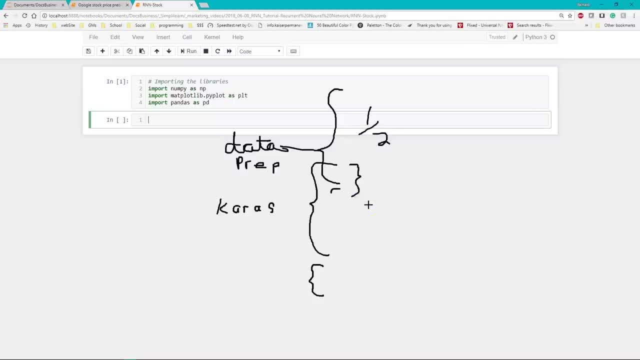 We'll take a look at that to see what comes up in our code as we go through and look at stock. And then the last part is to evaluate And if you're working with shareholders or classroom, whatever it is you're working with. 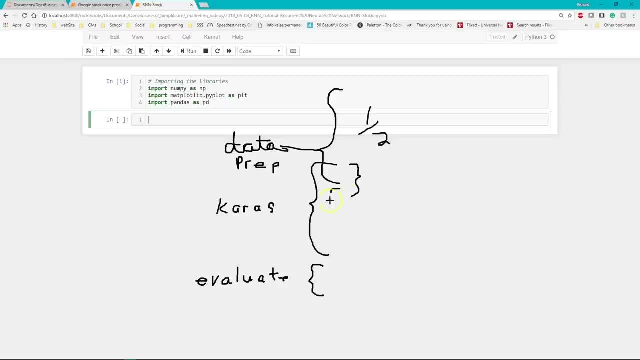 the evaluate is the next biggest piece. So the actual code here, Keras, is a little bit more, but when you're working with some of the other packages you might have like three lines. That might be it. All your stuff is in your pre-processing. 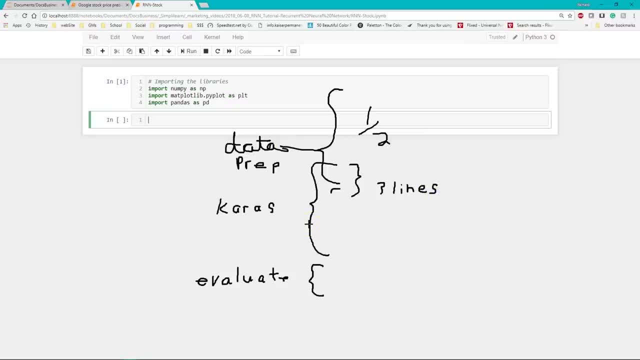 and your data, Since Keras is cutting edge and you load the individual layers, you'll see that there's a few more lines here and Keras is a little bit more robust, And then you spend a lot of times, like I said, with the evaluate. 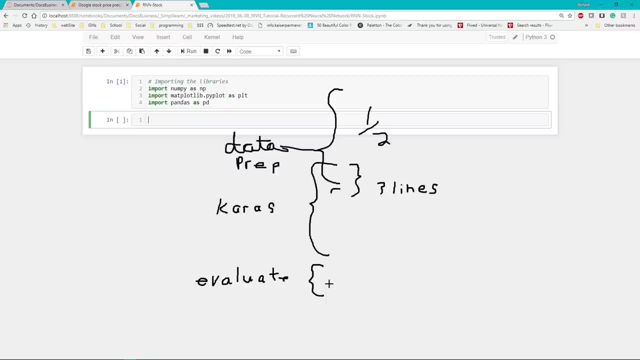 you want to have something you present to everybody else and say, hey, this is what I did, This is what it looks like. So let's go through those steps. This is like a kind of general overview And let's just take a look. 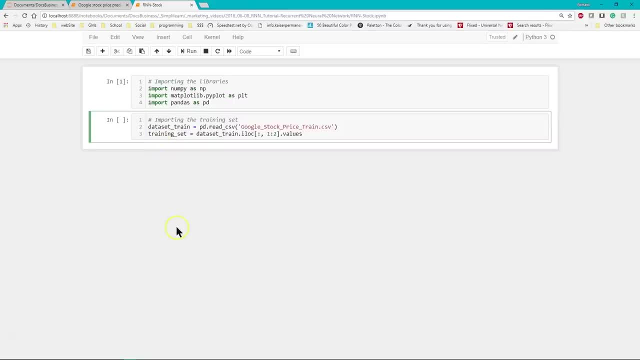 and see what the next set of code looks like. And in here we have a data set train and it's going to be read using the PD or pandas dot read CSV. And it's a Google stock price train dot CSV. And so under this, 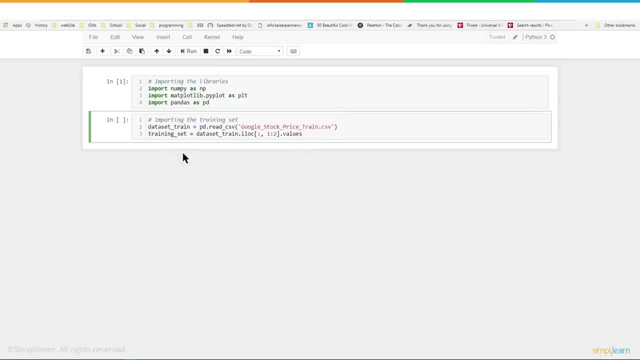 we have training set equals data set, train dot i location And we've kind of sorted out part of that. So what's going on here? Let's just take a look at and let's look at the actual file and see what's going on there. 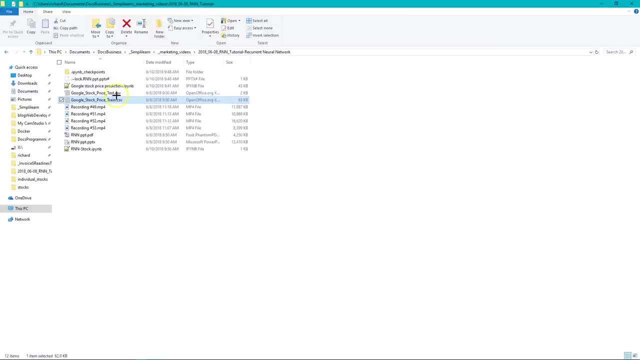 Now, if we look at this, here we go. Let's ignore all the extra files on this. I already have a train and a test set where it's sorted out. This is important to notice because a lot of times we do that as part of the preprocessing of the data. 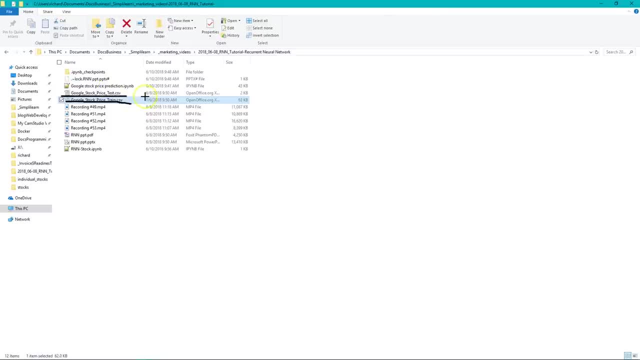 We take 20% of the data out so we can test it, and then we train the rest of it. That's what we use to create our neural network. That way we can find out how good it is. But let's go ahead and just take a look. 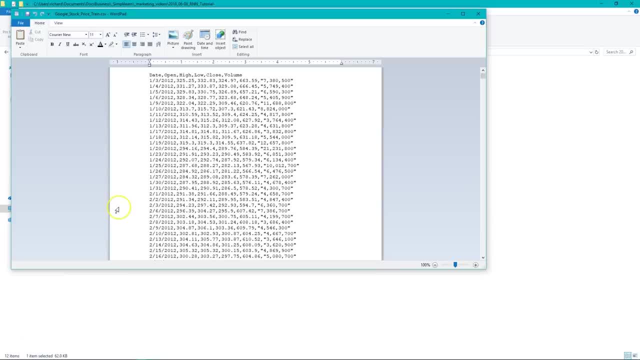 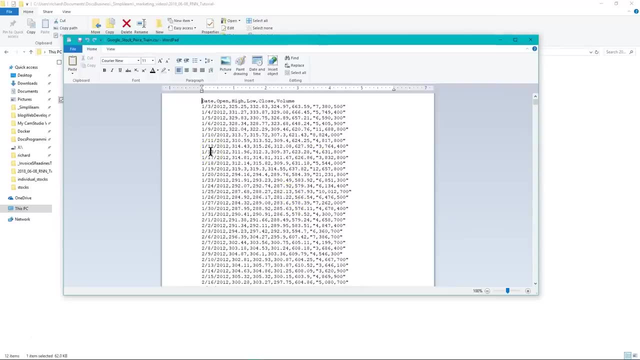 and see what that looks like. as far as the file itself- And I went ahead and just opened this up in a basic word pad and text editor just so we can take a look at it- Certainly you can open up in Excel or any other kind of spreadsheet. 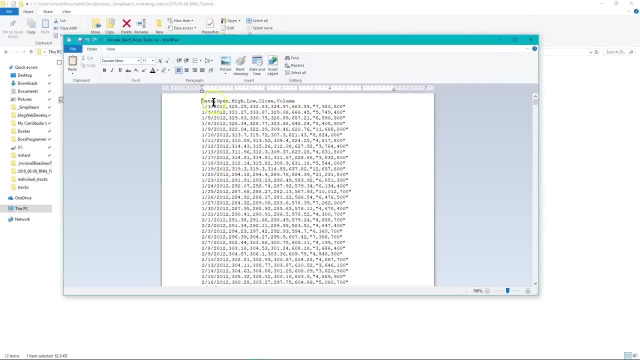 And we note that this is a comma separated variables. We have a date: open, high, low, close volume. This is the standard stuff that we import into our stock and one of the most basic set of information you can look at in stock. 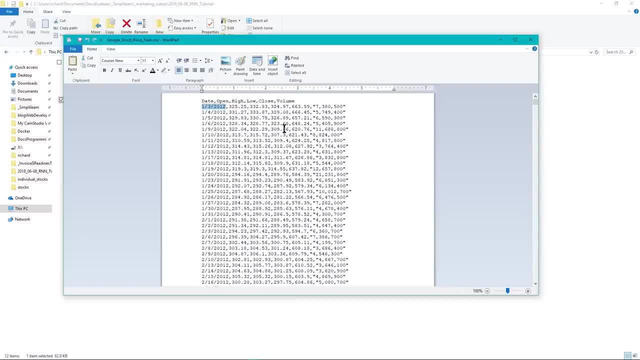 It's all free to download. In this case, we downloaded it from Google. That's why we call it the Google stock price And it specifically is Google. This is the Google stock values from. as you can see here, we started off at. 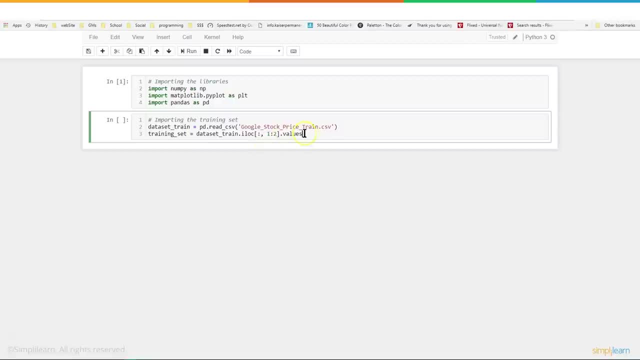 1-3-2012.. So when we look at this first setup up here we have a data set, train equals pd, underscore csv And if you noticed on the original frame, let me just go back there. they had it set to. 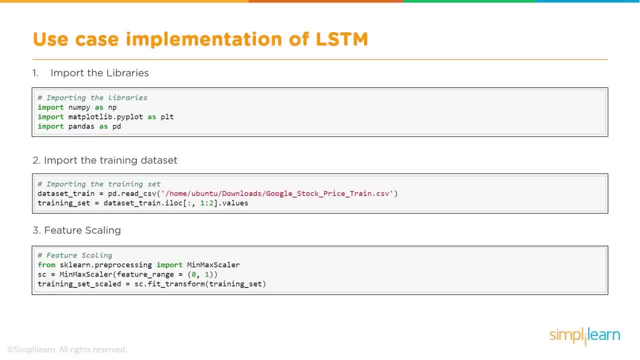 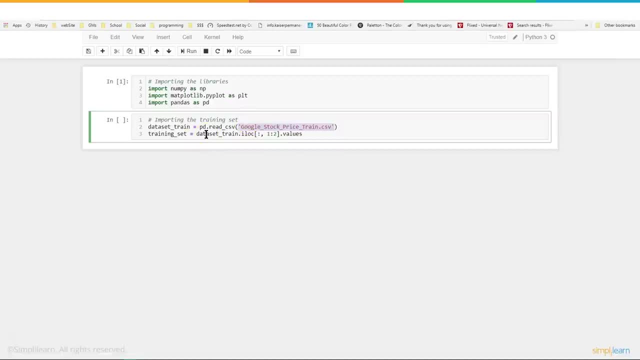 home. Ubuntu downloads. Google stock price train. I went ahead and changed that because we're in the same file where I'm running the code, So I've saved this particular Python code and I don't need to go through any special paths or have the full path on there. 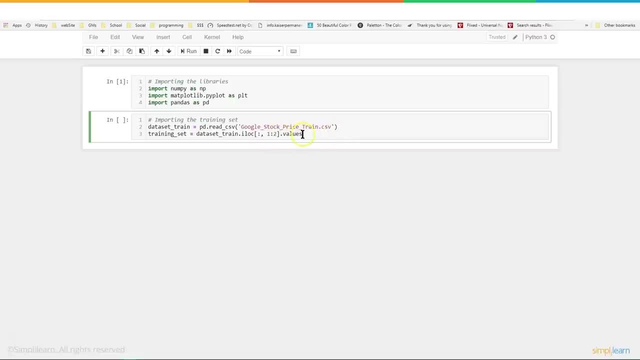 And then, of course, we want to take out certain values in here, And you're going to notice that we're using our data set and we're now in pandas. So pandas- basically it looks like a spreadsheet, And in this case, 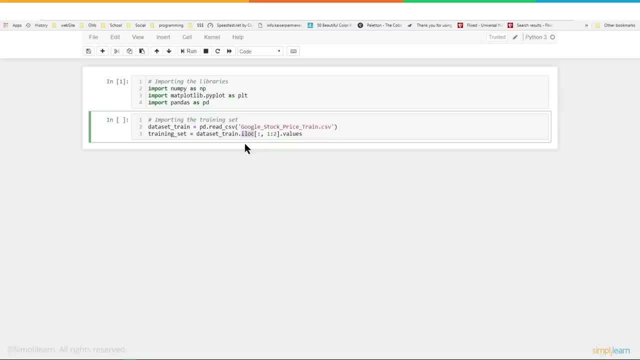 we're going to do i location, which is going to get specific locations. The first value is going to show us that we're pulling all the rows in the data, And the second one is we're only going to look at columns one and two. 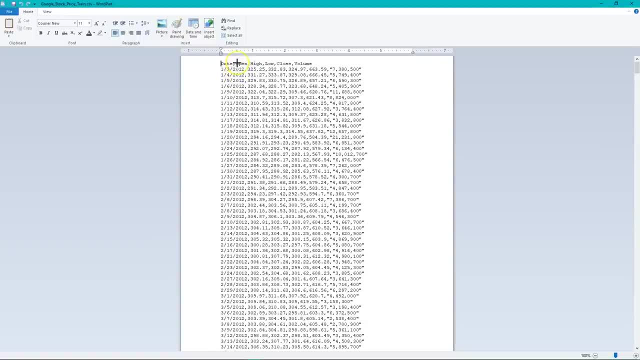 And, if you remember, here from our data, as we switch back on over columns, we always start with zero, which is the date And we're going to be looking at open and high, which would be one and two. We'll just label that right there. 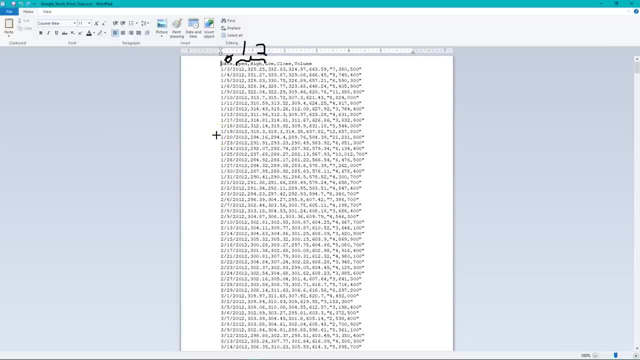 so you can see Now when you go back and do this. you certainly can extrapolate and do this on all the columns, But for the example let's just limit a little bit here so that we can focus on just some key aspects of stock. 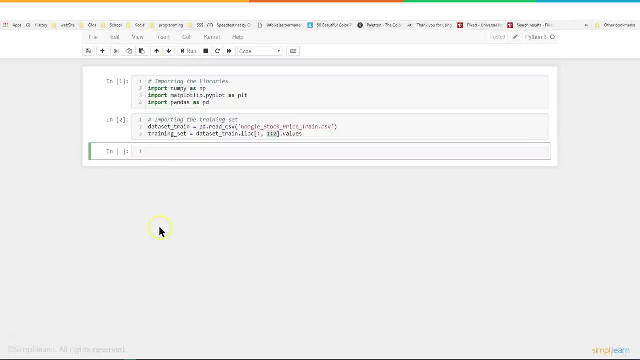 And then we'll go up here and run the code. And again, I said, the first half is very boring. Whenever we hit the run button, it doesn't do anything because we're still just loading the data and setting it up. Now that we've loaded our data, 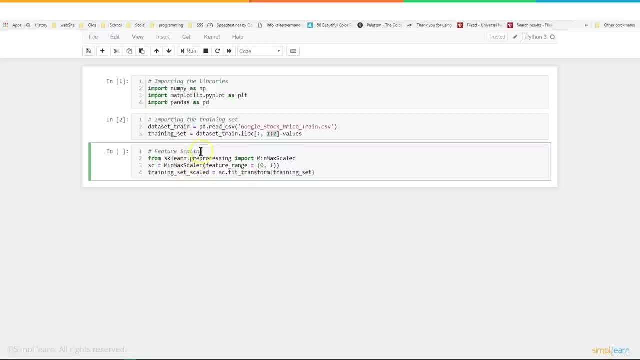 we want to go ahead and scale it. We want to do what they call feature scaling And in here we're going to pull it up from the sklearn or the skkit, preprocessing import minmax scalar. And when you look at this you got to remember: 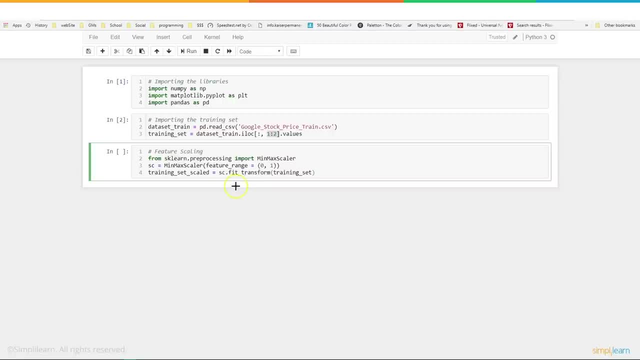 that biases in our data. we want to get rid of that. So if you have something that's like a really high value, let's just draw a quick graph, And I have something here like maybe the stock has a value. One stock has a value of 100. 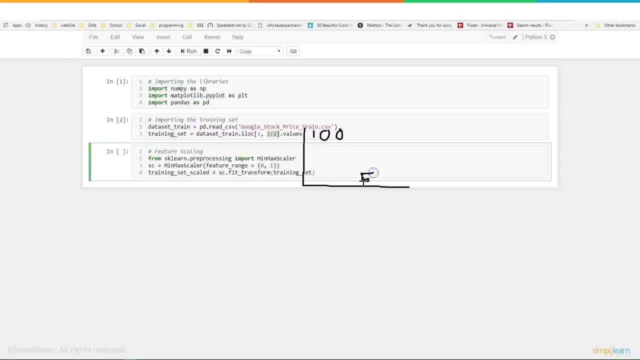 and another stock has a value of 5. You start to get a bias between different stocks, And so when we do this, we go ahead and say, okay, 100 is going to be the max and 5 is going to be the min. 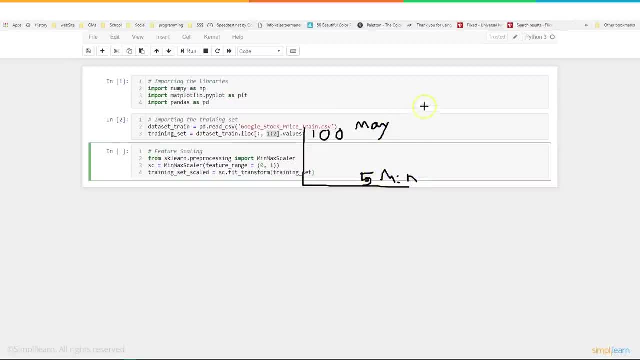 And then everything else goes to the max, And then we change this, So we just squish it down. I like the word squish. So it's between 1 and 0.. So 100 equals 1 or 1 equals 100. 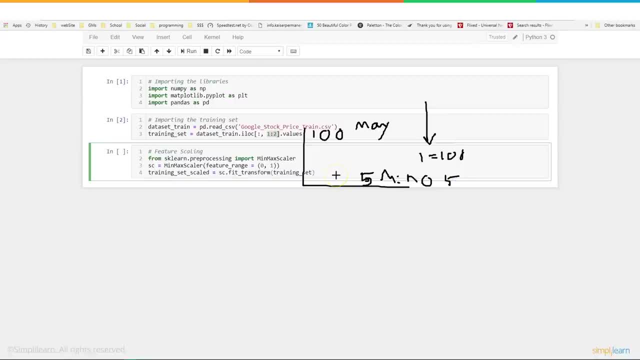 and 0 equals 5. And you can just multiply. It's usually just a simple multiplication. we're using Multiplication, So it's going to be minus 5 and then 100 divided or 95 divided by 1.. So whatever value it is, 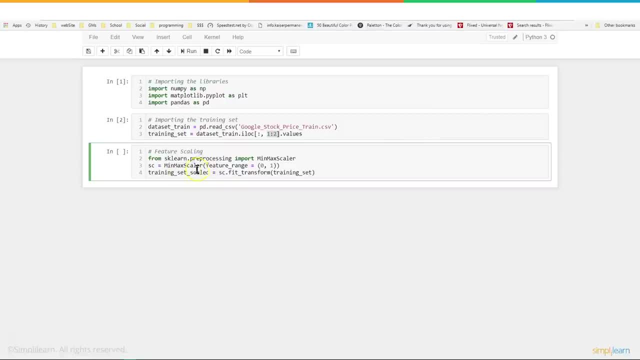 is divided by 95. And once we've actually created our scale, we're telling it's going to be from 0 to 1.. We want to take our training set and we're going to create a training set scaled And we're going to use our scalar. 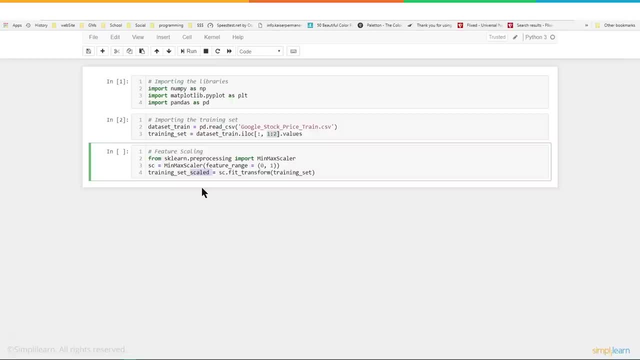 SC and we're going to fit. We're going to fit and transform the training set So we can now use the SC, this particular object. we'll use it later on our testing set Because, remember, we have to also scale that. 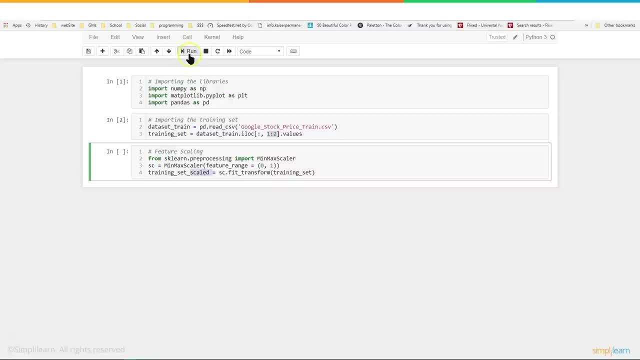 when we go to test our model and see how it works, And we'll go ahead and click on the run Again. it's not going to have any output yet because we're just setting up all the variables. Okay, so we paste the data in here. 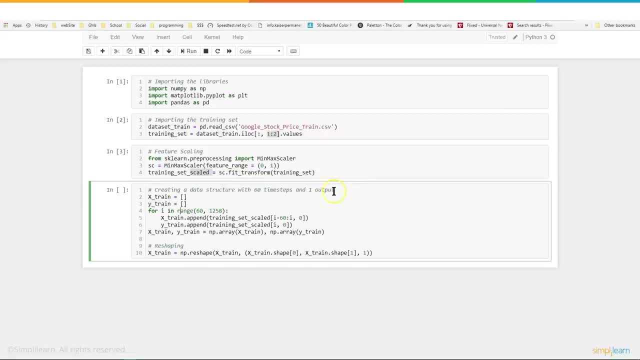 and we're going to create the data structure with the 60 time steps and output. First note: we're running 60 time steps And that is where this value here also comes in. So the first thing we do is we create our X train and Y train variables. 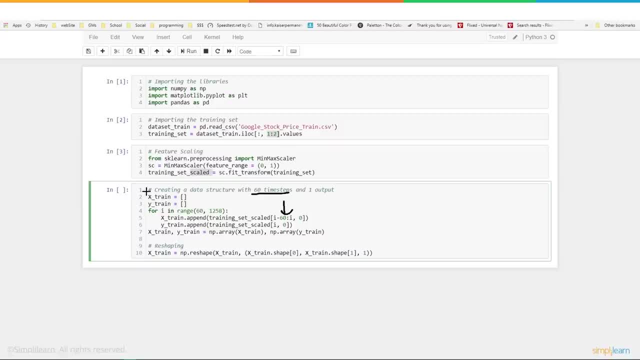 and we set them to an empty Python array- Very important to remember what kind of array we're in and what we're working with. And then we're going to come in here. We're going to go for I in range 60 to 1258.. 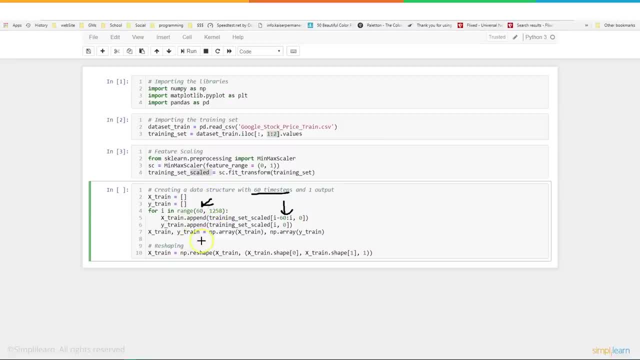 There's our 60, 60 time steps, And the reason we want to do this is, as we're adding the data in, there's nothing below the 60. So if we're going to use 60 time steps, we have to start at point 60. 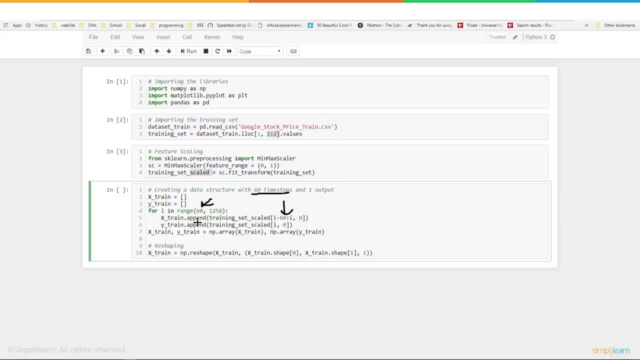 because it includes everything underneath of it. Otherwise you'll get a pointer error. And then we're going to take our X train and we're going to append training set scaled. This is a scaled value between 0 and 1.. And then, as I, is equal to 60,. 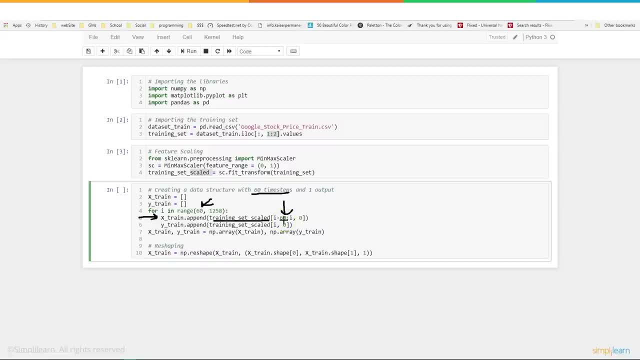 this value is going to be 60 minus 60 is 0. So this actually is 0 to I. So it's going to be 0 to 60, 1 to 61.. Let me just circle this part right here. 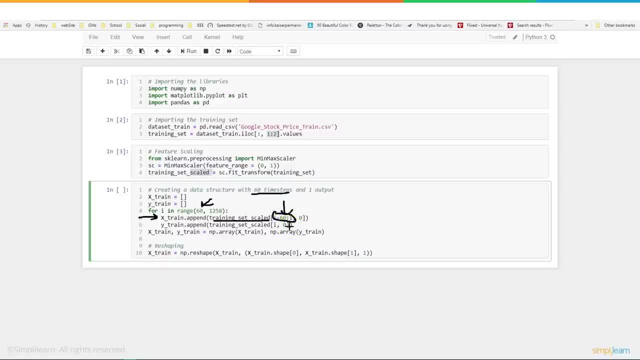 1 to 61,, 2 to 62, and so on and so on. And, if you remember, I said 0 to 60. That's incorrect because it does not count. Remember, it starts at 0.. So this is a count of 60. 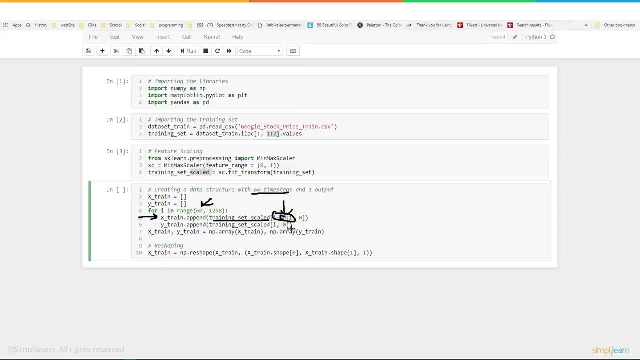 So it's actually 59. Important to remember that as we're looking at this And then the second part of this that we're looking at. So, if you remember correctly, here we go From 0 to 59 of I And then we have a comma a, 0, right here. 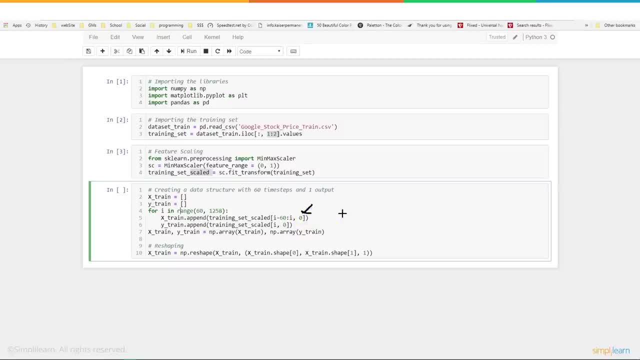 So, finally, we're just going to look at the open value. I know we did put it in there for 1 to 2.. If you remember correctly, it doesn't count the second one, So it's just the open value we're looking at. 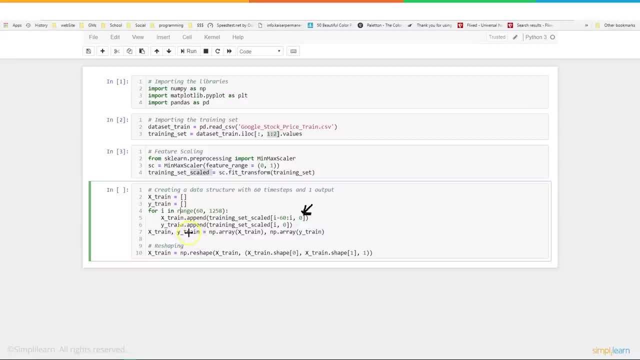 Just open. And then finally, we have Y train dot. append training set I to 0. And if you remember correctly, I comma 0. If you remember correctly, this is 0 to 59. So there's 60 values in it. 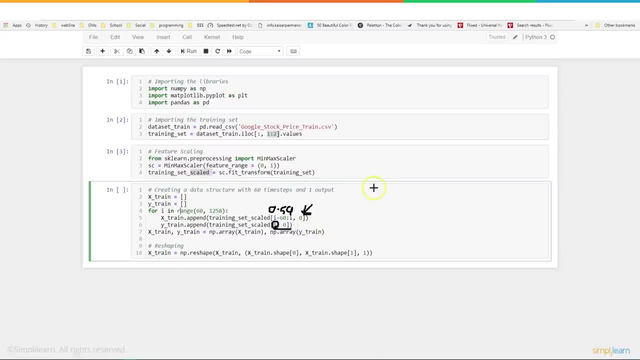 So when we do, I down here, this is number 60. So we're going to do this as we're creating an array And we have 0 to 59. And over here we have number 60, which is going into the Y train. 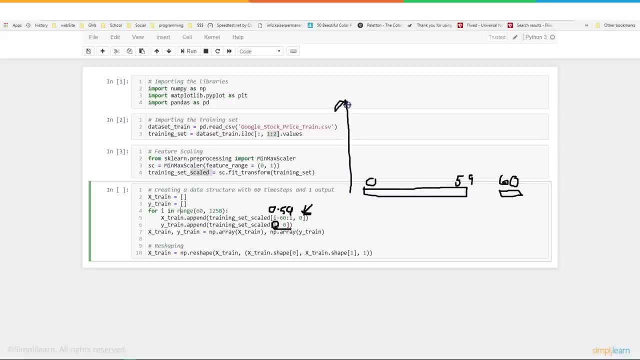 It's being appended on there And then this just goes all the way up. So this is down. here is 0 to 59. And we'll call it 60., Since that's the value over here, And it goes all the way up to 1258.. 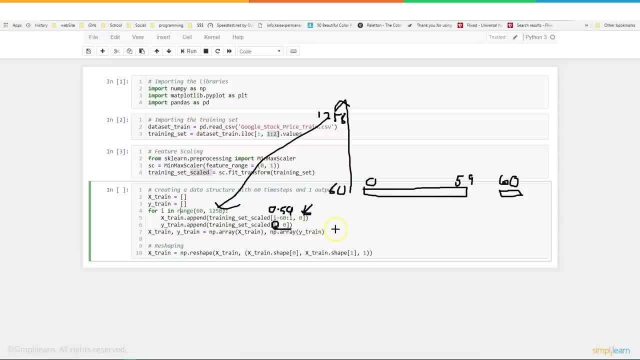 That's where this value here comes in. That's the length of the data we're loading. So we've loaded two arrays. We've loaded one array that has, which is filled with arrays from 0 to 59. And we loaded one array which is just the value. 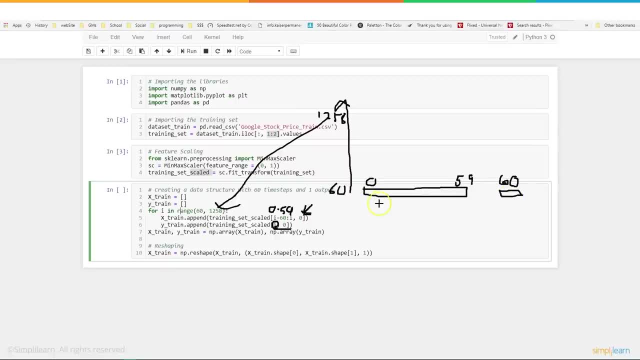 And what we're looking at. you want to think about this as a time sequence. Here's my open, open, open, open, open open. What's the next one in the series? So we're looking at the Google stock. 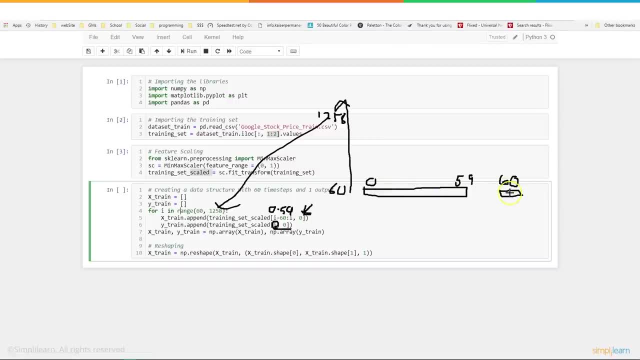 And each time it opens, we want to know what the next one? 0 through 59,, what's 60?? 1 through 60, what's 61?? 2 through 62, what's 62? And so on, and so on, going up. 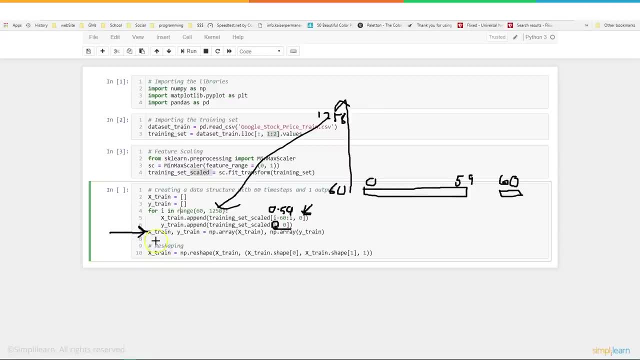 And then, once we've loaded those in our for loop, we go ahead and take X train and Y train: equals NP dot array X train dot NP array Y train. We're just converting this back into a numpy array. That way we can use all the cool tools that we get with numpy array, including reshaping. 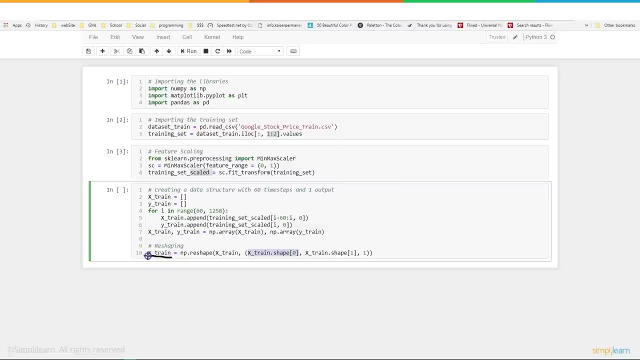 So if we take a look and see what's going on here, we're going to take our X train, We're going to reshape it. Wow, what the heck does reshape mean? That means we have an array, if you remember correctly. 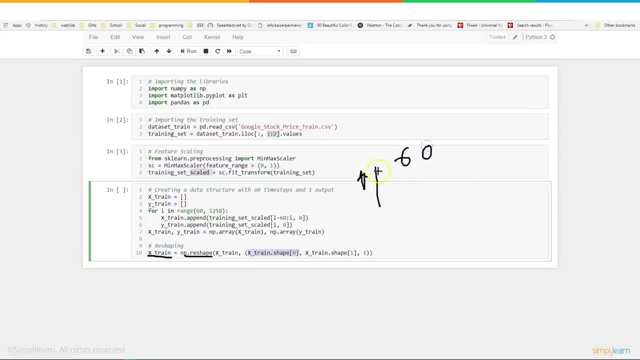 so many numbers by 60.. That's how wide it is, And so when you do X train dot shape, that gets one of the shapes. And you get X train dot shape of one gets the other shape, And we're just making sure the data is formatted correctly. 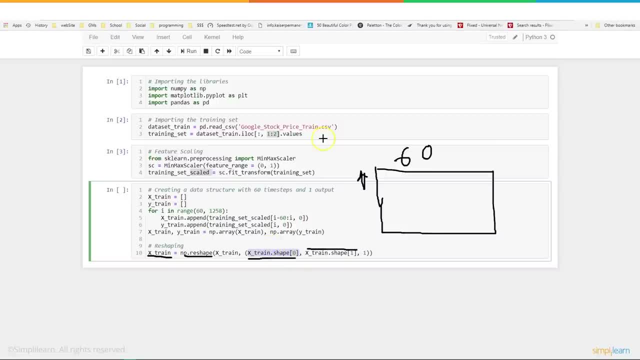 And so you use this to pull the format. The fact that it's 60 by in this case, where's that value 60 by 1199, 1258 minus 60, 1199.. And we're making sure that that is shaped correctly. 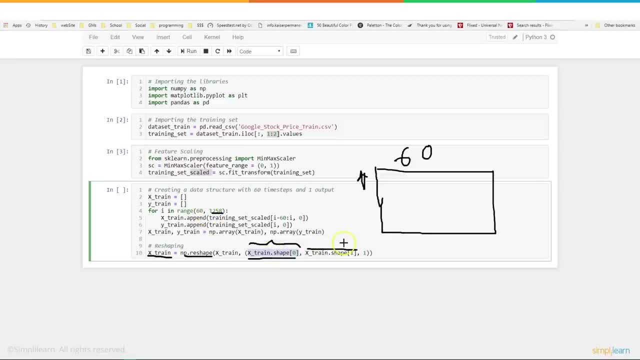 So the data is grouped into 1199 by 60 different arrays, And then the one on the end just means at the end, because when you're dealing with shapes and numpy they look at this as layers, And so the end layer needs to be one value. 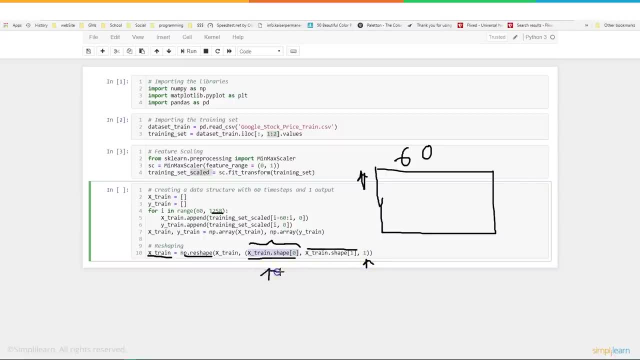 That's like the leaf of a tree, where this is the branch And then it branches out some more And then you get the leaf NP dot reshape comes from and using the existing shapes to form it, We'll go ahead and run this piece of code. 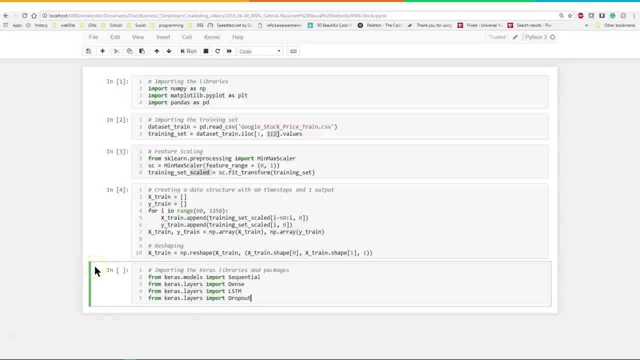 Again, there's no real output And then we'll import our different Keras modules that we need. So, from Keras models we're going to import the sequential model. We're dealing with sequential data. We have our dense layers. We have actually three layers we're going to bring in. 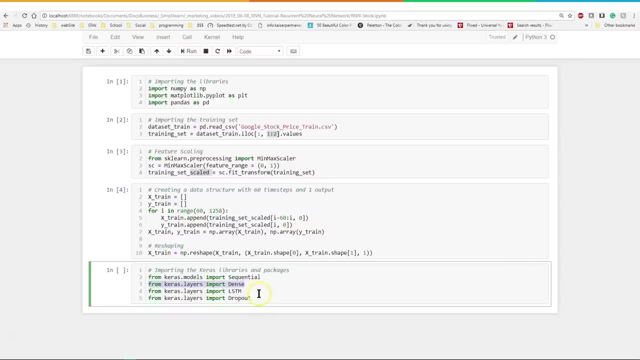 Our dense, our LSTM- which is what we're focusing on- and our dropout, And we'll discuss these three layers more in just a moment. But with the LSTM you do need the dropout And then the final layer will be the dense. 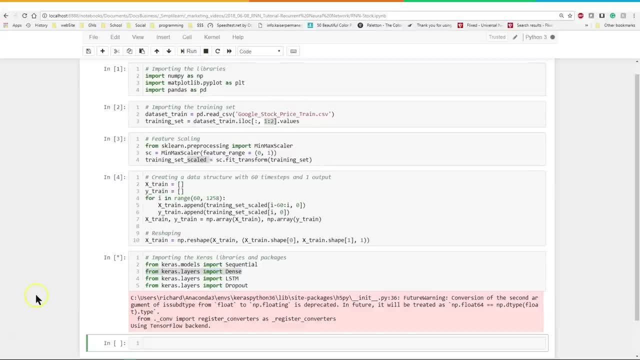 But let's go ahead and run this And that will import our modules And you'll see we get an error on here. And if you read it closer, it's not actually an error, It's a warning. What does this warning mean? 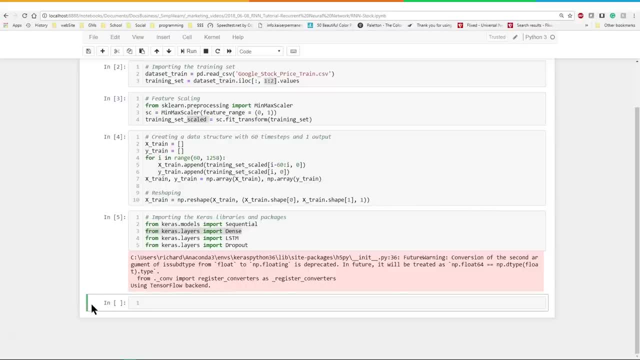 These things come up all the time when you're working with such cutting edge modules that are completely being updated all the time. We're not going to worry too much about the warning. What it's saying is that the H5PY module, which is part of Keras. 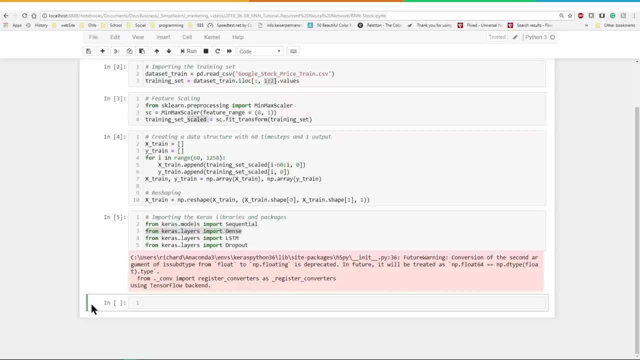 is going to be updated at some point, And if you're running new stuff on Keras and you start updating your Keras system, you better make sure that your H5PY is updated too, Otherwise you're going to have an error later on. 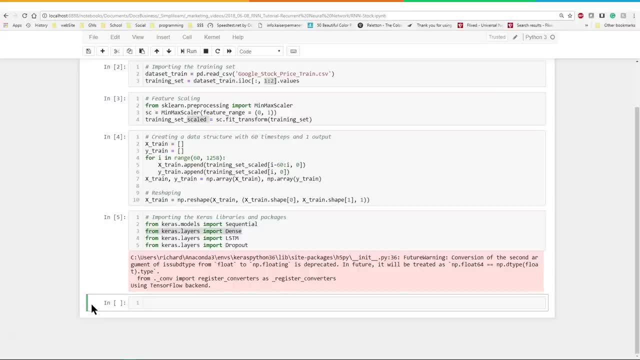 And you can actually just run an update on the H5PY now if you wanted to. Not a big deal. We're not going to worry about that today, And I said we were going to jump in and start looking at what those layers mean. 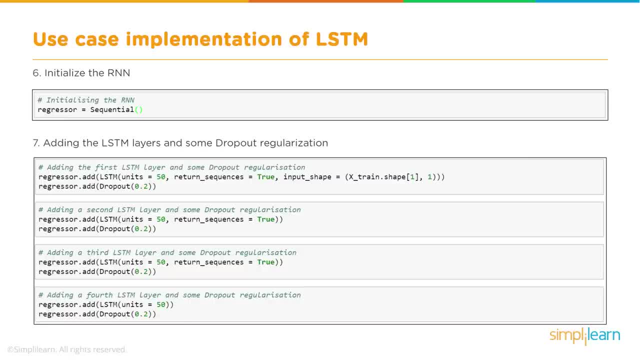 I meant that, And we're going to start off with initializing the RNN And then we'll start adding those layers in And you'll see that we have the LSTM and then the dropout, LSTM, then dropout, LSTM, then dropout. 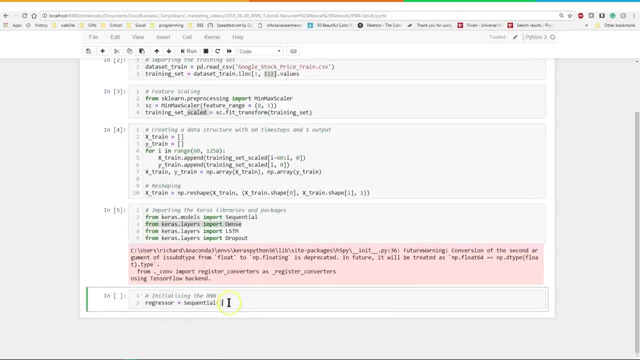 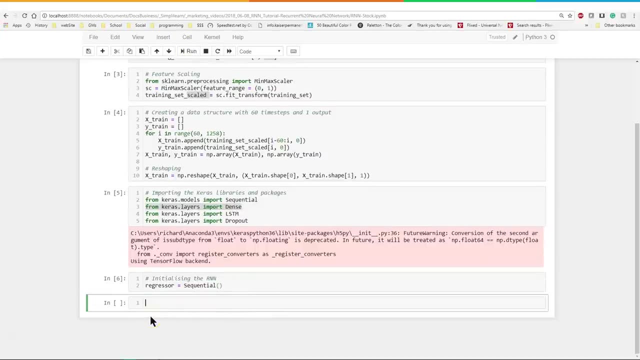 What the heck is that doing? So let's explore that. We'll start by initializing the RNN. regressor equals sequential, because we're using the sequential model- And we'll run that and load that up, And then we're going to start adding our LSTM layer and some dropout regularization. 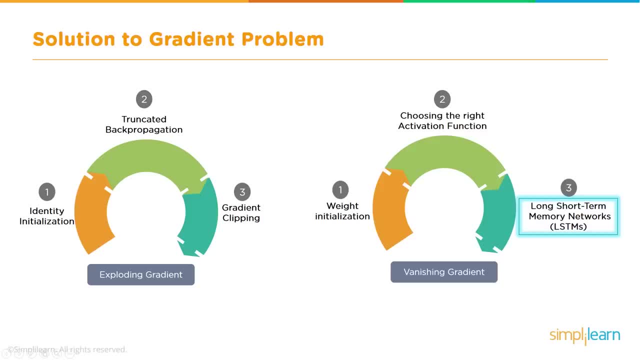 And right, there should be the Q dropout regularization. And if we go back here and remember our exploding gradient, well, that's what we're talking about. The dropout drops out unnecessary data, So we're not just shifting huge amounts of data through the network. 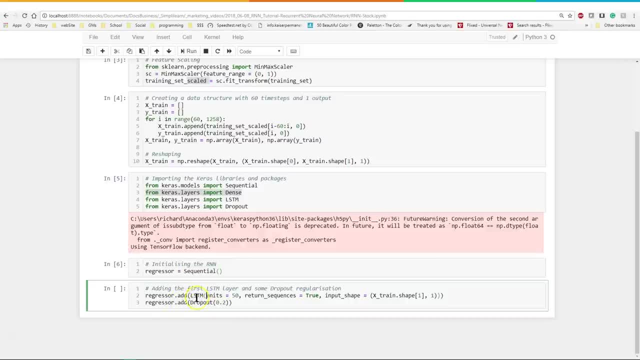 And so we go in here. Let's just go ahead and add this in. I'll go ahead and run this, And we had three of them, So let me go ahead and put all three of them in, And then we can go back over them. 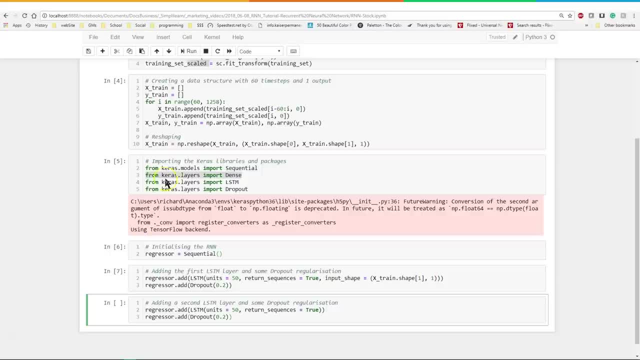 Here's the second one, And let's put one more in. Let's put that in And we'll go ahead and put two more in. I'm just going to do that. I said one more in, but it's actually two more in. 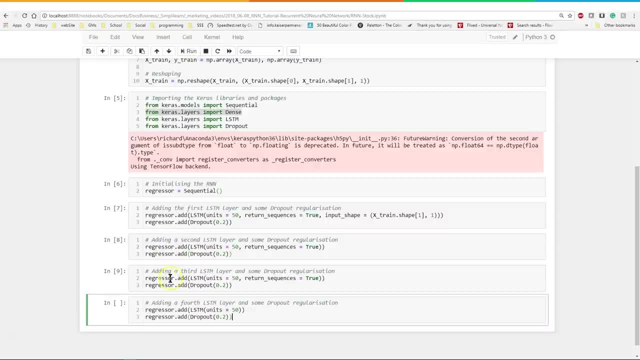 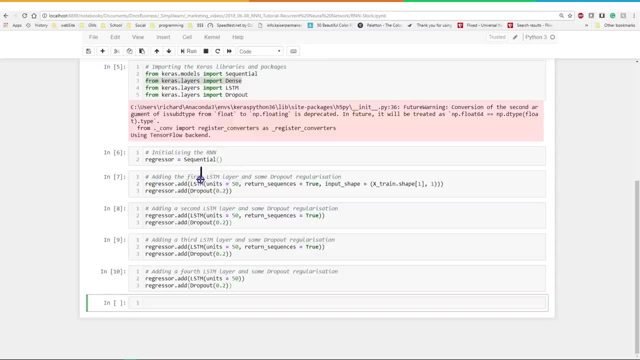 And then let's add one more after that And, as you can see, each time I run these they don't actually have an output, So let's take a closer look and see what's going on here. So we're going to add our first LSTM layer in here. 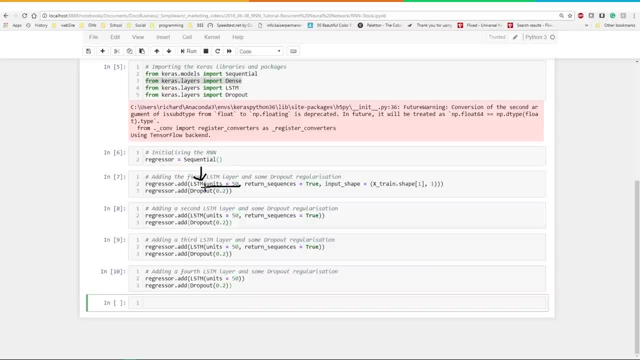 We're going to have units 50.. The units is the positive integer and it's the dimensionality of the output space. This is what's going out into the next layer. So we might have 60 coming in but we have 50 going out. 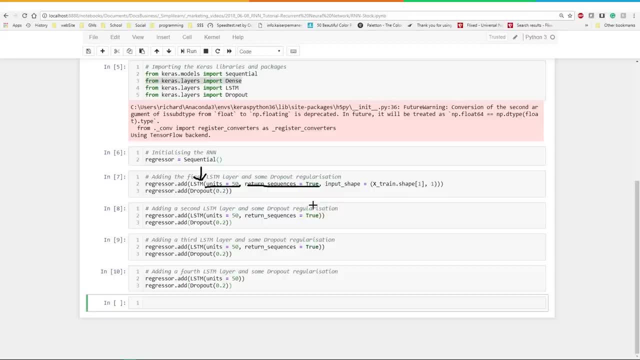 We have a return sequence. because it is a sequence data, I'm going to keep that true. And then you have to tell it what shape it's in. Well, we already know the shape by just going in here and looking at X train shape. 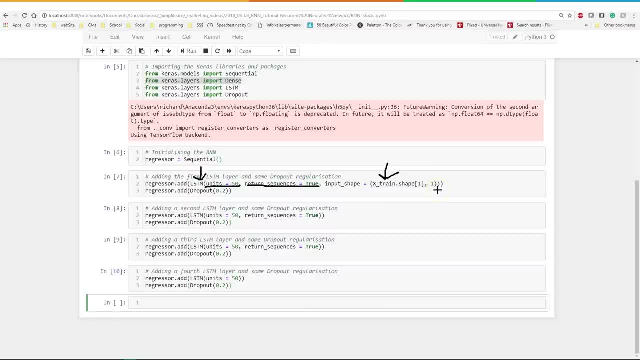 So input shape equals the X train shape of 1 comma 1.. It makes it real easy. You don't have to remember all the numbers that we put in, 60 or whatever else is in there. You just let it tell the regressor what model to use. 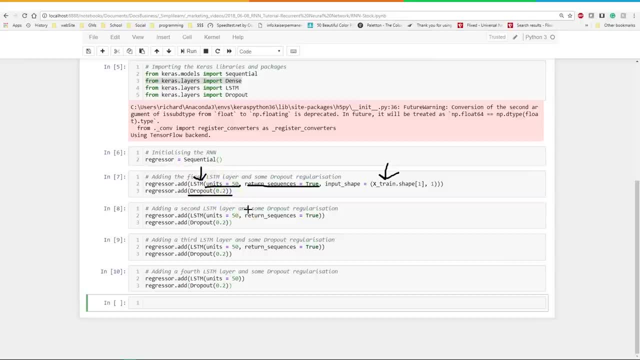 And so we follow our STM with a dropout layer. Now, understanding the dropout layer is kind of exciting, because one of the things that happens is we can overtrain our network. That means that our neural network will memorize such specific data that it has trouble predicting anything that's not in that specific realm. 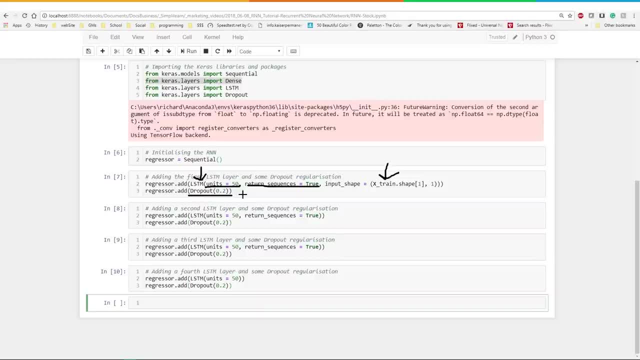 To fix for that. each time we run through the training mode, we're going to take 0.2 or 20% of our neurons and just turn them off, So we're only going to train on the other ones, And it's going to be random. 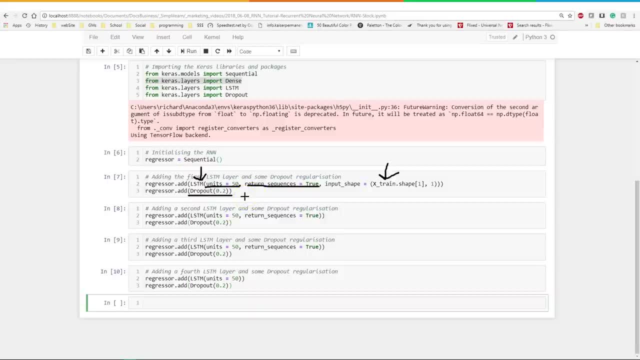 That way, each time we pass through this, we don't overtrain. These nodes come back in in the next training cycle. We randomly pick a different 20. And finally they see a big difference from the first to the second and third and fourth. 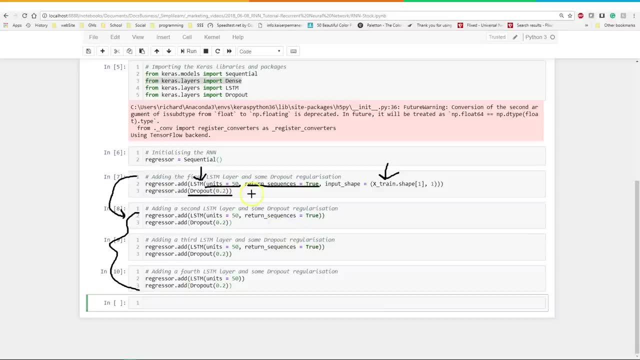 The first thing is we don't have to input the shape, Because the output units is 50 here. the next step automatically knows this layer is putting out 50. And because it's the next layer, it automatically sets that and says: oh, 50 is coming out from our last layer. 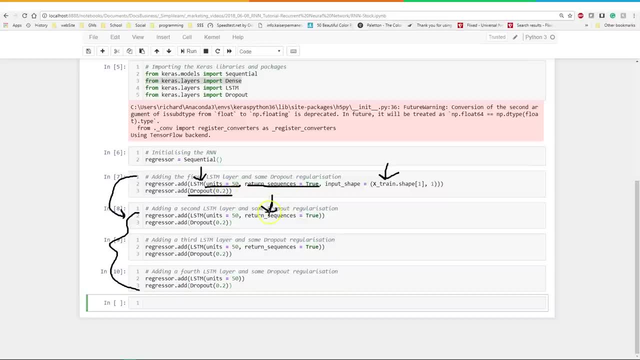 It goes into the regressor and of course we have our dropout And that's what's coming into this one, and so on and so on. And so the next three layers. we don't have to let it know what the shape is. 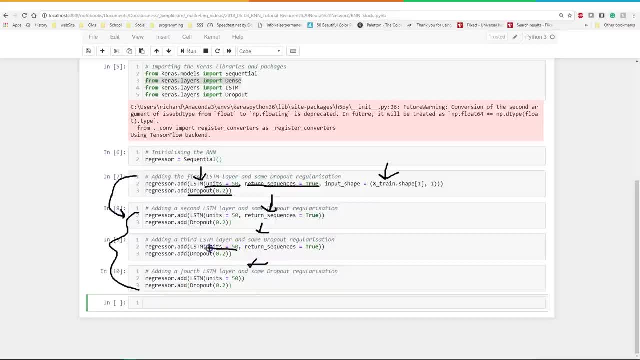 It automatically understands that And we're going to keep the units the same. We're still going to do 50 units. It's still a sequence coming through 50 units and a sequence. Now the next piece of code is what brings it all together. 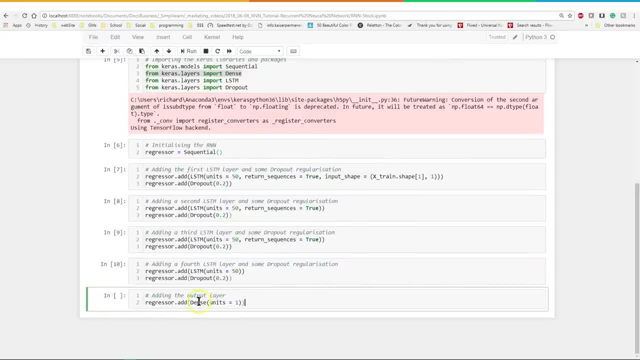 Let's go ahead and take a look at that And we come in here, We put the output layer, the dense layer And, if you remember, up here we had the three layers, We had LSTM, dropout and dense. Dense just says we're going to bring this all down into one output. 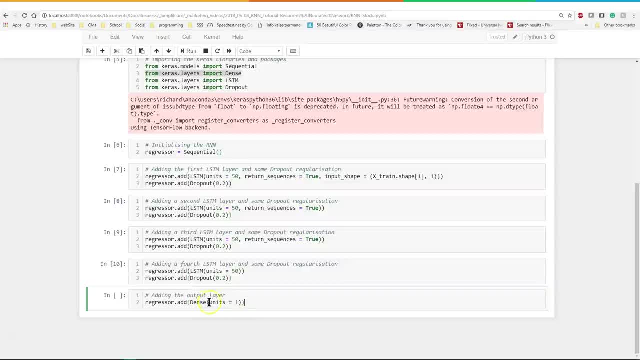 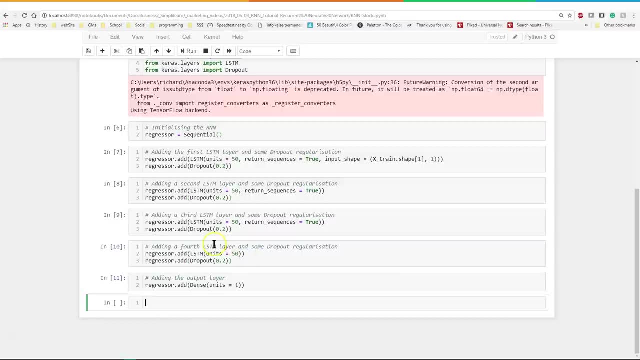 instead of putting out a sequence, We just want to know the answer at this point, And let's go ahead and run that. And so in here you notice, all we're doing is setting things up one step at a time. So far, we've brought in our way up here. 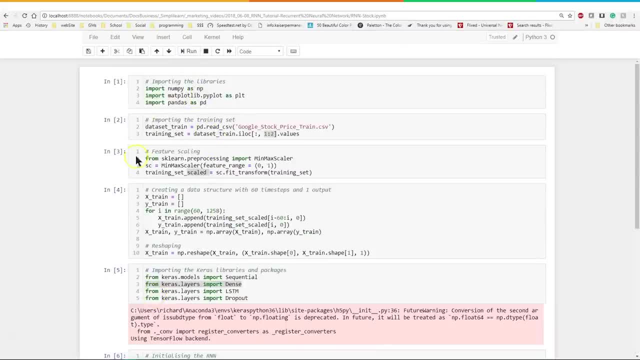 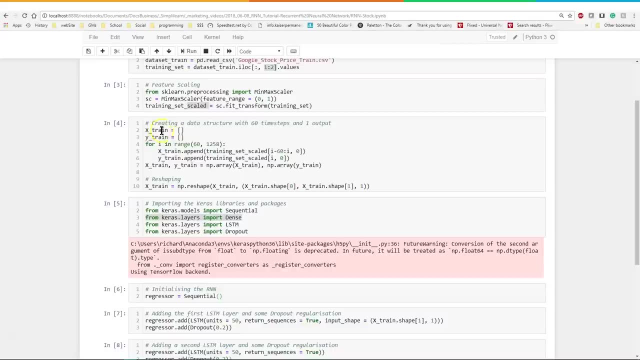 We brought in our data. We brought in our different modules. We formatted the data for training it. We set it up. We have our YX train and our Y train. We have our source of data and the answers we know so far that we're going to put in there. 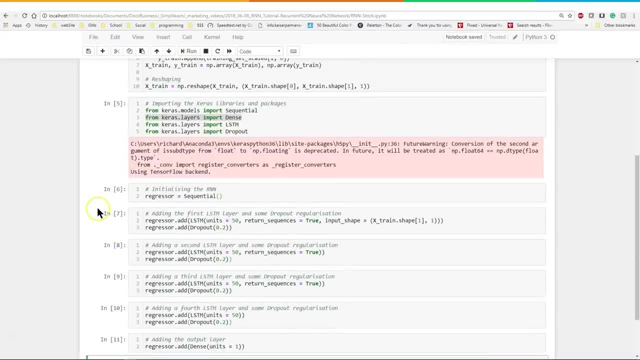 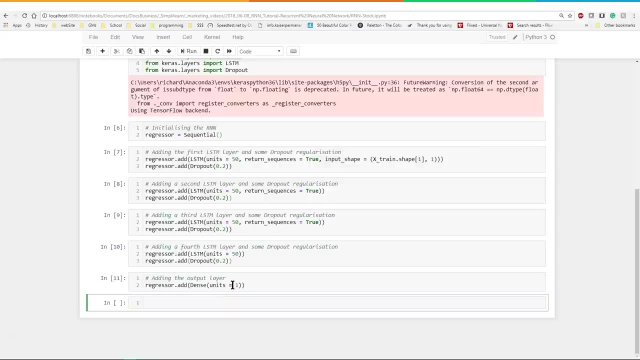 We've reshaped that. We've come in and built our Keras. We've imported our different layers And we have in here- if you look, we have what? Five total layers Now. Keras is a little different than a lot of other systems. 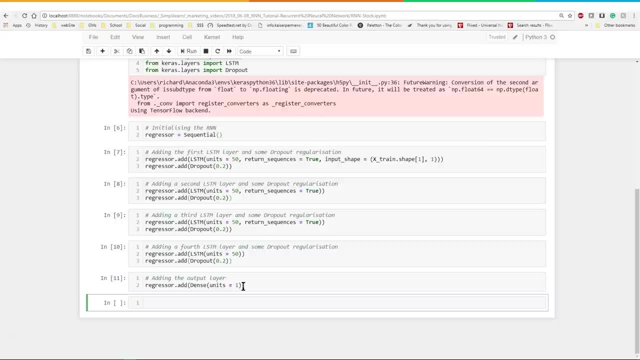 because a lot of other systems put this all in one line and do it automatic, But they don't give you the options of how those layers interface And they don't give you the options of how the data comes in. Keras is cutting edge for this reason. 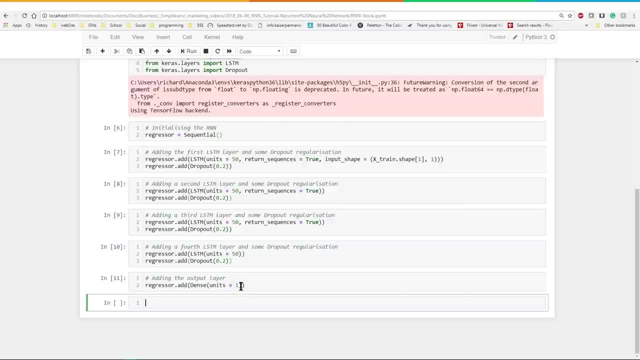 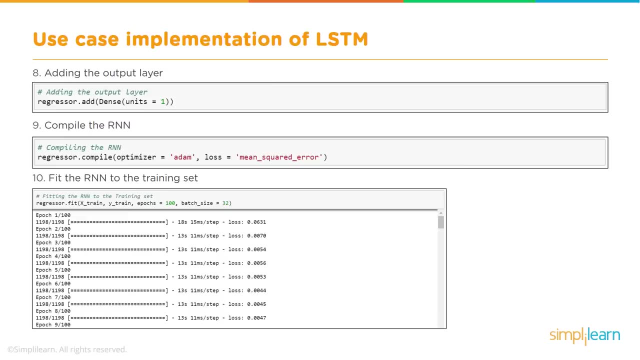 So, even though this is a lot of extra steps in building the model, this has a huge impact on the output and what we can do with these new models from Keras. So we brought in our dense. We have our full model put together. 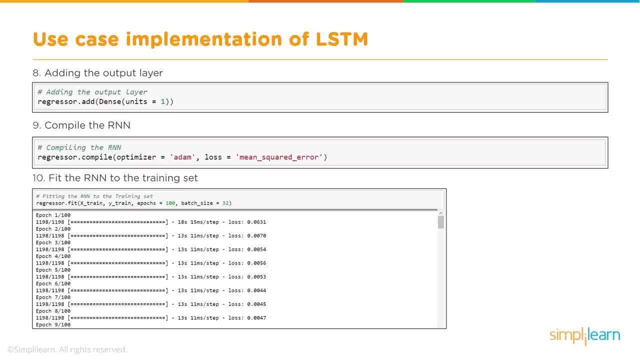 And we're going to use our regression regressor, So we need to go ahead and compile it, And then we're going to go ahead and fit the data, We're going to compile the pieces so they all come together And then we're going to run our training data on there. 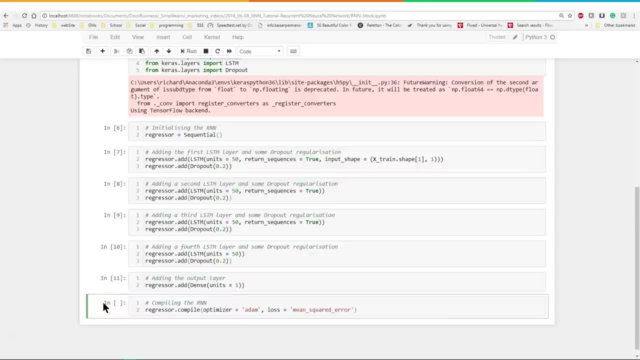 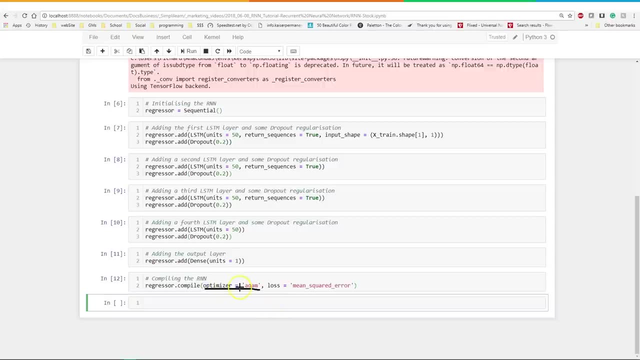 and actually create our regressor. so it's ready to be used. So let's go ahead and compile that And I can go ahead and run that. And if you've been looking at any of our other tutorials on neural networks, you'll see we're going to use the optimizer Atom. 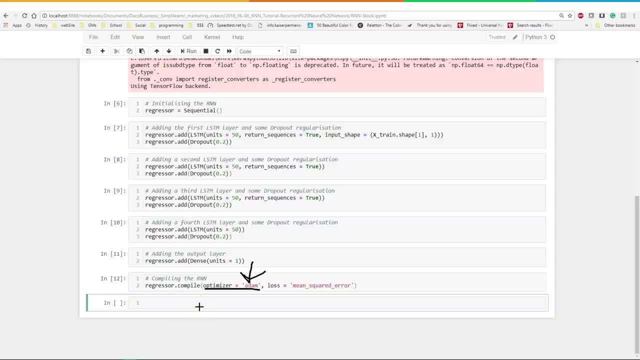 Atom is optimized for big data. There's a couple other optimizers out there beyond the scope of this tutorial, But certainly atom will work pretty good for this. And loss equals mean squared value. So when we're training it, this is what we want to base the loss on. 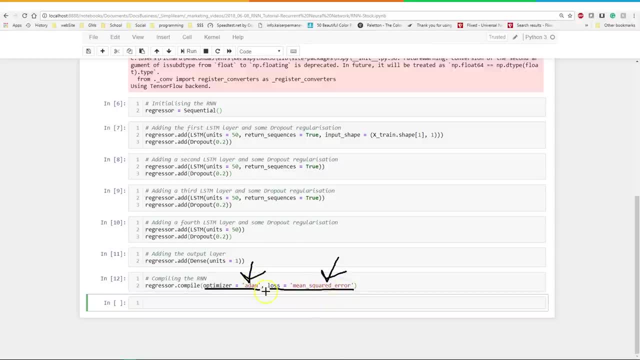 How bad is our error? Well, we're going to use the mean squared value for our error and the atom optimizer for its differential equations. You don't have to know the math behind them, but certainly it helps to know what they're doing and where they fit into the bigger models. 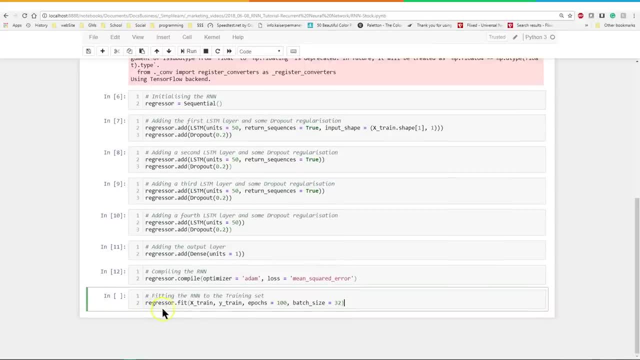 And then, finally, we're going to do our fit, fitting the RNN to the training set. We have the regressorfit, X train, Y train, epics and batch size. So we know where this is. This is our data coming in for the X train. 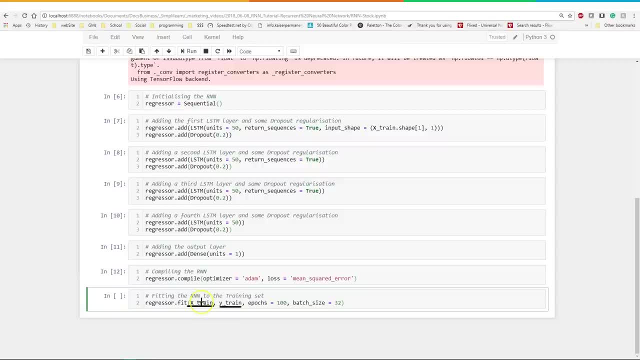 Our Y train is the answer we're looking for of our data. our sequential input, Epics, is how many times we're going to go over the whole data set. We created a whole data set of X train, So this is each of those rows which includes a time sequence of 60.. 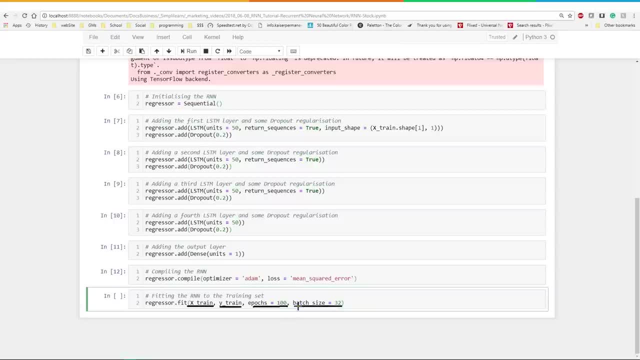 And batch size. another one of those things where Keras really shines is if you were pulling this, say, from a large file instead of trying to load it all into RAM. it can now pick smaller batches up And load those indirectly. 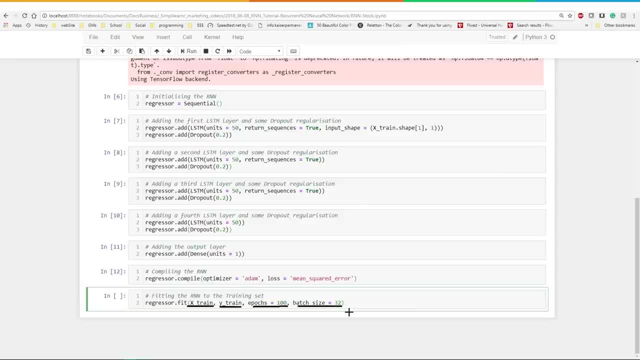 We're not worried about pulling them off a file today because this isn't big enough to cause the computer too much of a problem to run, Not too straining on the resources. But as we run this, you can imagine what would happen if I was doing a lot more than just one column in one set of stock. 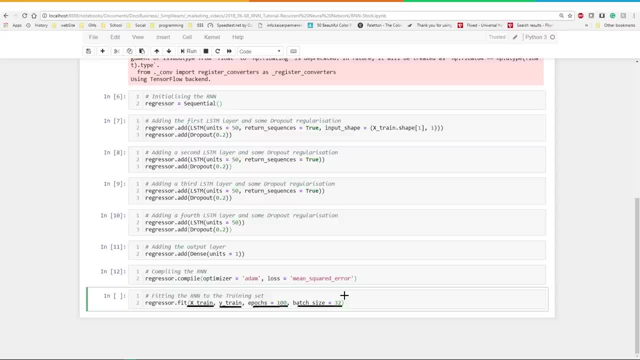 In this case, Google stock. Imagine if I was doing this across all the stocks and I had, instead of just the open, I had open, close, high, low. You can actually find yourself with about 13 different variables times 60,. 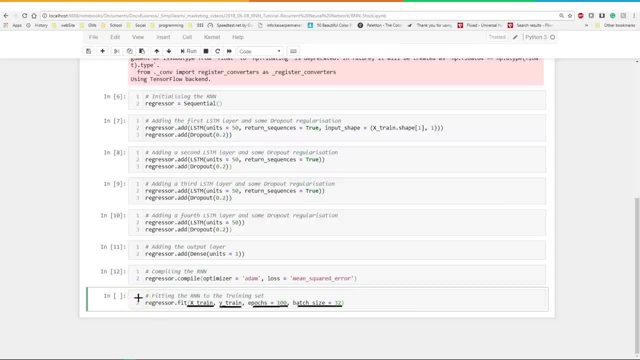 because there's a time sequence. Suddenly you find yourself with a gig of memory you're loading into your RAM which will just completely. you know, if it's just, if you're not on multiple computers or cluster, you're going to start running into resource problems. 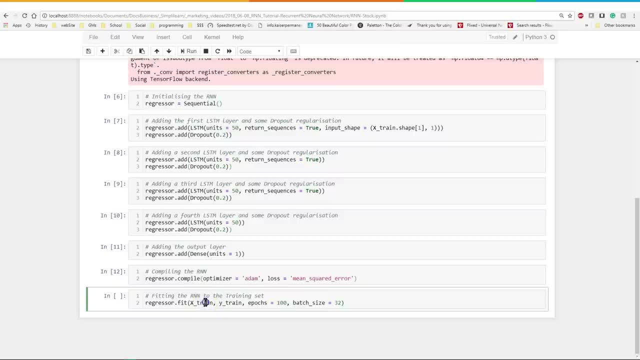 But for this we don't have to worry about that. So let's go ahead and run this- And this will actually take a little bit on my computer because it's an older laptop- And give it a second to kick in there. 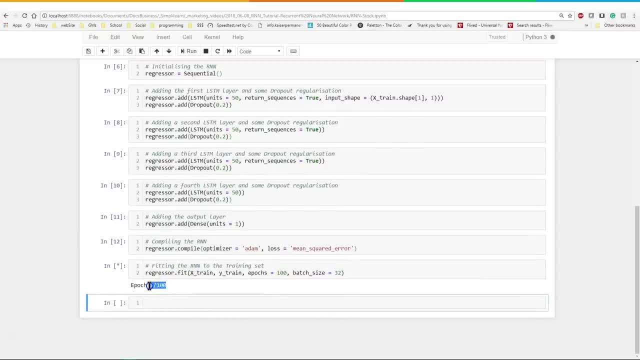 There we go, All right, So we have Epic. So this is going to tell me it's running the first run through all the data And, as it's going through, it's batching them in 32 pieces. So 32 pieces. 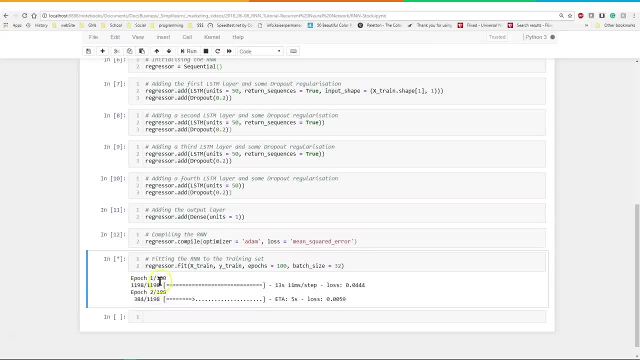 So 32 lines each time And there's 1,198.. I think I said 1,199 earlier, but it's 1,198.. I was off by one And each one of these is 13 seconds, So you can imagine this is roughly 20 to 30 minutes runtime on this computer. 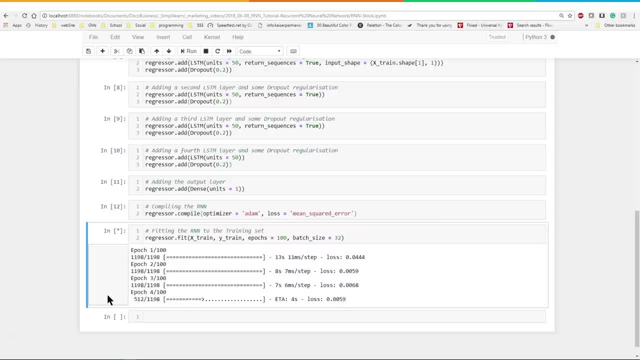 Like I said, it's an older laptop running at 0.9 gigahertz on a dual processor, And that's fine. What we'll do is I'll go ahead and stop, go get a drink of coffee and come back. 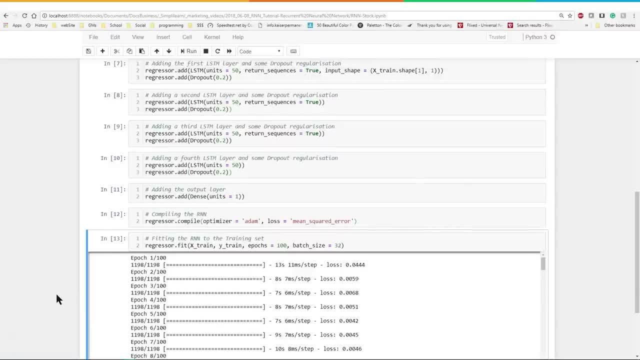 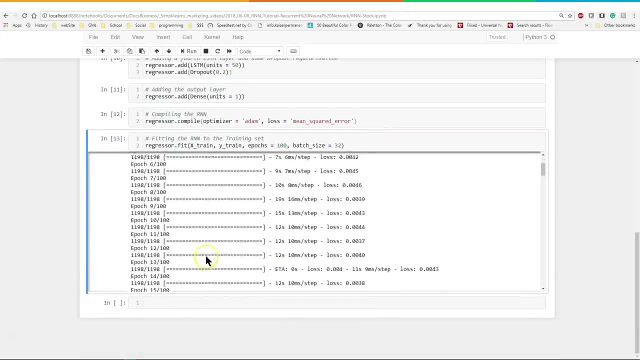 And let's see what happens at the end and where this takes us. And, like any good cooking show, I've kind of gotten my latte. Okay, I also had some other stuff running in the background, So you'll see these numbers jumped up to like 19 seconds, 15 seconds. 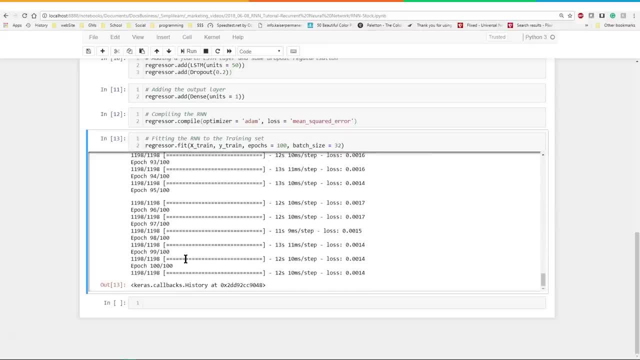 But you can scroll through and you can see we've run it through 100 steps or 100 Epics. So the question is: what does all this mean? One of the first things you'll notice is that our loss is over here. 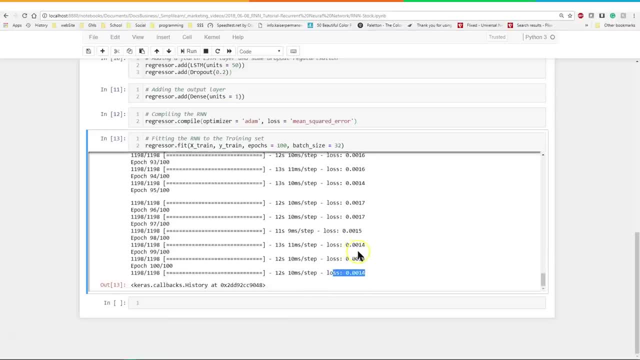 It kind of stopped at 0.0014, but you can see it kind of goes down until we hit about 0.014 three times in a row. So we guessed our Epic pretty close, since our loss has remained the same on there. 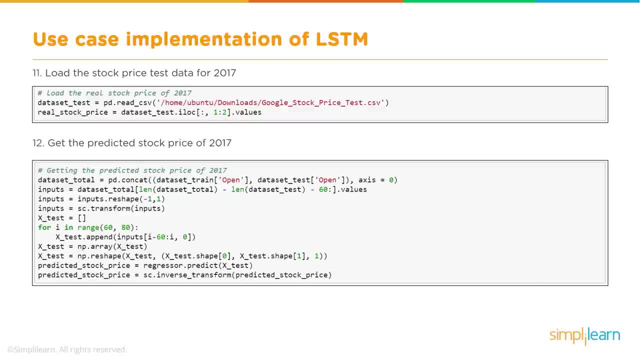 So, to find out what we're looking at, we're going to go ahead and load up our test Data, the test data that we didn't process yet and a real stock price data set test I location. This is the same thing we did when we prepped the data in the first place. 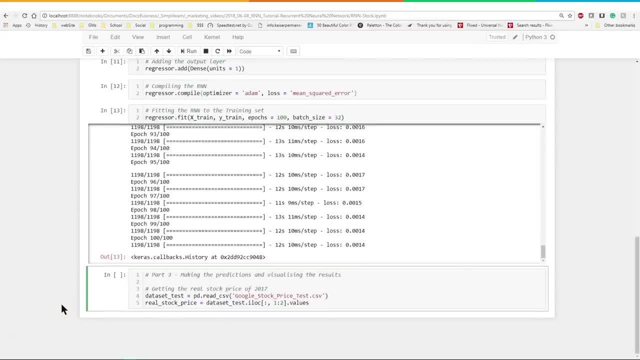 So let's go ahead and go through this code and we can see we've labeled it. part three, making the predictions and visualizing the results. So the first thing we need to do is go ahead and read the data in from our test CSV. 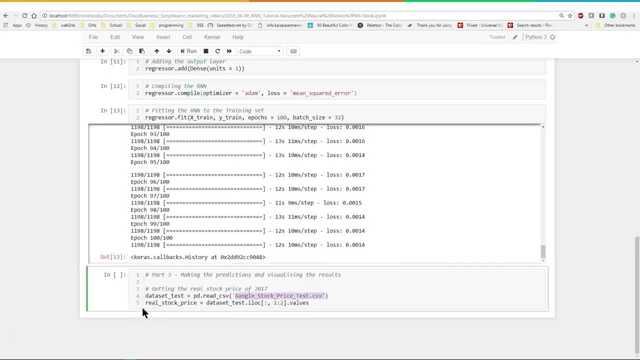 And you see I've changed the path on it for my computer And then we'll call it the real stock price And again we're doing just the one column here And the values from I location. So it's all the rows and just the values from these, that one location. 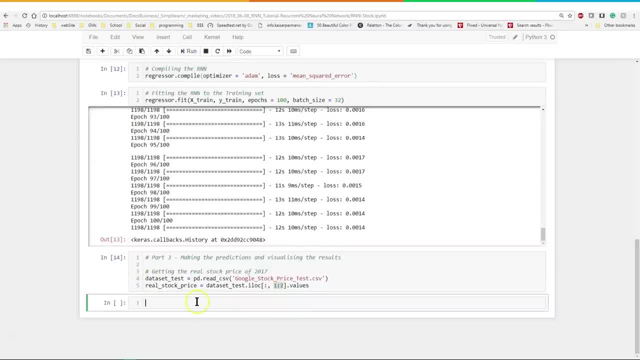 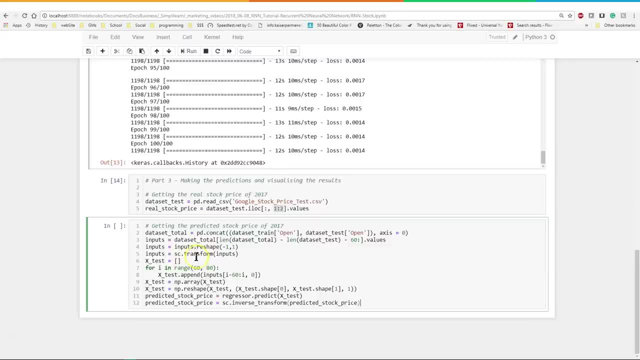 That's the open stock open. Let's go ahead and run that, So that's loaded in there, And then let's go ahead and create. We have our inputs, We're going to create inputs here, And this should all look familiar because this is the same thing we did before. 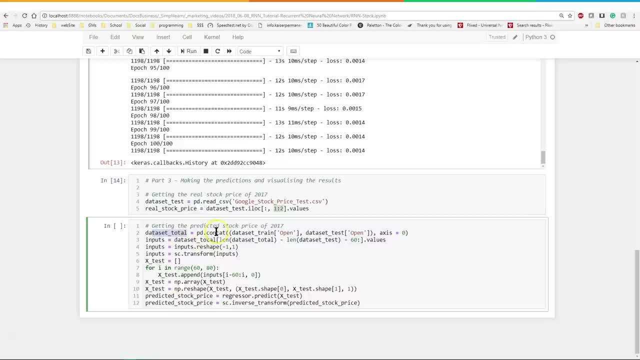 We're going to take our data set total. We're going to do a little pandas can cap from the data set train. Now, remember, the end of the data set train is part of the data going in And let's just visualize that. 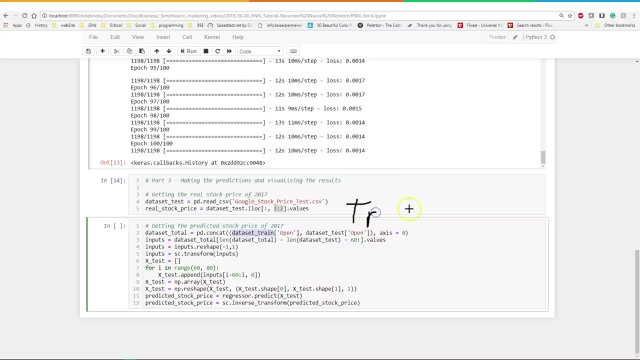 Just a little bit. Here's our train data. Let me just put TR for train. and it went up to this value here, But each one of these values generated a bunch of columns, So it was 60 across and this value here equals this one and this value here equals. 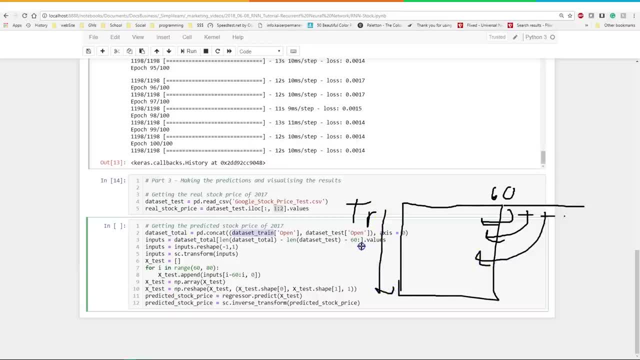 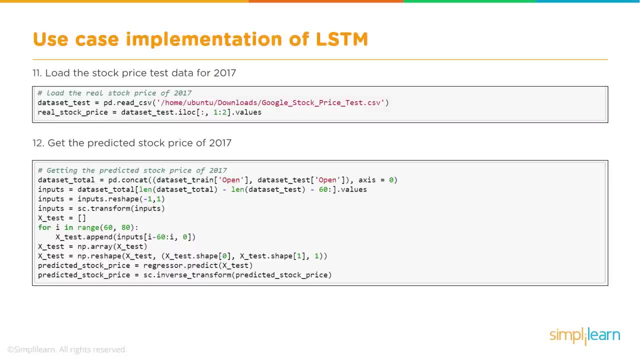 this one, and this value here equals this one, And so we need these top 60 to go into our new data. So, to find out we're looking at, we're going to go ahead and load up our test data- the test data that we didn't process yet, and a real stock price. 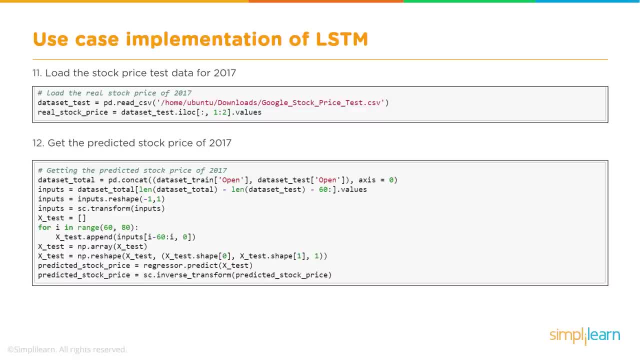 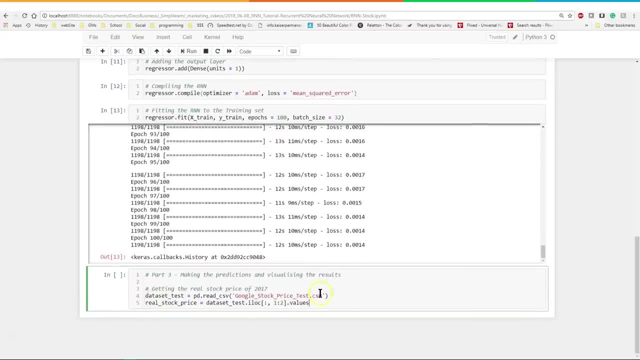 Data set test I location. This is the same thing we did when we prepped the data in the first place. So let's go ahead and go through this code And we can see. we've labeled it. part three: making the predictions and visualizing the results. 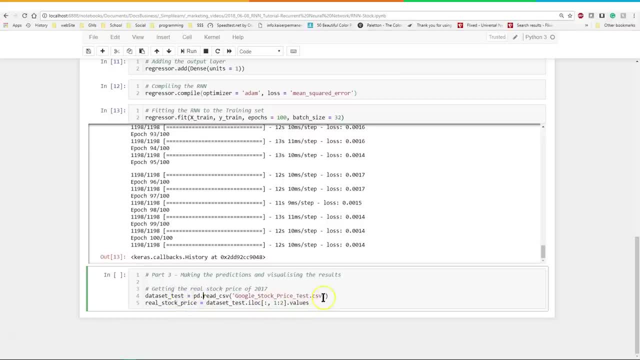 So the first thing we need to do is go ahead and read the data in from our test CSV- And you see, I've changed the path on it for my computer- And then we'll call it the real stock price, And again we're doing just the one column here and the values from I location. 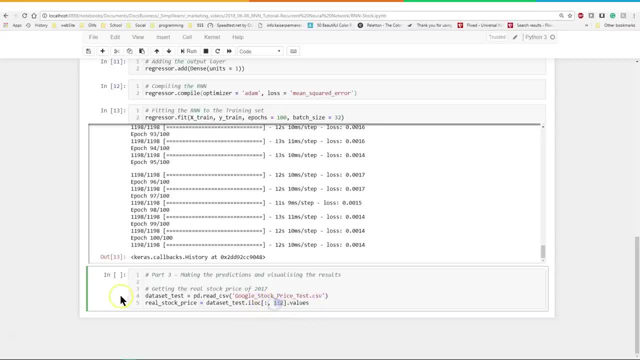 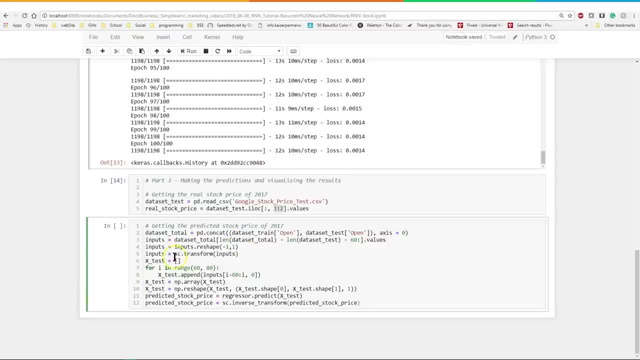 So it's all the rows, Just the values, The values from that one location. That's the open stock open. Let's go ahead and run that, So that's loaded in there, And then let's go ahead and create. We have our inputs. 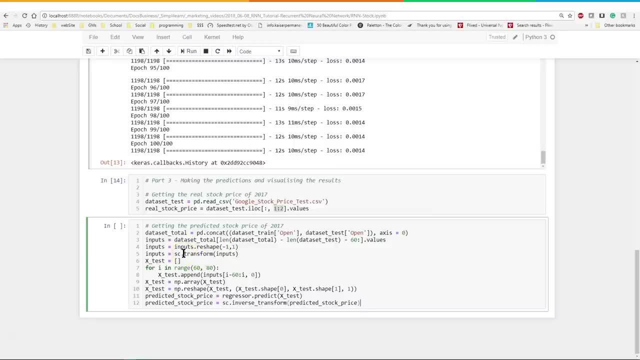 We're going to create inputs here- And this should all look familiar because this is the same thing we did before. We're going to take our data set total. We're going to do a little pandas concat from the data set train. Now, remember, the end of the data set train is part of the data going in. 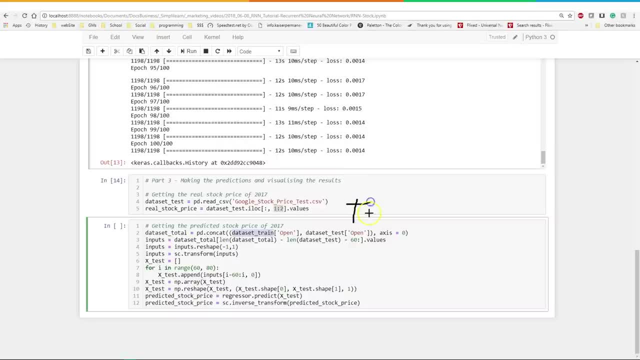 And let's just visualize that just a little bit. Here's our train data. Let me just put TR for train And it went up to this value here, But each one of these values generated a bunch of columns, So it was 60 across. 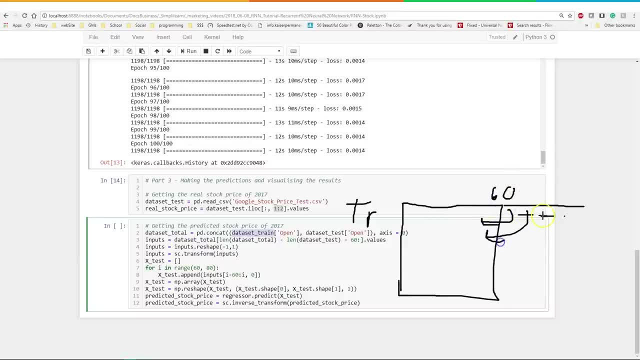 And this value here equals this one, And this value here equals this one, And this value here equals this one, And so we need these top 60 to go into our new data, because that's part of the next data, Or it's actually the top 59.. 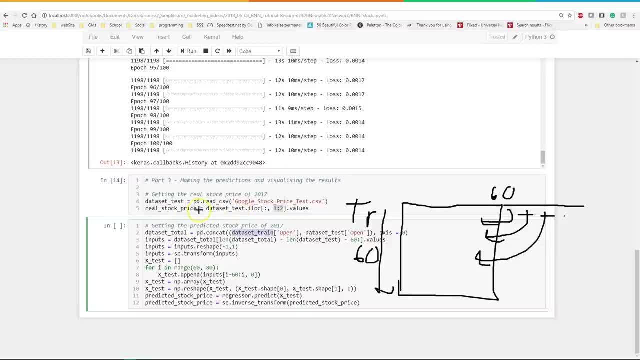 So that's what this first setup is over here is: we're going in, We're doing the real stock price And we're going to just take the data set test And we're going to load that in And then the real stock price is our data test test location. 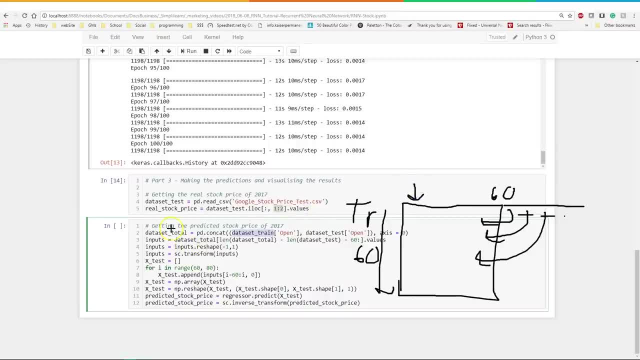 So we're just looking at that: first column, the open price, And then our data set total. We're going to take pandas and we're going to concat And we're going to take our data set train for the open and our data set test open. 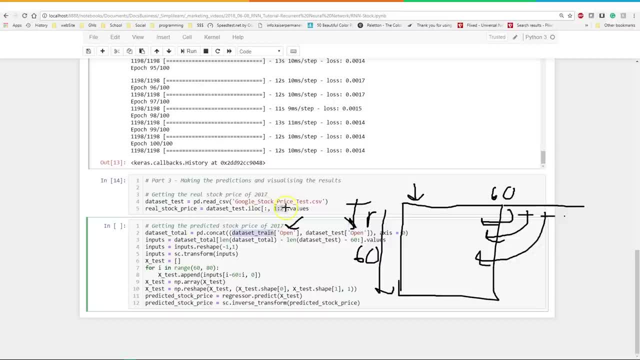 And this is one way you can reference these columns. We've referenced them a couple of different ways. We've referenced them up here with the one two, But we know it's labeled as a panda. set is open, So pandas is great that way. 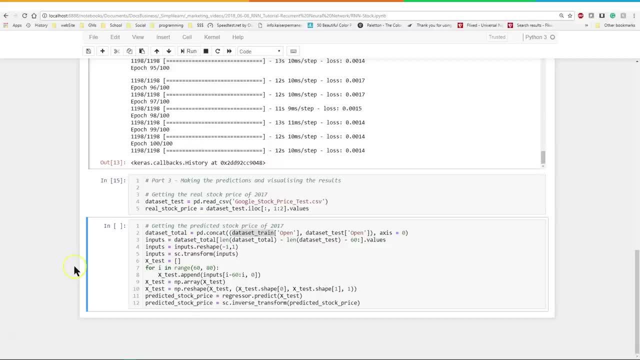 Lots of versatility there And we'll go ahead and go back up here and run this. There we go And you'll notice this is the same as what we did before. We have our open data set. We've pended our two different or concatenated our two data sets together. 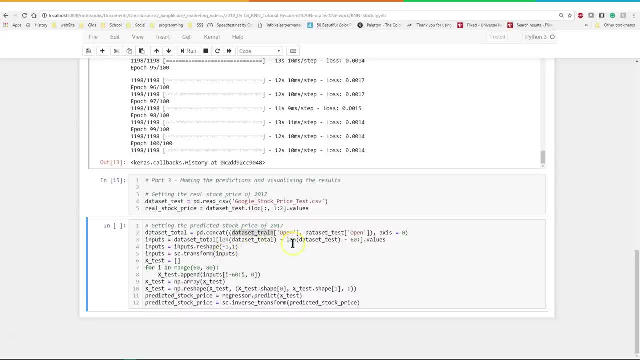 We have our inputs: equals: data set, total length. data set total minus length of data set, minus test, minus 60 values. So we're going to run this over all of them And you'll see why this works, because normally when you're running your test, 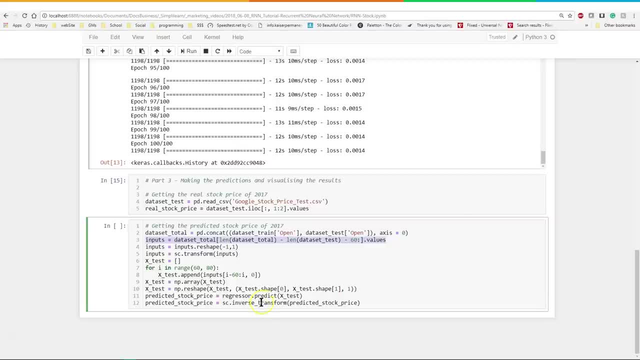 set versus your training set. you run them completely separate. But when we graph this, you'll see that we're just going to be looking at the part that we didn't train it with to see how well it graphs, And we have our inputs, equals inputs, dot, reshapes or reshaping, like we did before. 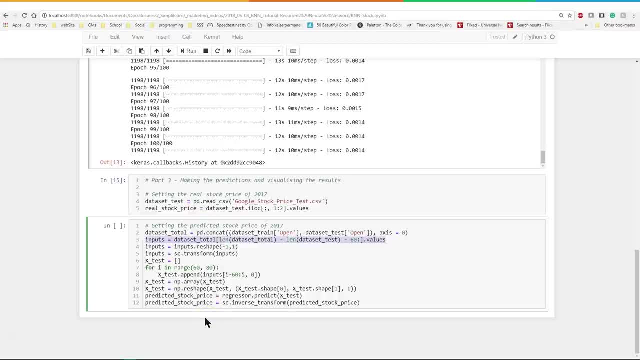 We're transforming our inputs. So if you remember, from the transform between zero and one, And finally, we're going to go ahead and take our X test and we're going to create that X test and for I, in range 60 to 80.. 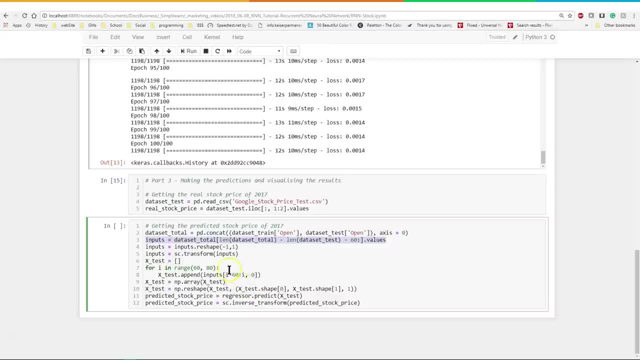 So here's our X test And we're appending our inputs I to 60, which, remember, is zero to 59, and I comma zero on the other side. So it's just the first column which is our open column, And once again we take our X test. 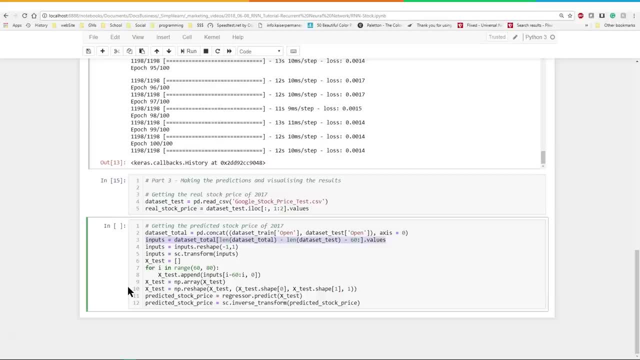 We convert it to a numpy array, We do the same reshape we did before, And then we get down to the final two lines, And here we have something new, right here on these last two lines. Let me just highlight those or mark them. 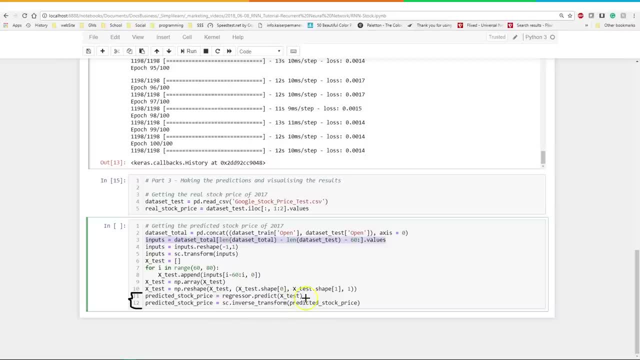 Predicted stock price equals regressor dot predicts X test. So we're predicting all the stock, including both the training and the testing model here. And then we want to take this prediction and we want to inverse the transform. So remember we put it between zero and one. 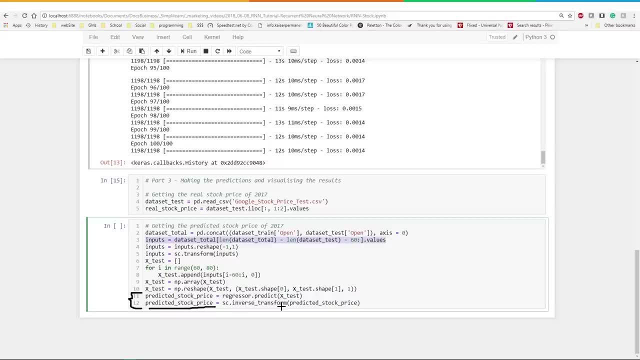 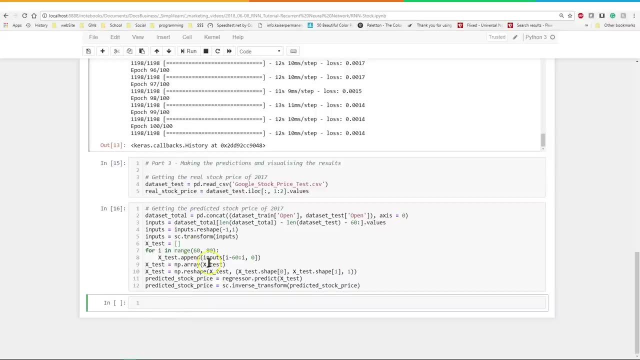 Well, that's not going to mean very much to me to look at a float number between zero and one. I want the dollar amounts, I want to know what the cash value is, And we'll go ahead and run this and you'll see, it runs much quicker than the training. 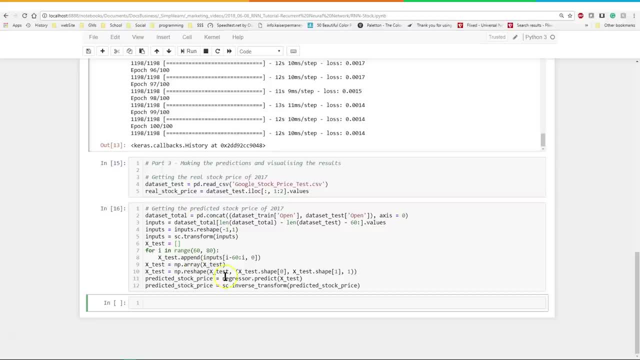 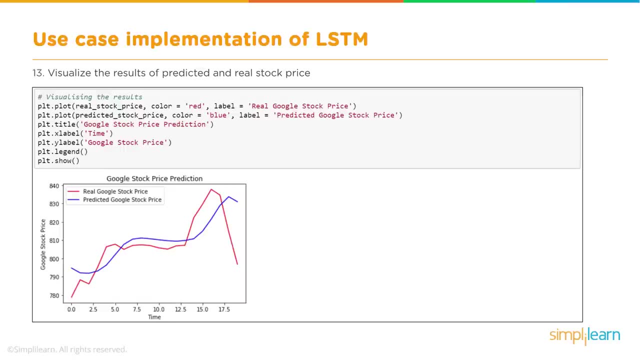 That's what's so wonderful about these neural networks: Once you put them together, it takes just a second to run the same neural network. that took us what a half hour to train, Add and plot the data. We're going to plot what we think it's going to be and we're going to plot it. 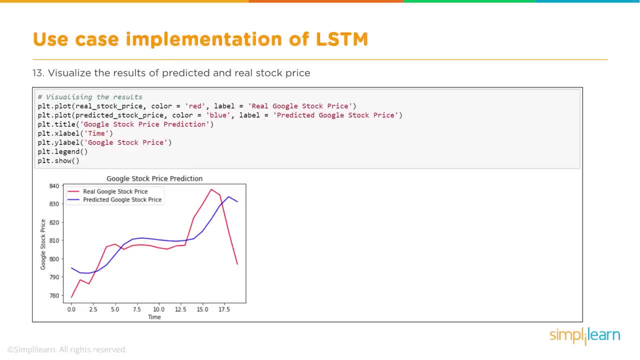 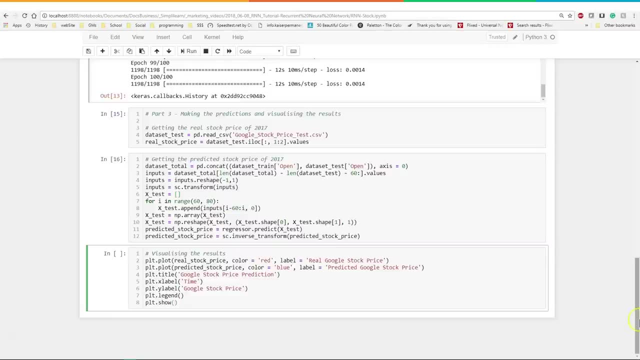 against the real data what the Google stock actually did. So let's go ahead and take a look at that in code and let's pull this code up. So we have our PLT. That's our, if you remember from the very beginning. let me just go back up to 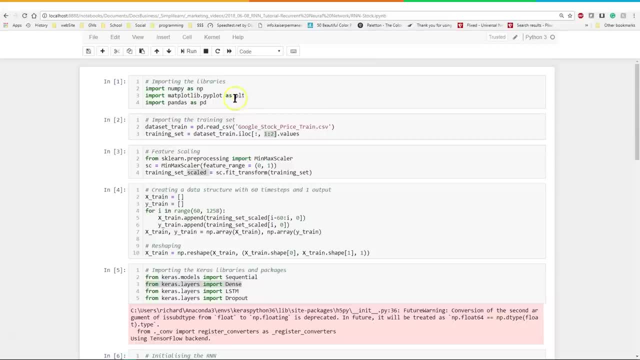 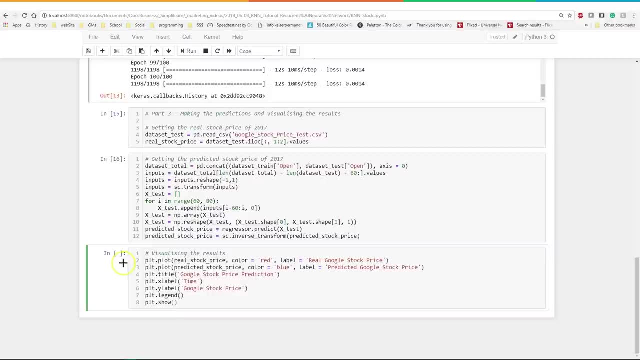 the top we have our matplotlibrarypyplot as PLT. That's where that comes in. When we come down here, we're going to plot. Let me get my drawing thing out again. We're going to go ahead and PLT is basically kind of like an object. 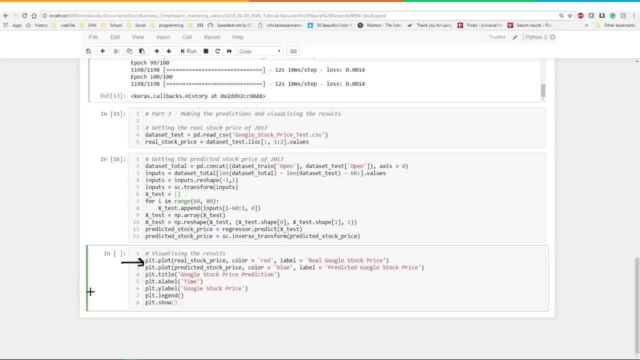 It's one of the things that always threw me when I'm doing graphs in Python, because I always think you have to create an object and then it loads that class in there. Well, in this case, PLT is like a canvas: you're putting stuff on. 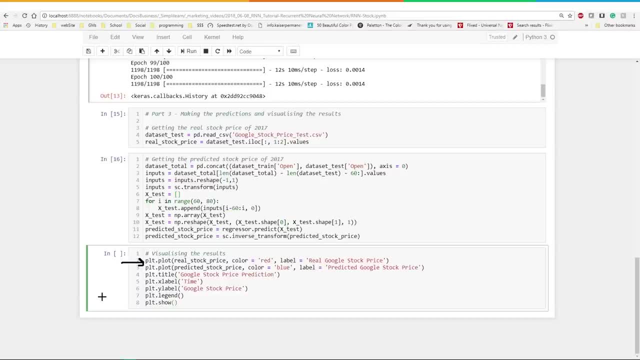 So if you've done HTML5, you'll have the canvas object. This is the canvas, So we're going to plot the real stock price- That's what it actually is- And we're going to give that color red, So it's going to be a bright red. 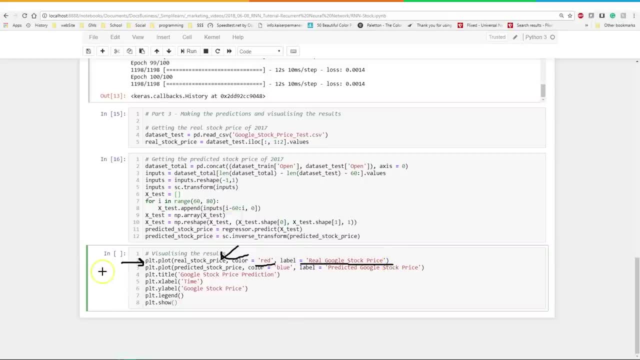 We're going to label it real Google stock price And then we're going to do our predicted stock. We're going to do it in blue and it's going to be labeled predicted. And we'll give it a title, because it's always nice to give a title to your graph. 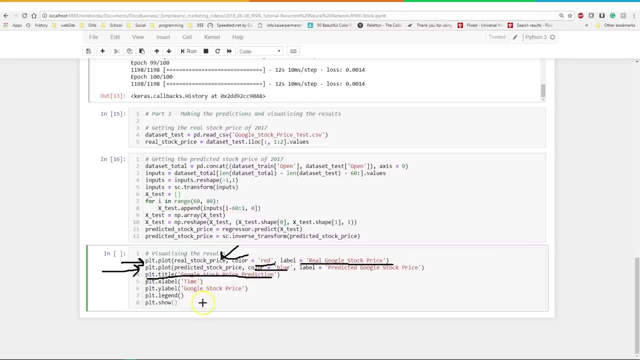 especially if you're going to present this to somebody, to your shareholders in the office, And the X label is going to be time, because it's a time series And we didn't actually put the actual date and times on here. but that's fine. 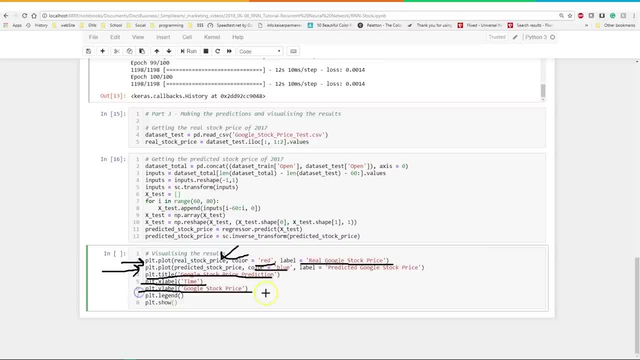 We just know they're incremented by time. And then, of course, the Y label is the actual stock price. PLTLegend tells us to build the legend on here so that the color red and real Google stock price show up on there. 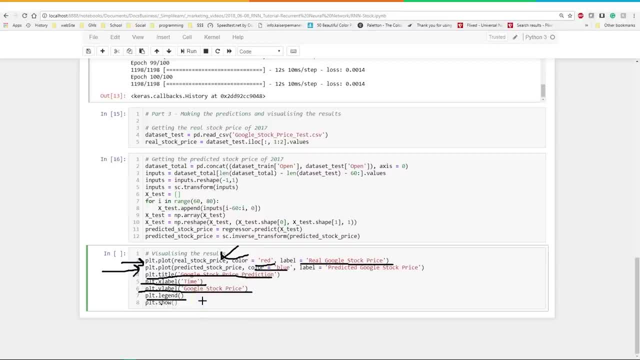 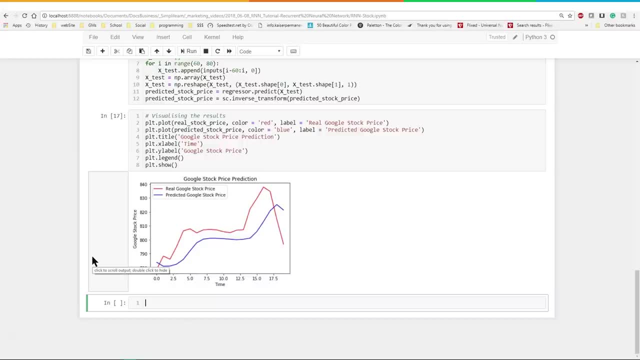 And then the plot shows us that actual graph. So let's go ahead and run this and see what that looks like. And you can see, here we have a nice graph. And let's talk just a little bit about this graph before we wrap it up. 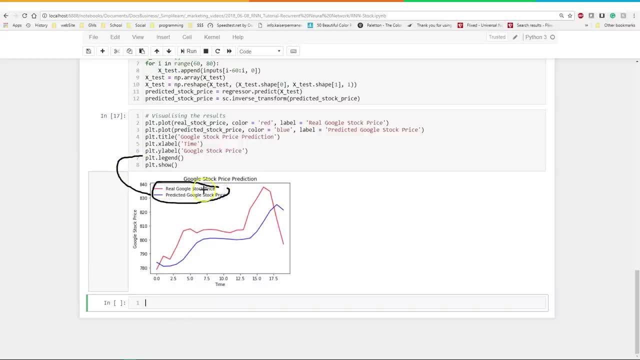 Here's our legend I was telling you about. That's why we have the legend to show the prices. We have our title and everything And you'll Notice on the bottom we have a time sequence. We didn't put the actual time in here. 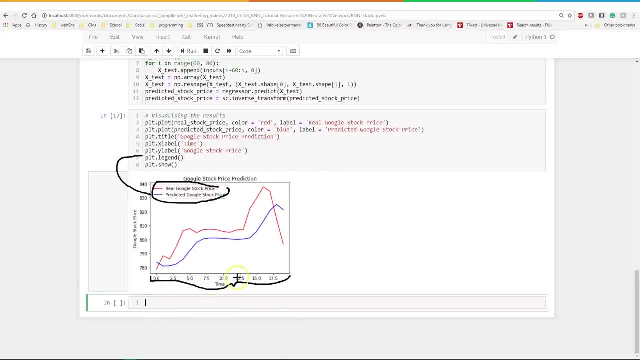 Now we could have. We could have gone ahead and plotted the X, since we know what the dates are, and plotted this to dates. But we also know that it's only the last piece of data that we're looking at. So, last piece of data which in somewhere, probably around here on the graph, 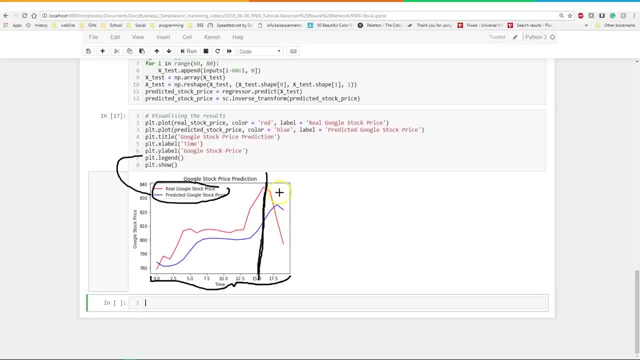 I think it's like about 20% of the data, probably less than that. We have the Google price and the Google price has this little up jump and then down, And you'll see that the actual Google, Instead of a turn down here, just didn't go up as high and didn't go down. 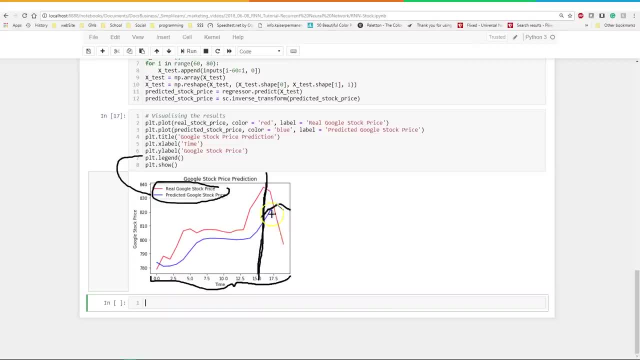 So our prediction has the same pattern, but the overall value is pretty far off as far as stock. But then again, we're only looking at one column, We're only looking at the open price, We're not looking at how many volumes were traded. 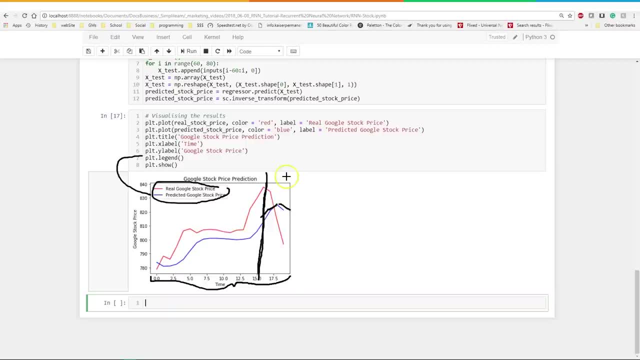 Like I was pointing out earlier, we talk about stock just right off the bat. There's six columns. There's open, high, low, close volume. Then there's whether I mean volume, shares, Then there's the adjusted Open, adjusted high, adjusted low, adjusted close. 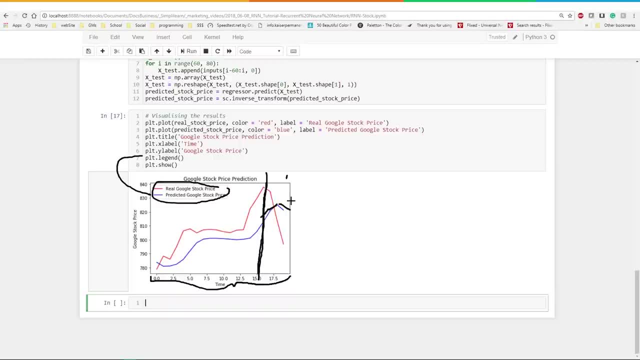 They have a special formula to predict exactly what it would really be worth, based on the value of the stock, And then from there there's all kinds of other stuff you can put in here. So we're only looking at one small aspect: the opening price of the stock. 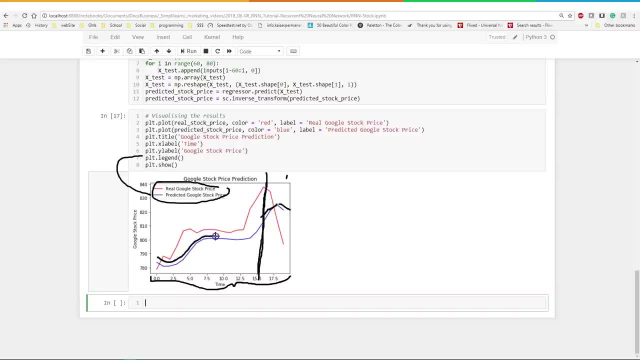 And as you can see here we did a pretty good job. This curve follows the curve pretty well. It has like a little jumps on it Bins. they don't quite match up. So this bin here does not quite match up with that bin there, but it's pretty darn close.